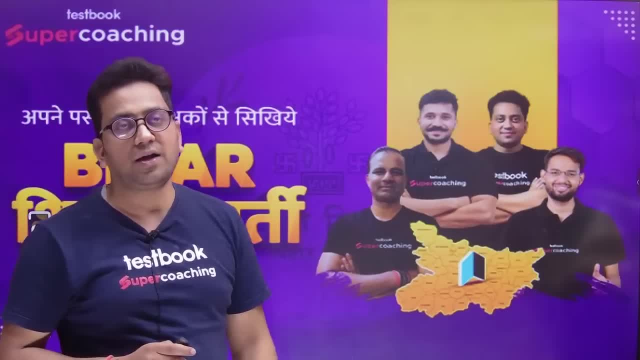 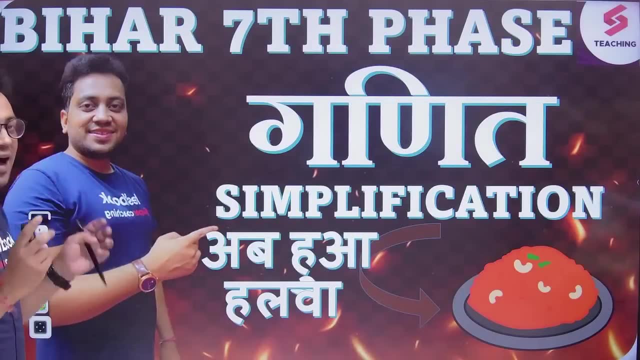 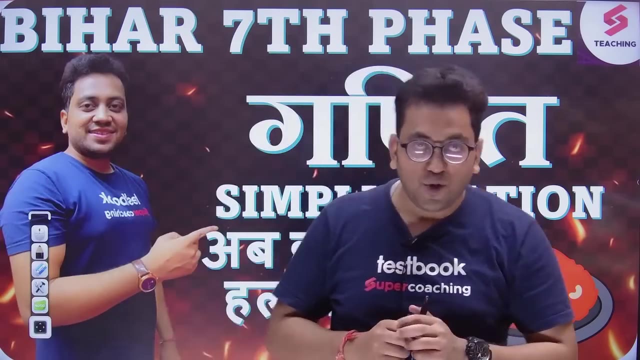 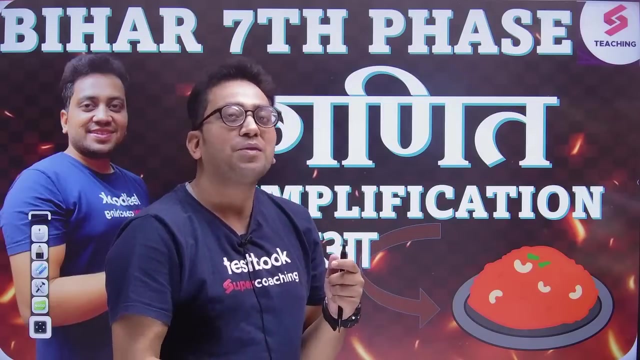 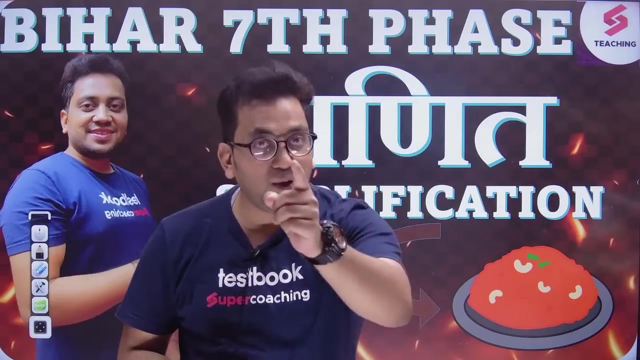 Thank you, Thank you, Thank you all, Thank you, Thank you, Thank you all, Thanków, Thank you all. You all have to get rid of your hunger. Are you all ready Say yes, sir, Hungry, hungry, hungry. 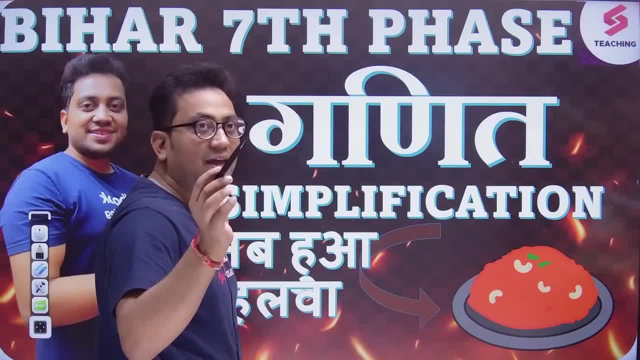 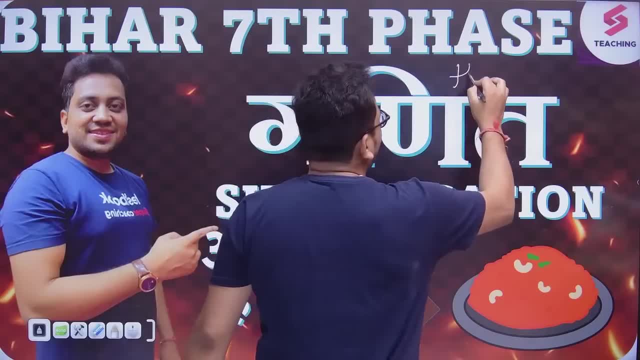 We will quickly write in the comment section, all of you together. What will you write? What will you write, Hungry, Right, What will you write, son, Hungry, Because we will get rid of your hunger. Why are you taking your tension? 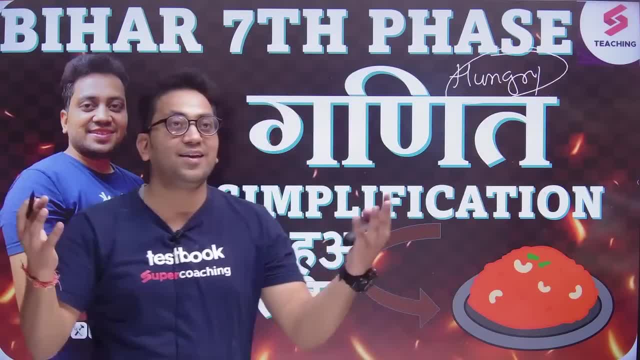 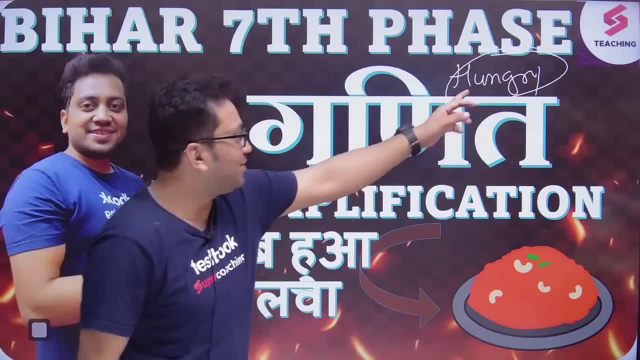 Quickly, All the children will write in the comment section once: Hungry. For whom, sir? Yes, For Garit, He is hungry. He has hunger inside him Right. Quickly write all the children once in the comment section: Are you hungry? 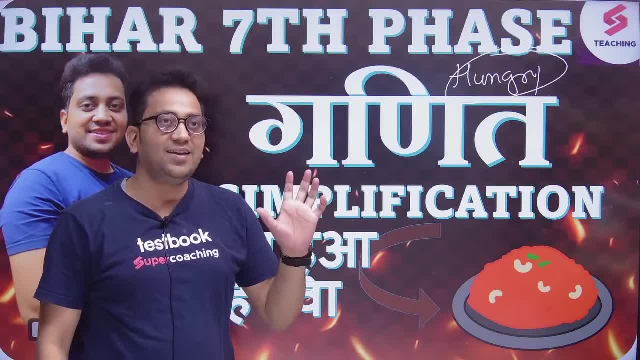 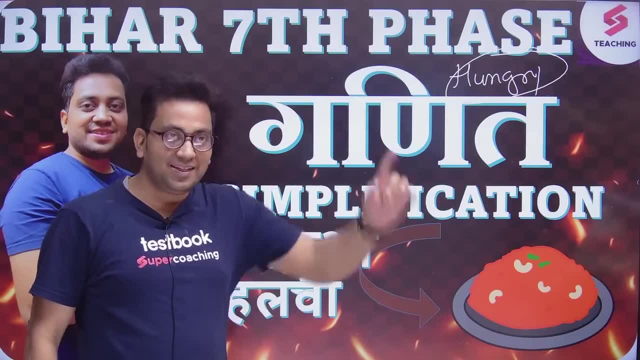 Are you ready to eat Garit's today's halwa? Ready? All of you Not now. You have to write now, Right, Write Hungry. H-U-N-G-R. Hungry. You all take English classes. 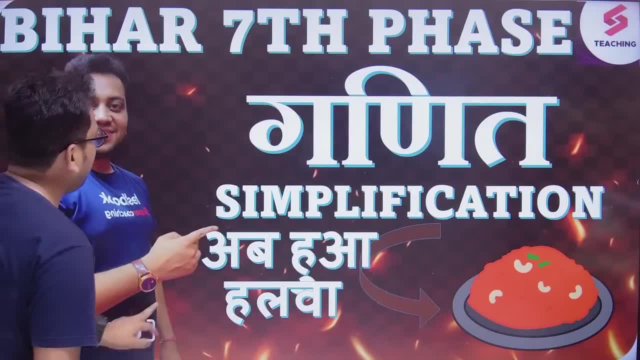 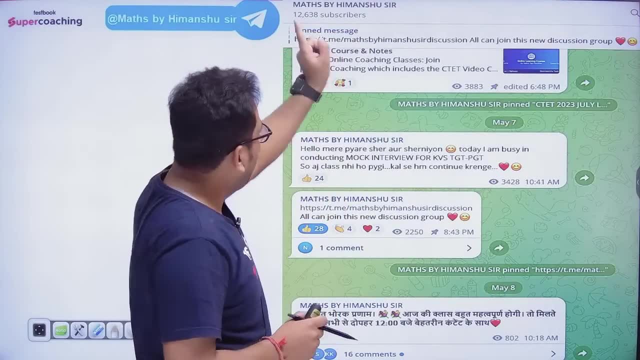 Hungry, Tell everyone: Yes, Very good, Come on, Let's start. Let's start. And the child who is not yet connected to this telegram channel? It is limited. They join Maths by Himanshu Sir is a telegram channel. 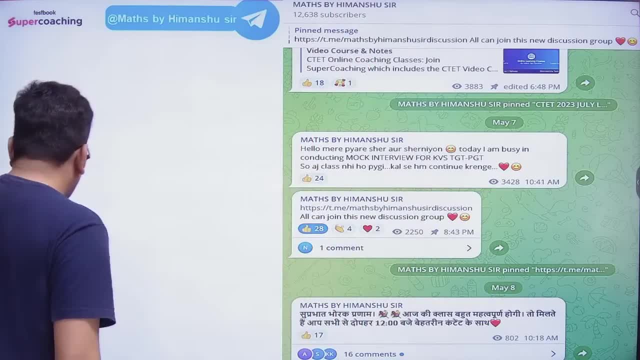 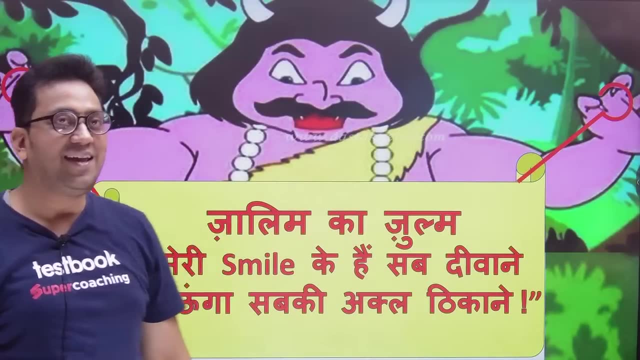 If any child is not yet connected, then join Right, Come on. So let's start. And we will start with the cruelty of the tyrant. See what the tyrant is saying. Did you see his smile? Two teeth are coming out of him. 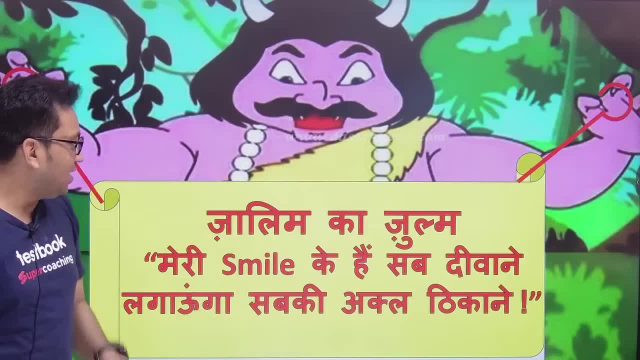 Right, Yes, He says the cruelty of the tyrant. So he says that everyone is crazy about my smile, But I will put everyone's brains. So, son, we are going to see the cruelty of the tyrant. How did you bring the cruelty? 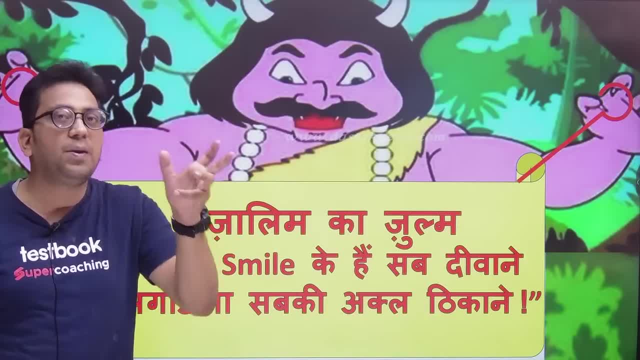 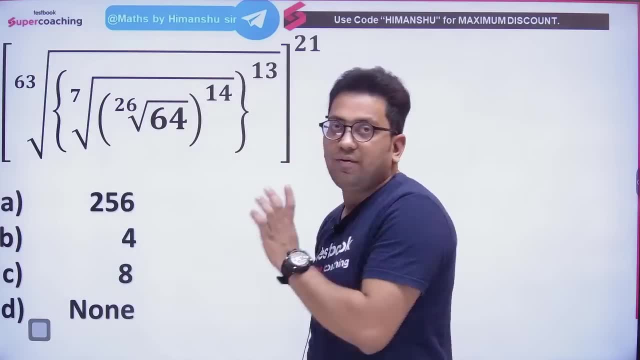 What kind of questions did you bring Which is very important for our BPSC Today? only on these questions We are going to see all the questions of simplification. So the first question of today's session. This was the first question in today's session. 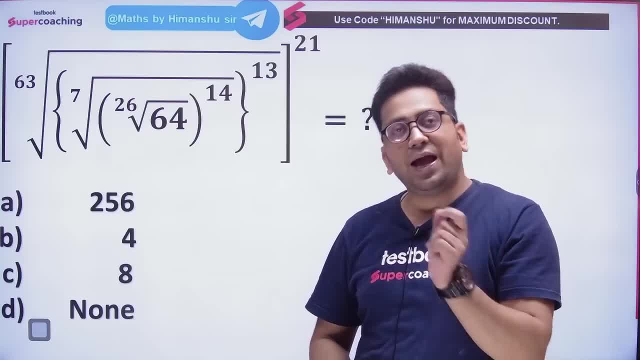 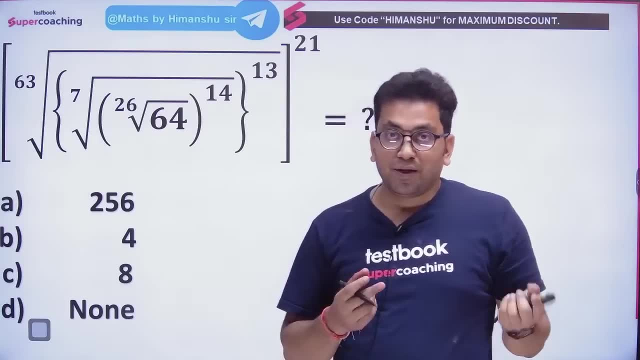 Tomorrow. the last session is also on our simplification. Today it is the second class of simplification. Okay, Look, this question came to you in this way. Now I said I have brought the teeth Like elephant teeth, Sir. they are on the side of eating and on the side of showing. 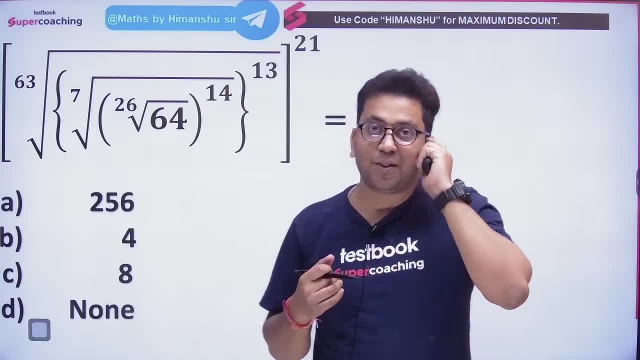 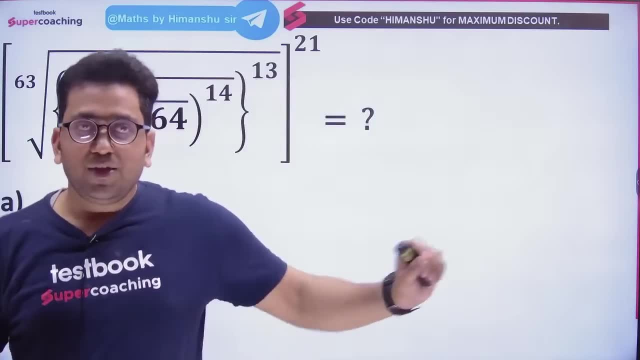 This is the same question. Now it seems to be visible, Sir. I don't know what this question is, But we will shine it. We will tell you how to shine it. So in today's session, we will not shine it. 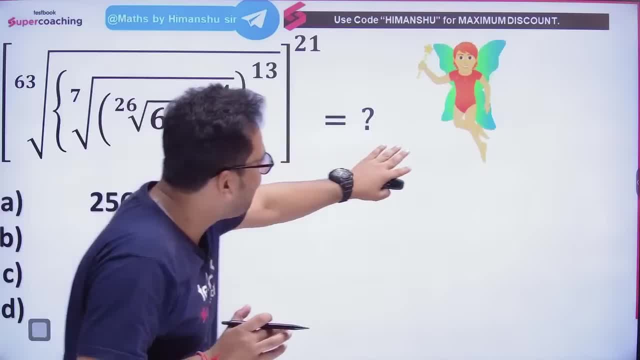 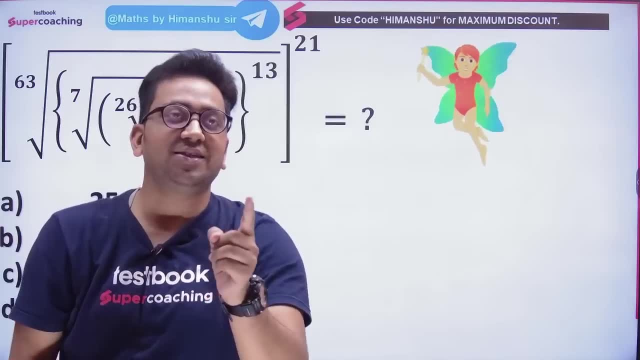 We will not shine it. To shine it, we have called it, brother, Papa's fairy. Papa's fairy is like Papa's fairy, So Papa's fairy will shine, son. Today. Papa's fairy will shine this question. Okay, Now see how it will shine. 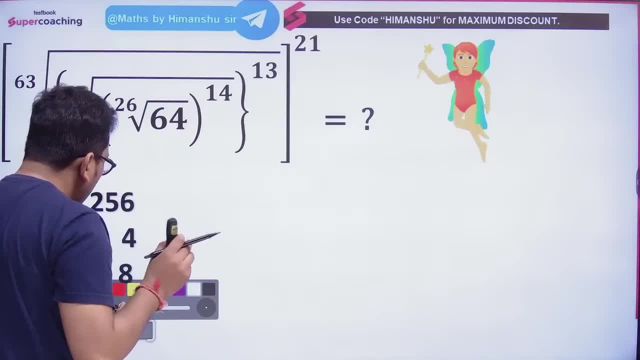 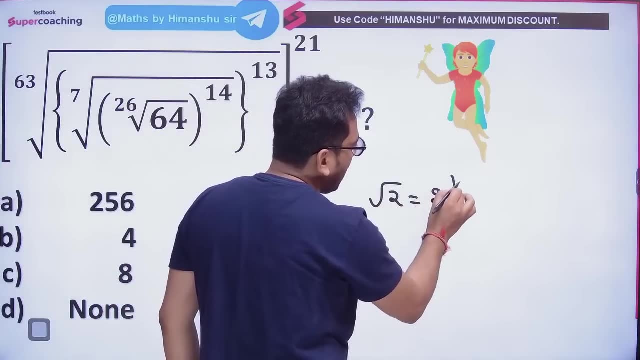 So Papa's fairy says this: Look, there is a simple logic, There is a concept. And Papa's fairy shines with the concept. He says this: Tell me, how can you write root 2?? So you will say: divide 1 by 2.. 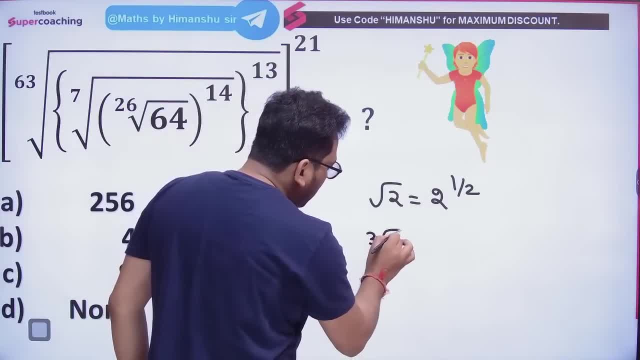 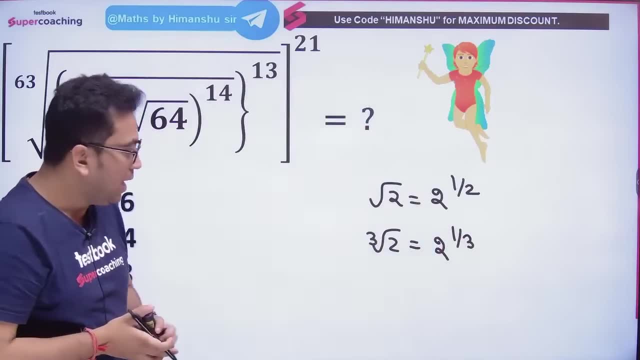 Say yes or no. He says, Sir, if there were two cube roots? That is, how would it be written if there were 2 root roots? So you say: divide 1 by 2 by 3. It means that the number put in the number with the root here goes to the part in the root. 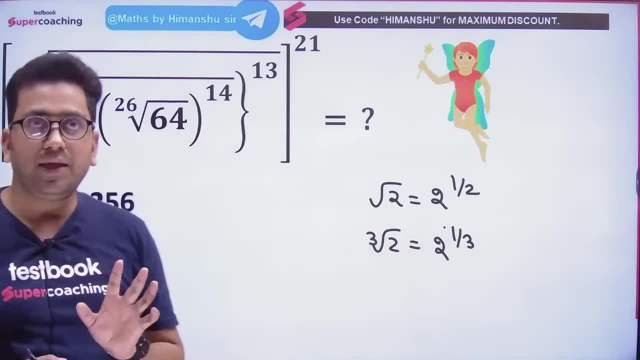 Or it goes down, It goes in the divide. Do you understand this thing? Do you understand this concept? Yes, it comes. Okay, sir, If I say the power of 2, will anyone interfere in it? No, sir. 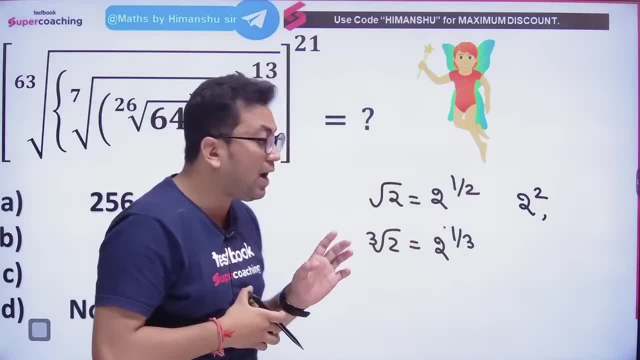 There will be no interference in it. That is what is in the root will remain in the root, But the one with the root, The one with the root, will come down in the root. It will come in the divide, As you can see: 1 divided by 3.. 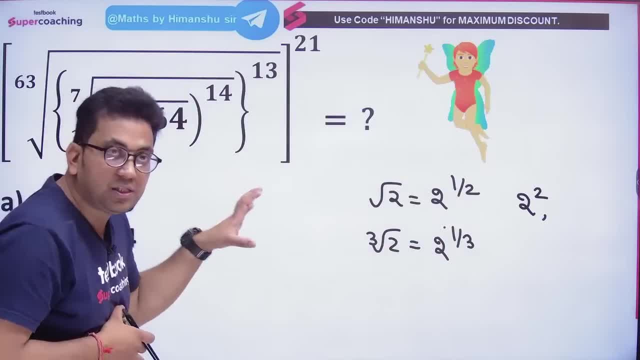 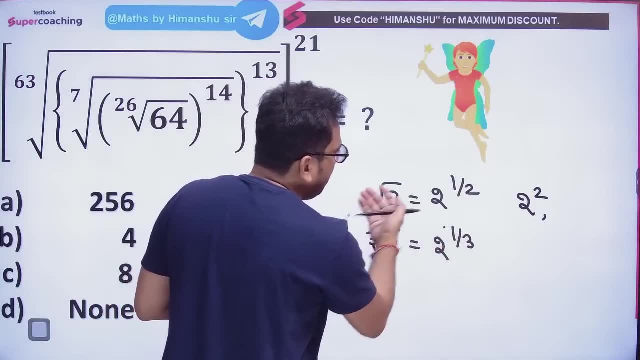 As you can see, 1 divided by 2.. So with the same concept we will shine this question. So Papa's fairy is saying that the way you put the one with the root in the divide, In the same way you see here that what is attached to the root here. 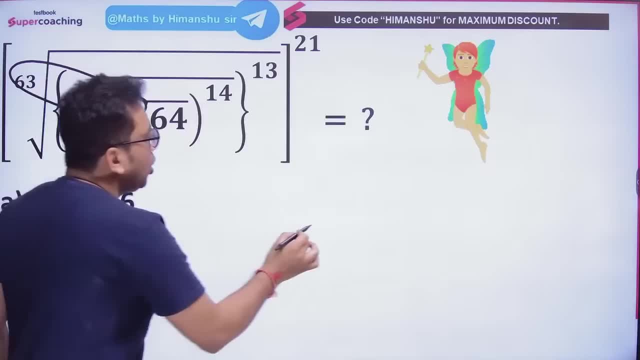 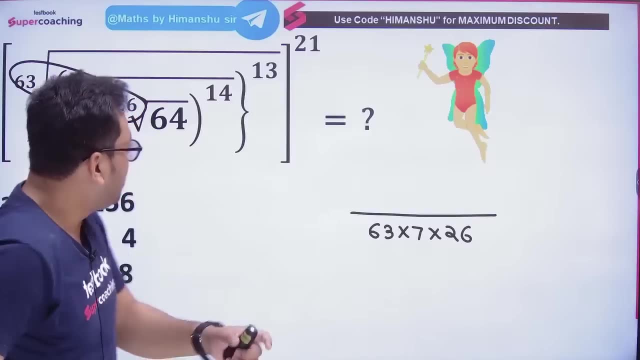 This is going on continuously: 63,, 7 and 26.. So he says, put it down: 63,, 7 and 26.. Put it down, And the one with the root put it on top of it: 14 times, 13 times 21.. 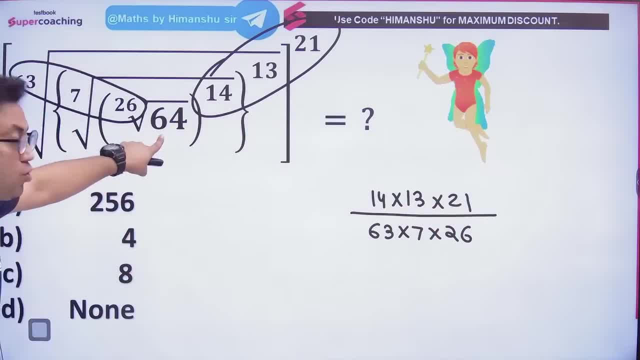 Do you understand what I am saying And whose root is this? This is 64.. Put 64 here. See this. Now you must be liking it, Isn't it Why? Because you put this one up and put this one down. 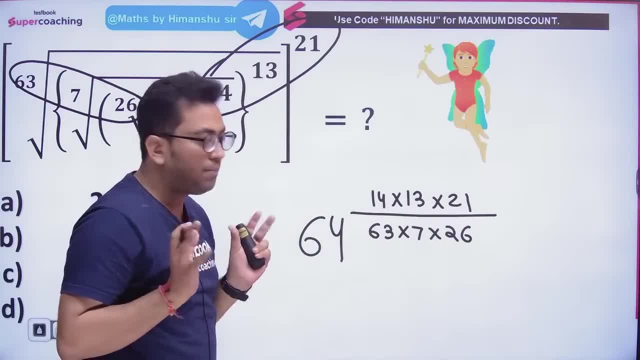 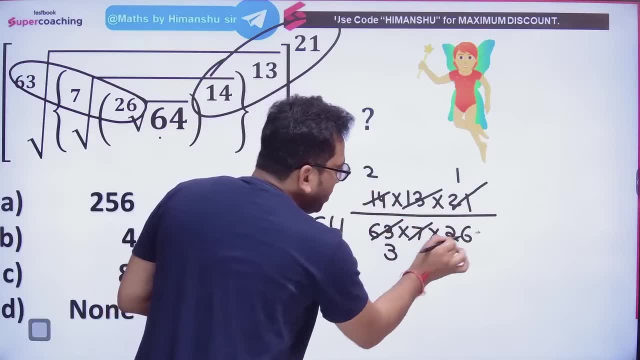 Now all of this has become the root of 64. Now I will solve this. It is very easy: 21 minus 21.. 21,, 33.. 21,, 33,, 63.. 7 times 14.. 13 times 26.. 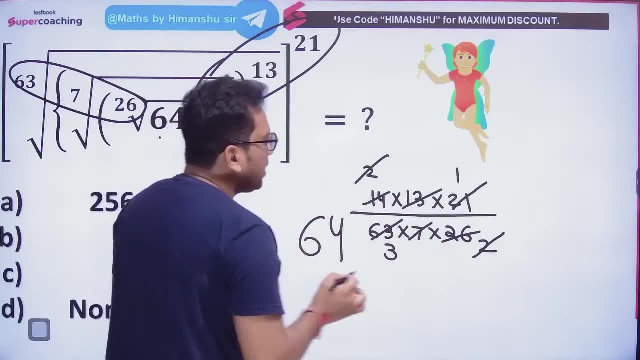 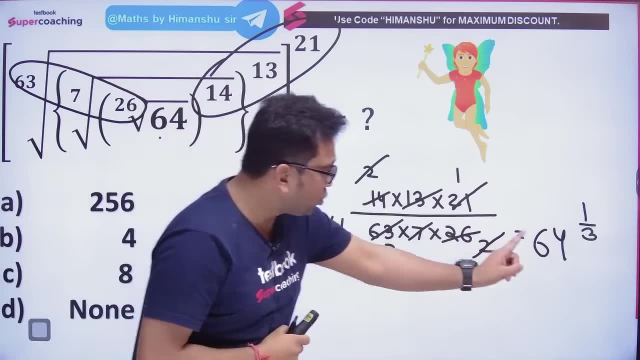 Say yes, Tell me 2 divided by 2.. We did it So 64.. How much is the root? It is 1 divided by 3.. Now you see that whose root is 64? This is 3.. 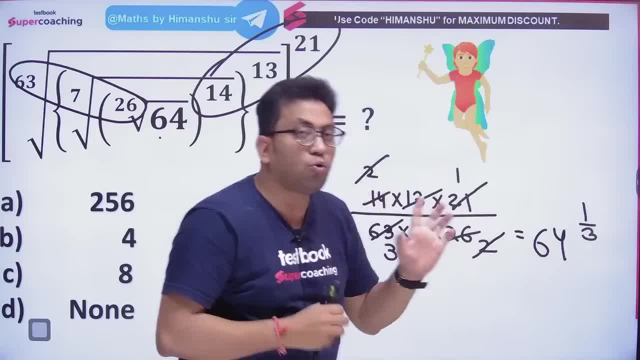 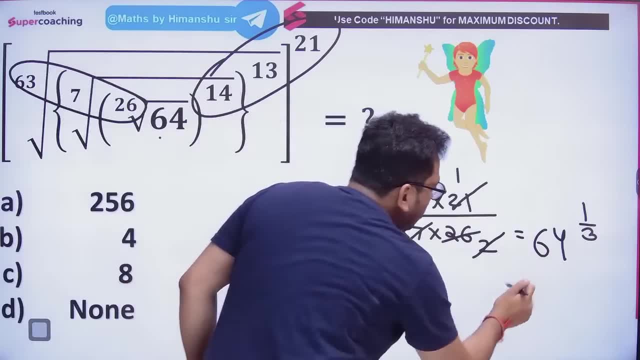 Only then it will be able to cut Which is below. this: 3 is cut only when you see whose root is 64. So it is 4.. 4, 4, 16, 64. You will say, sir, this is 4 plus 3, and outside there is 1 plus 3 plus 3, so 3 to 3 is cut. 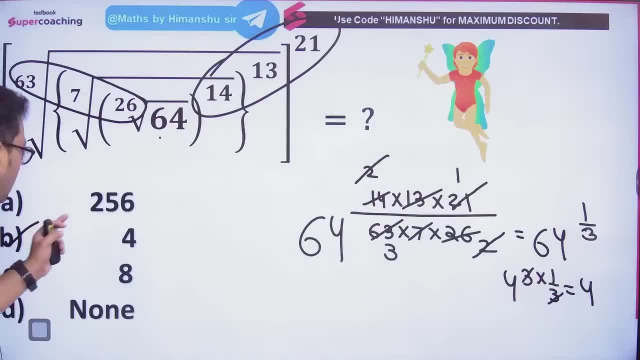 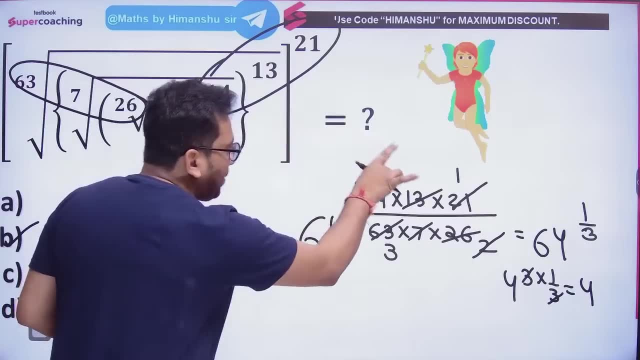 What is the answer? 4.. So 4 is our answer and option B will also be our answer. Tell me, did it shine? Did it shine or not? Did it shine? If every child understood, then if your father is able to shine, then you will also shine. 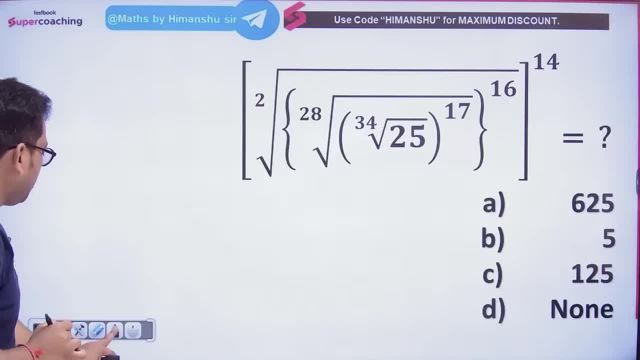 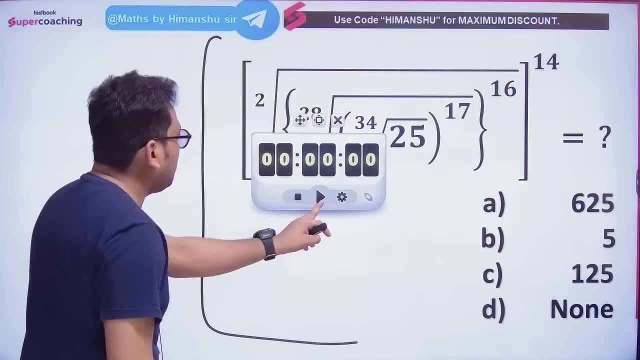 Is it not? Next question? Next question is coming in front of you. My every child will shine quickly, Answer quickly. Tell me what will be the answer. Let's set the timer Today. I have brought so many questions for you in this session. 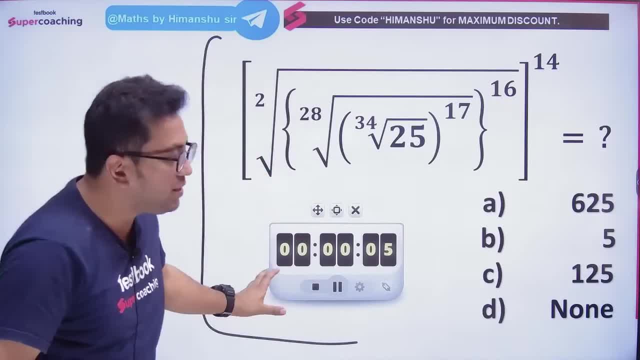 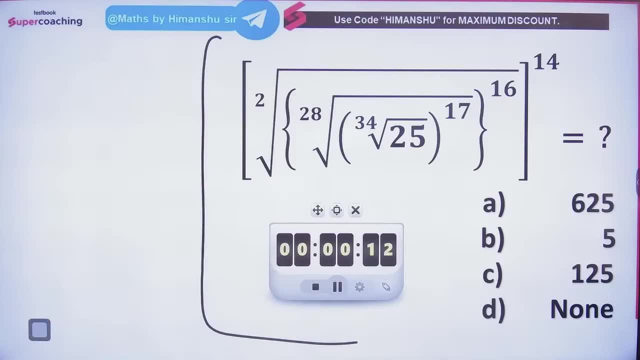 There are more than 40 questions. More than 40 questions. We will see the best way to shine all the questions. Tell me quickly, my son, what will be the answer. All of you Answer me, Tell me, And let's share the session, like all of you, in a great way. 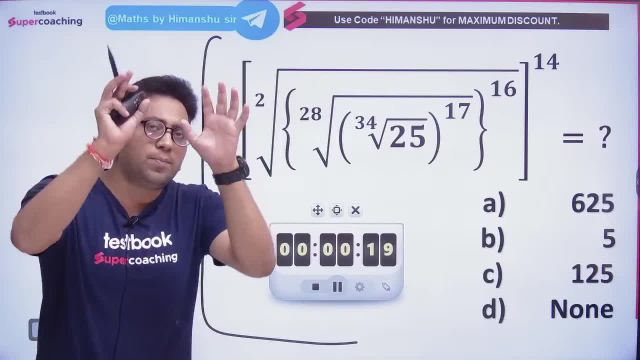 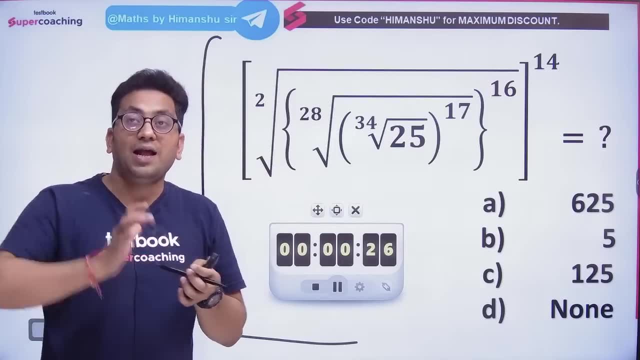 Today the session should be on fire. I say that you have to study any subject. Supercoaching is such a platform for you. You don't have to go anywhere. It happens You have to study from different places. If you study, then there will be confusion too. son. 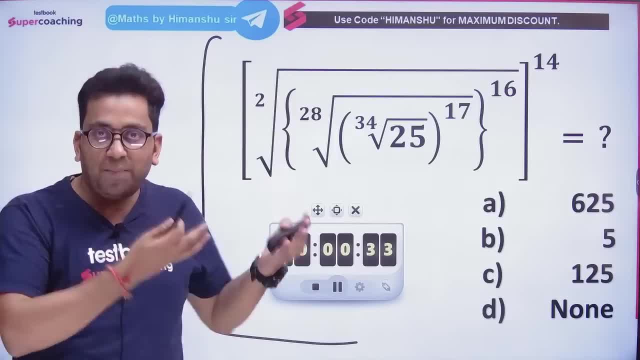 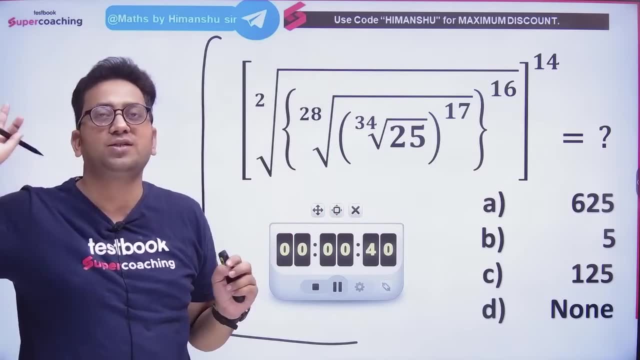 Everyone is making you do it, Is it not? CDP at 11 o'clock, 12 o'clock with me, 1.5 o'clock with Mr Lokesh, then Mr Raj Rana comes and the whole day, son, for you. all the things are provided here on supercoaching. there is no need to go anywhere. 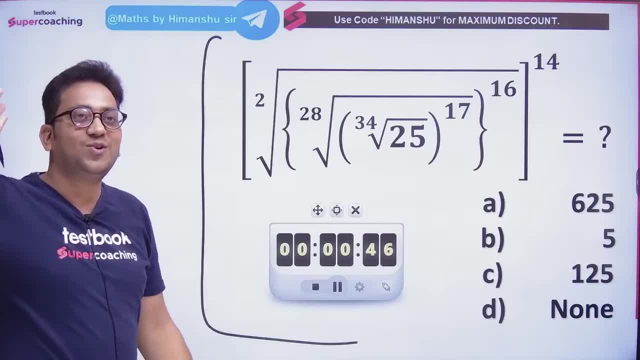 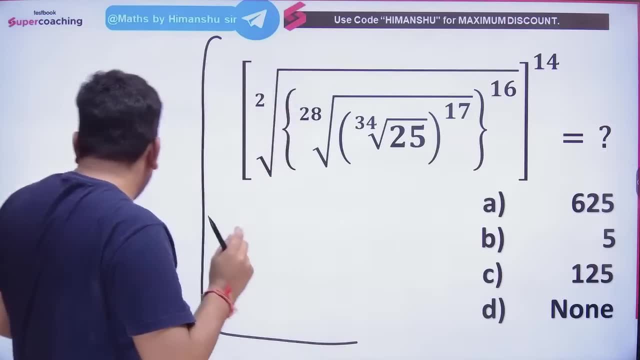 Study at one place, study hard and take the selection, Is it not? Why am I saying, Because I want to eat your sweets, I will not let anyone else eat, Is it not? I am a little selfish in this thing. Come here. 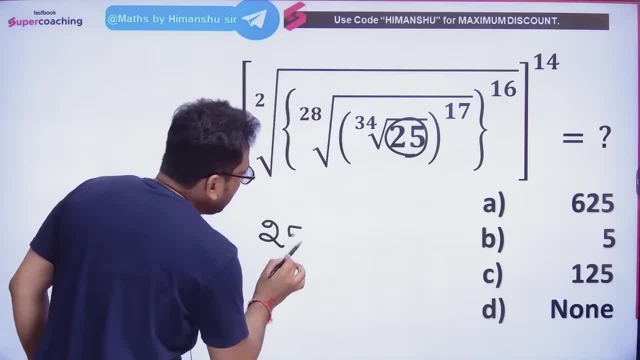 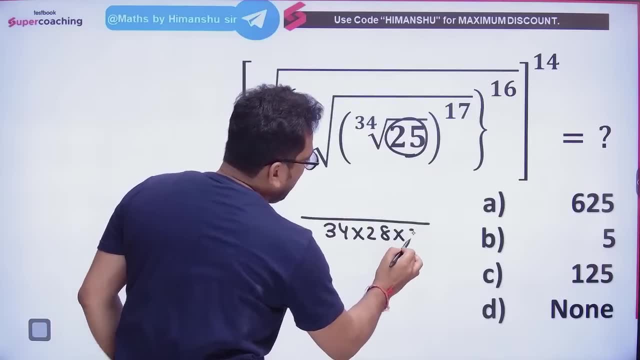 Come here. Twenty-five is twenty-five. See, this is twenty-five. Now see the one that is attached to your left hand. we will put it down. That is thirty-four times twenty-eight times two. And son, what is in the ghat? 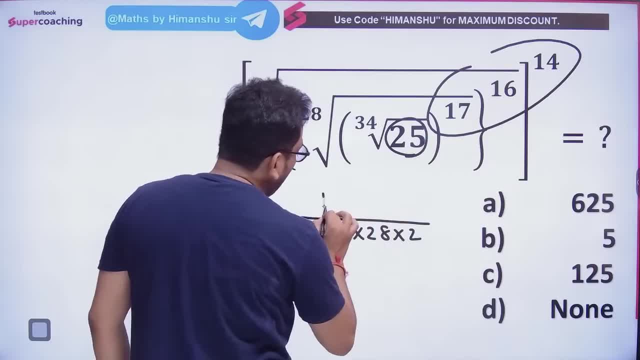 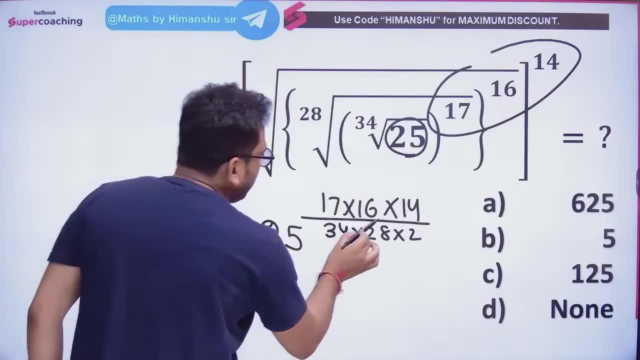 See what is in the ghat. Okay, In the ghat there is seventeen times sixteen times fourteen, Is my thing understood? Now, just solve this. So you will say, sir, it is a simple thing. Seventeen times thirty-four. 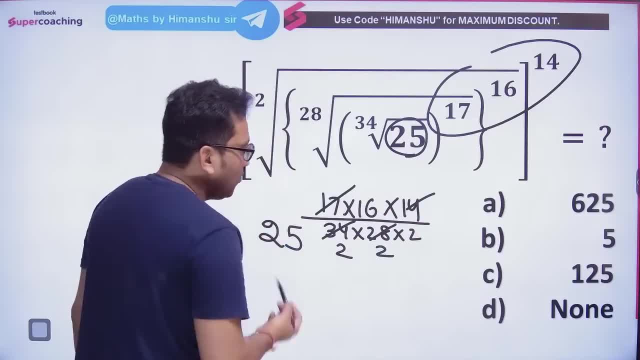 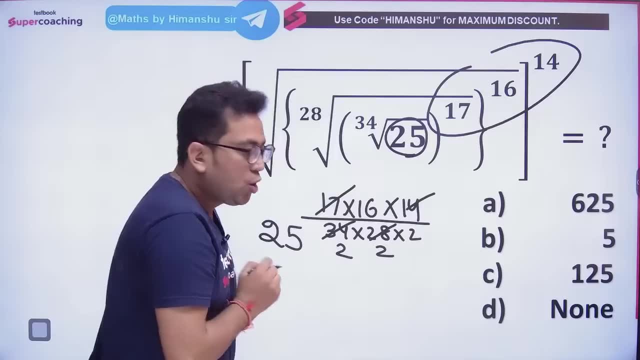 Is it not Fourteen times twenty-eight And see two times four? How many days are there in the ghat? Eight, So there are eight below. There are sixteen above, So there are sixteen days in the ghat. That is, there are two days left in the ghat. 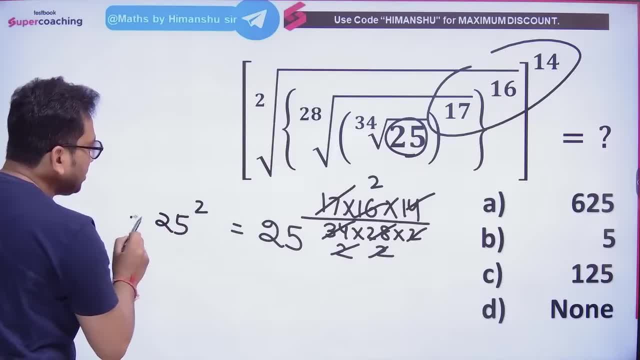 Now, sir, here there is twenty-five times two. So what does twenty-five times two mean? Twenty-five times twenty-five means six hundred and twenty-five. What will come? Six hundred and twenty-five, That is our answer. is option A. 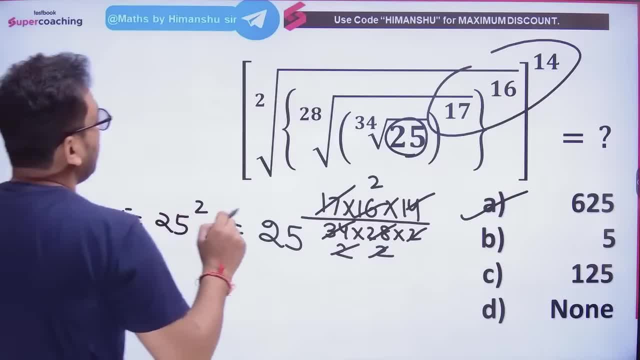 Is it not? The number of children who are answering A is correct. Now see what did some children do? They scored five answers, which is wrong. Son five answers would have come when they would have scored one answer. Son five answers would have come. 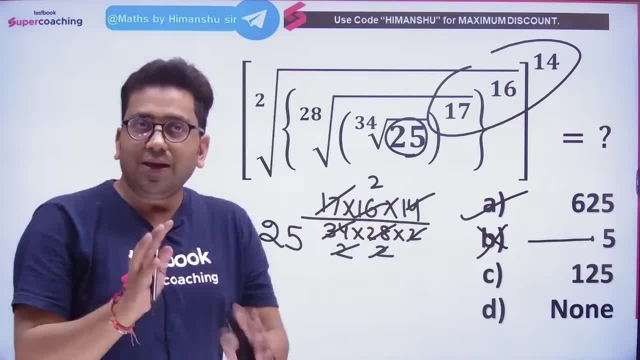 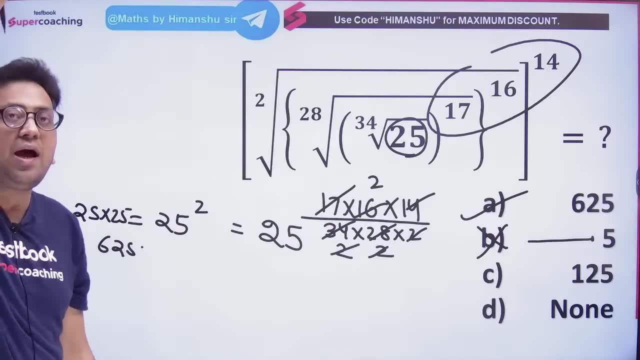 when they would have scored. one answer, One divided by two, would have come the power. Do you understand what I am saying? There is no doubt that the power will always come, down or up. We have to do whatever solution comes Now here. twenty-five times two means twenty-five times twenty-five. 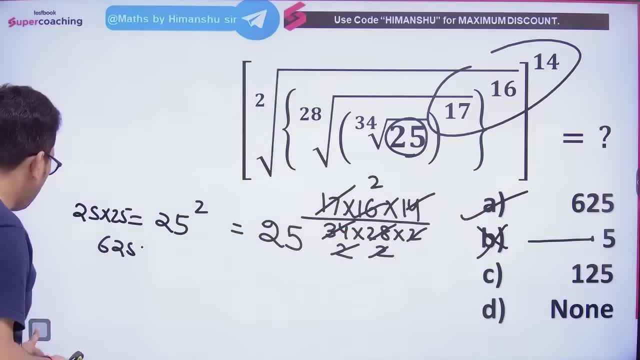 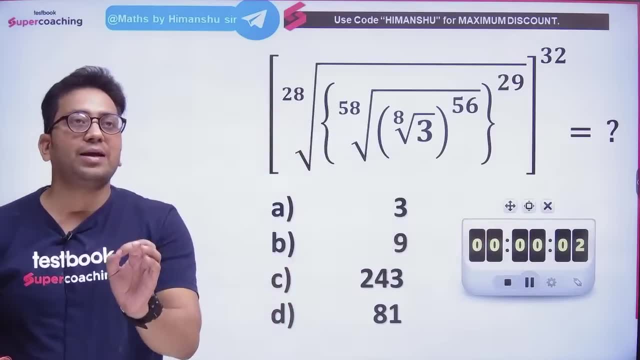 Do you understand? So here, option A will be our answer. Next question. Next question: Shine son, Shine, shine, shine. Answer quickly. Twenty seconds of time has been given to you. Blow the question. Tell me what the answer will be. 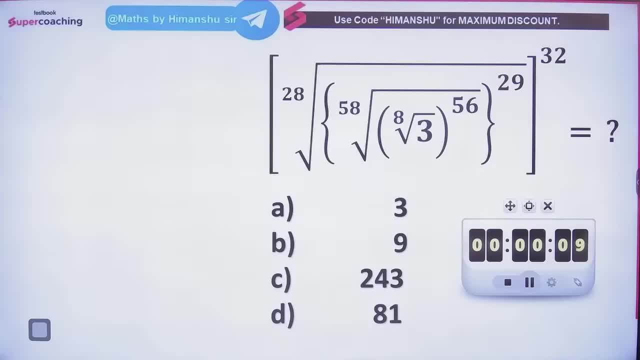 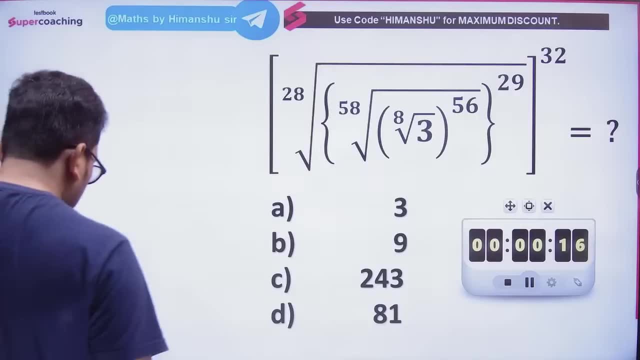 I am right, Very good, Very good, son. Very good, Very good. Fine, Everyone should be right. Brother should not be left. Come on, whatever you are, brother, you are right, you are left. Everyone's answer should come right, isn't it? 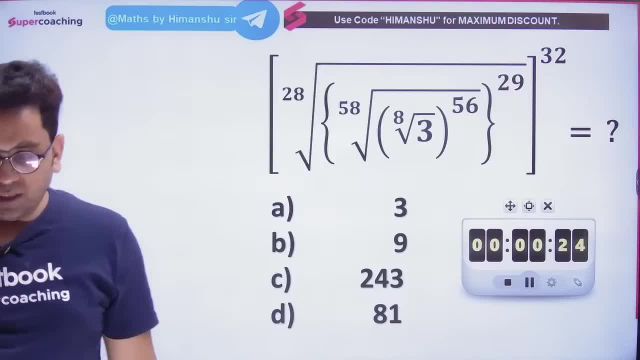 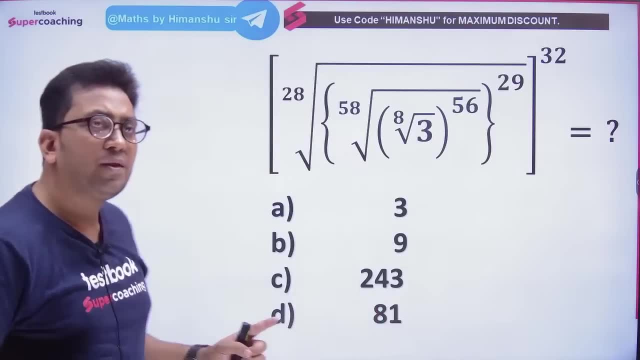 Come on, answer with speed, Everyone's right. Tell me, son, what will be the answer And let's share the session. like maximum, Okay, like and share. should not stop you. Like and share in a great way. Okay, sir, the first one is confused. 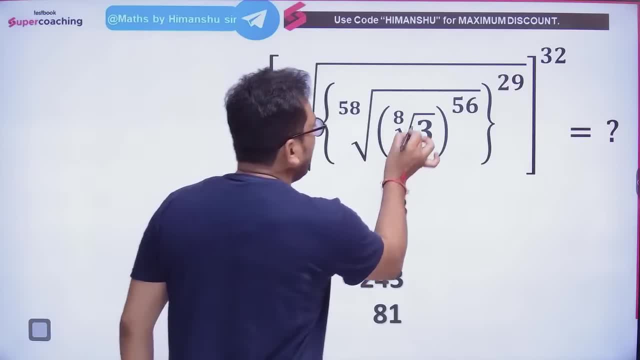 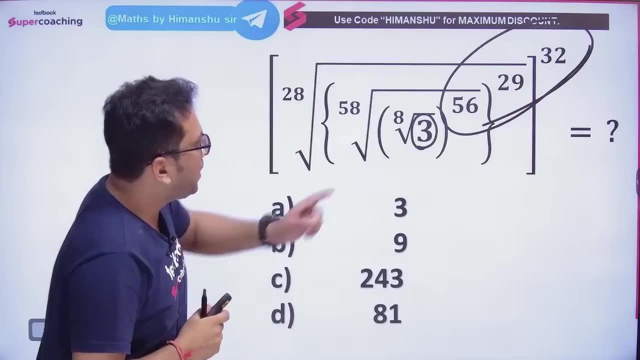 Hey son, let's show the third one. What happened, if there is confusion in the first one? Look here, Look here, my son. there are three, there are three. Now see how much is this ghat. look at the ghat. look at the ghat. see how much is going up in his skull. this ghat is going, so you put it in power. 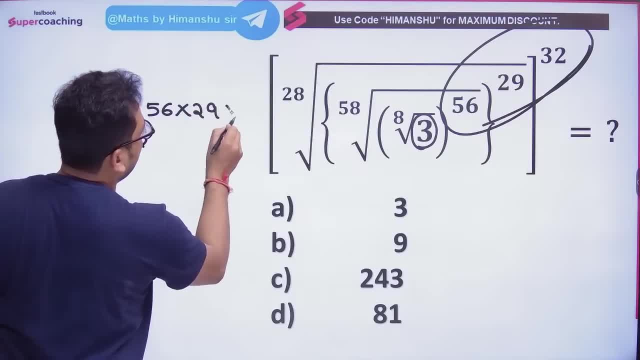 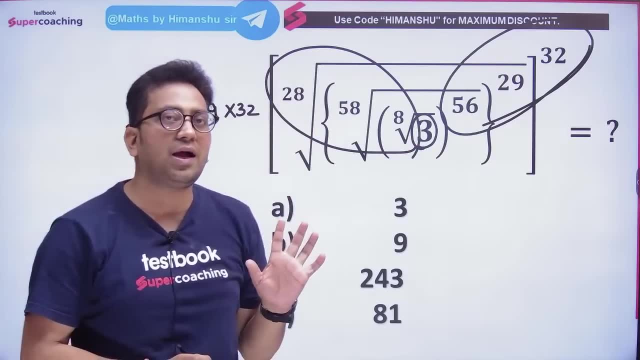 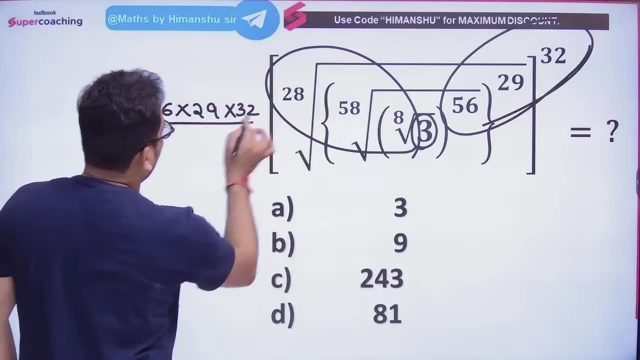 That is fifty-six times twenty-nine times thirty-two right. Now look at the left hand. what is on the left hand? put it down on the left hand. you will remember the concept. why? Because what is the class value? it goes into the divide in the ghat, it goes into the part. so you will remember, you will not have to run. 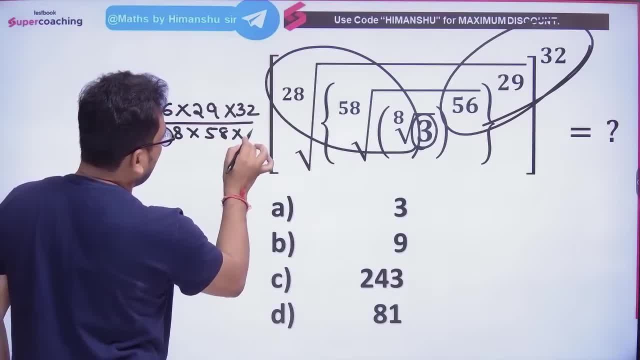 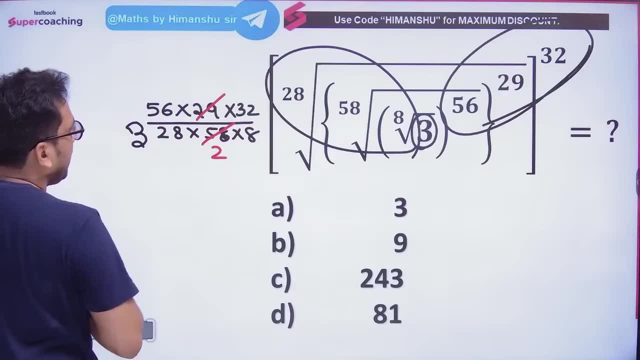 So twenty-eight below Eight, Fifty-five below And eight below. Now come son, let's fly it. Sir, twenty-nine times fifty-eight, It is straight, it will go on two, Is it? Fourteen times fifty-six. 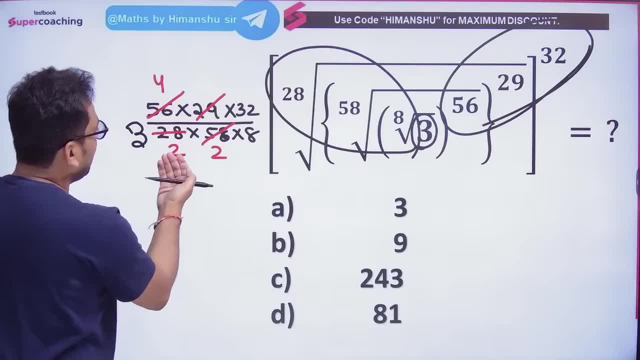 Fourteen times twenty-eight. Is it The rest? twenty-eight times twenty-six. we could have done it too. Let's do it. Twenty-eight times twenty-eight. Twenty-eight times twenty-six. Sir, it went from two to two. 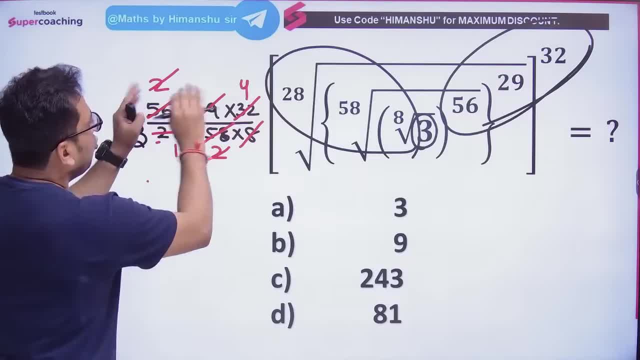 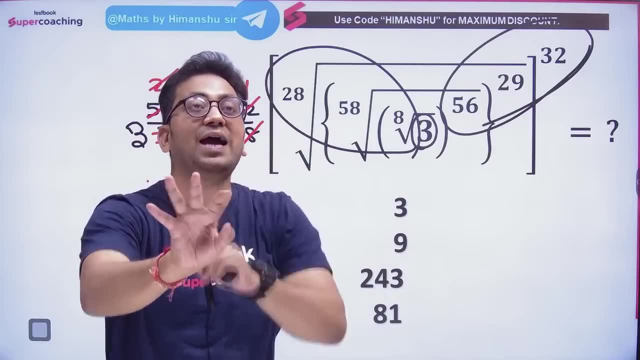 And eight times thirty-two. You see, nothing is left below. There is four left above. That is the ghat. of three means four. Multiply three by four, Three times nine, Three times seven, So I have got eighty-one. 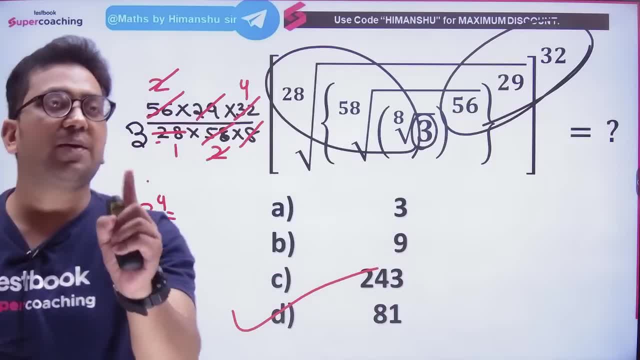 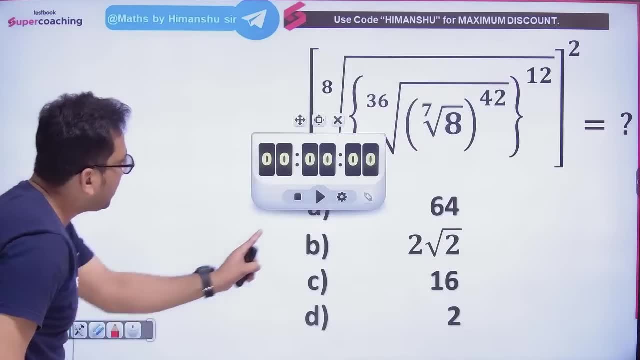 It means eighty-one is my answer. The answer of people who are beating. the answer is correct. The next question is coming. Next question: here it is: Look, let's see how many kids are shining. Let's fly it. The time is twenty seconds. 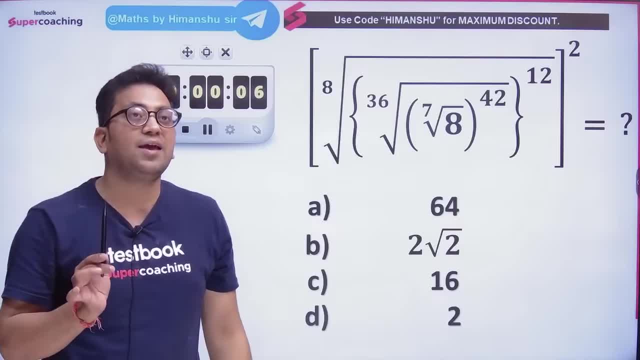 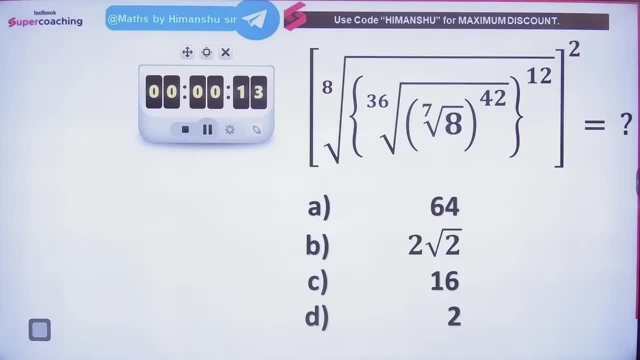 We will blow the smoke, We will make the counting a dessert. Yes, then eat it with pleasure. Come on, it's hot, quickly, No one should get burnt. Fly the question and tell what the answer is. All of you. 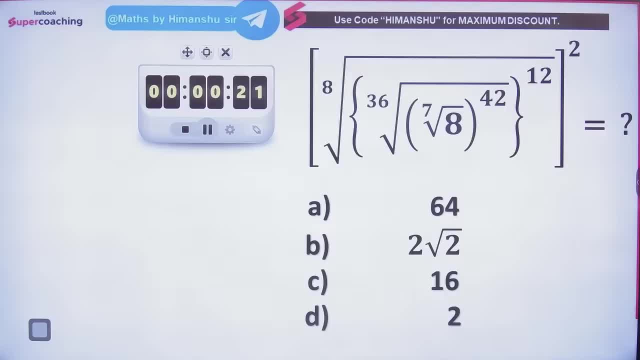 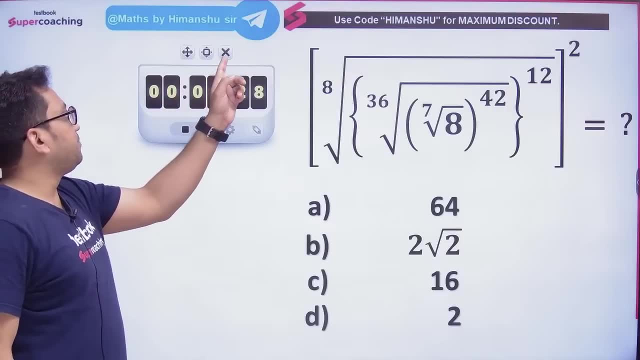 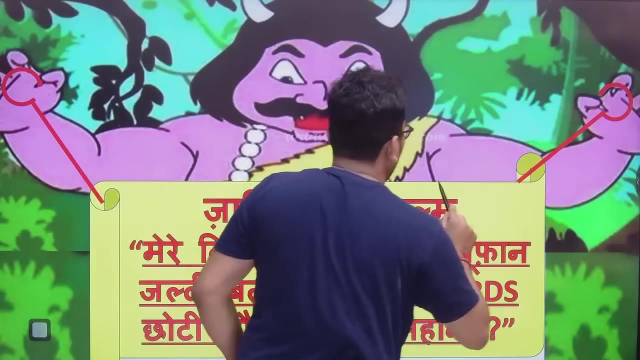 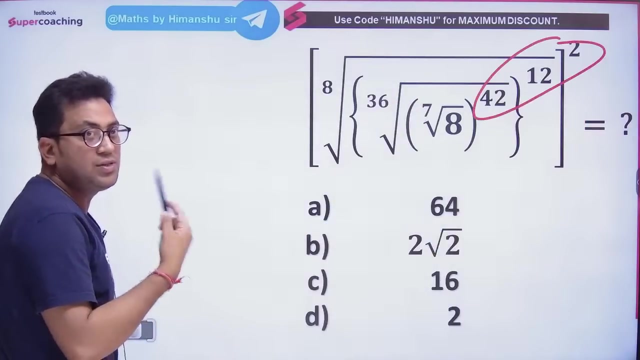 Come, son, let's come to this question. what is he saying to you? give 30 seconds. has anyone got the answer? what will we do, son, in the power, in the power, in the power, we will put it up. this is the last question, son, with this concept, then, the tyrant is bringing another oppression, another oppression, isn't it? 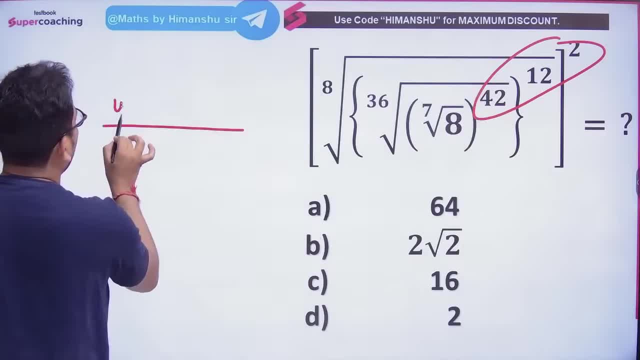 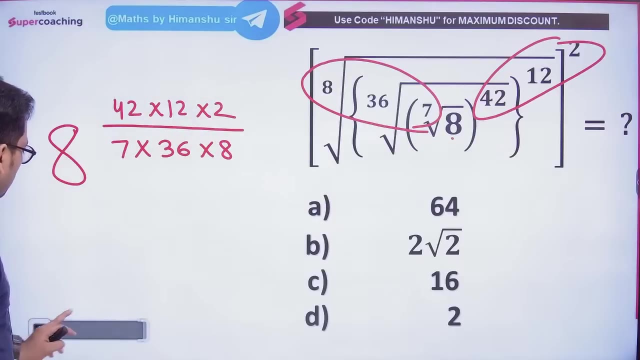 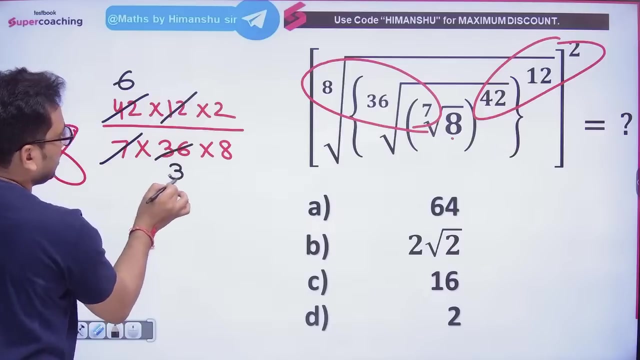 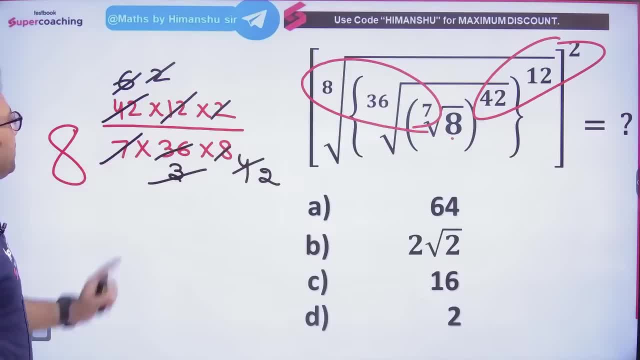 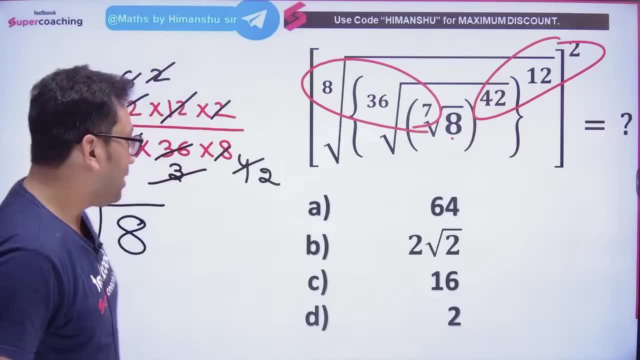 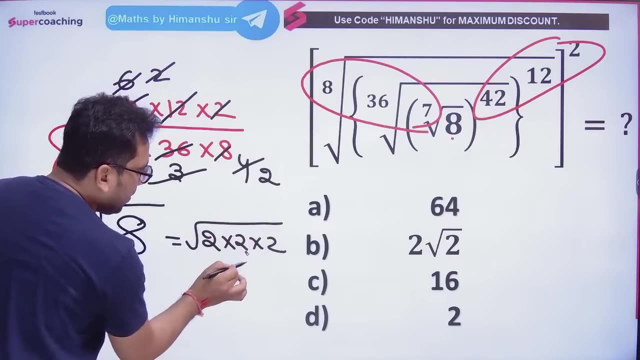 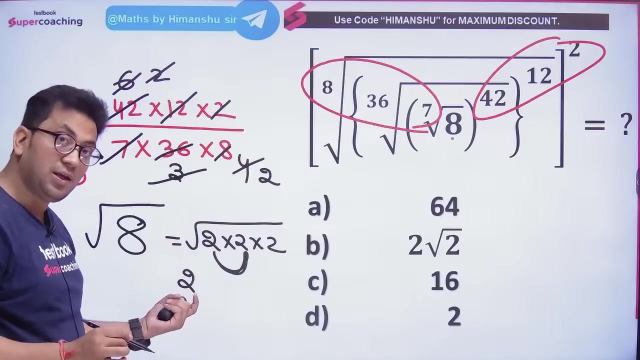 2, 1 less 2 and 2 times 4, now, see, nothing is left above, but 2 is left below. that is this class of 8 has come. now you can understand my words. now how can you write 8, see, understand. you can call 8. 2 times 4 times 8, and if you get the pair of 2 inside the class, it comes out as a single. do you understand my words? there was a mingle inside. it will come out as a single. that is, 1 came 2 and 1, 2 remained inside. that is the answer will come, son. the option will also come. 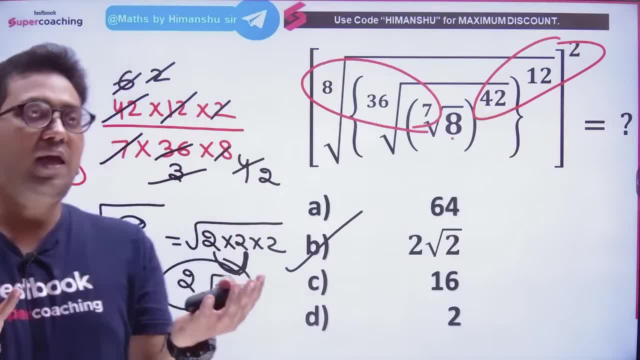 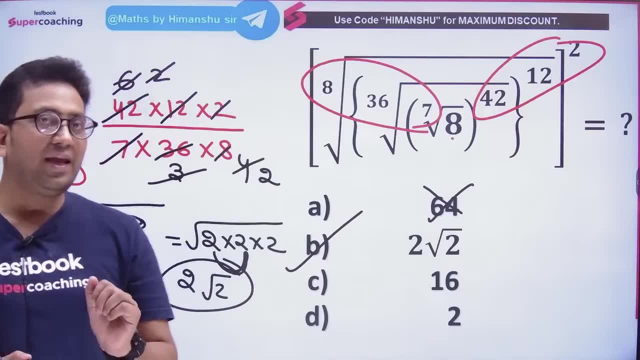 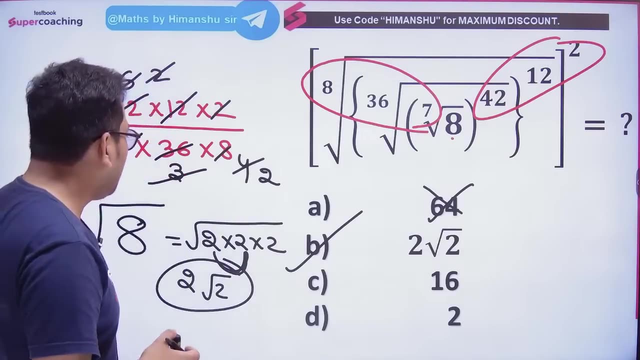 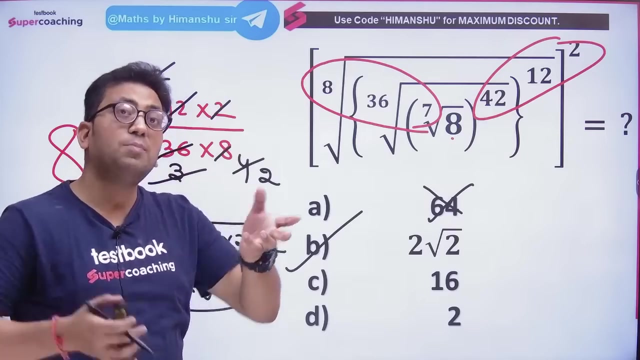 all the children who are typing the answer. their answer is correct, brother. I can see that some children are also answering 64, so here they are wrong. why? because they do not have to do the class of 8, what they have to do, they have to see it easily. so they put the square of 8, hey, the game is not going on. it is not going to happen like this, that whatever I want to do, I will give it to him. it is not like this son now think. even God started thinking like this: whoever I want to do, you also come up, you also come up. 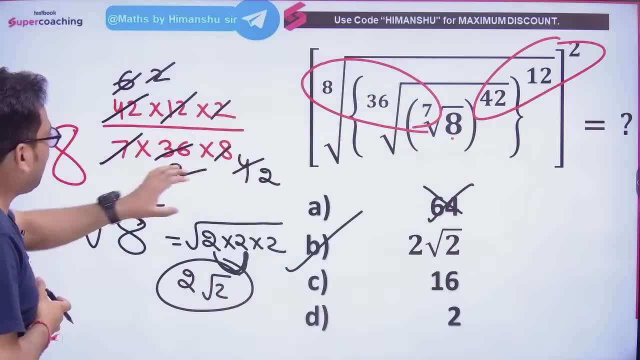 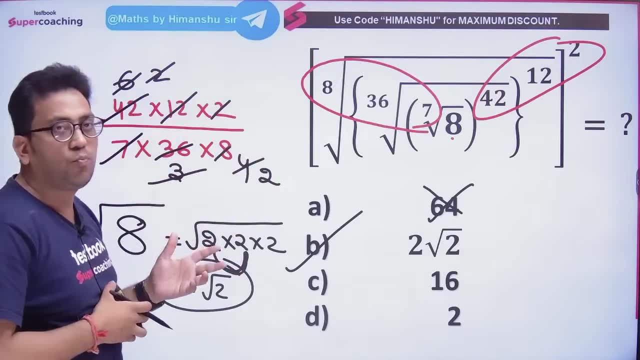 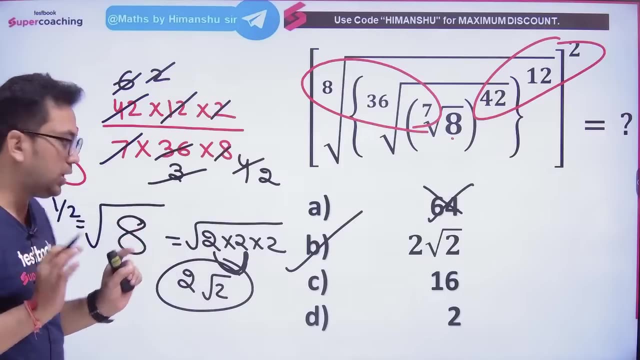 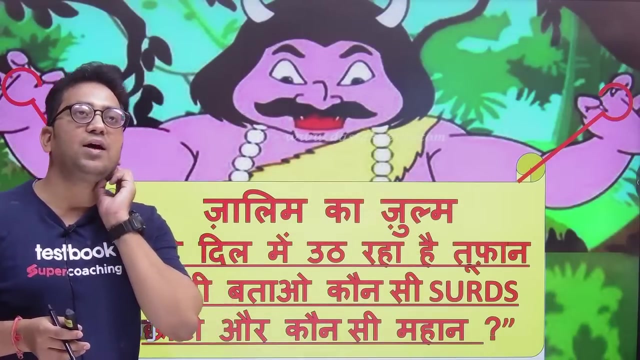 where it has happened. hmm, this is also a number. ok, you are his son, you are their God, so don't call it up all of a sudden. let the one who is below be below, call whoever is above. ok, what will happen below? what will be the meaning of the pie of 8,? what will be the difference between one and two? what will be the root art? it means that it will happen. let's go, brother now. let's come, brother next, next, next, next, next, next. 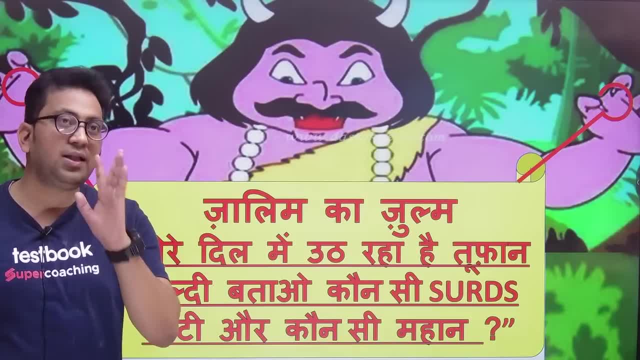 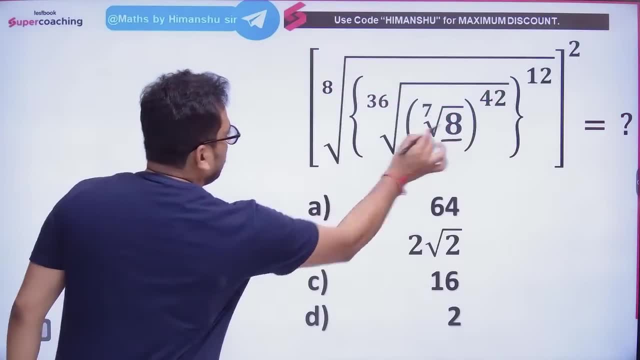 I'll tell you, you will have to do meditation, you will have to do penance. Okay, it will not be like this, son, come here for a while. see the door again. son, see how much is the weight of 8?. 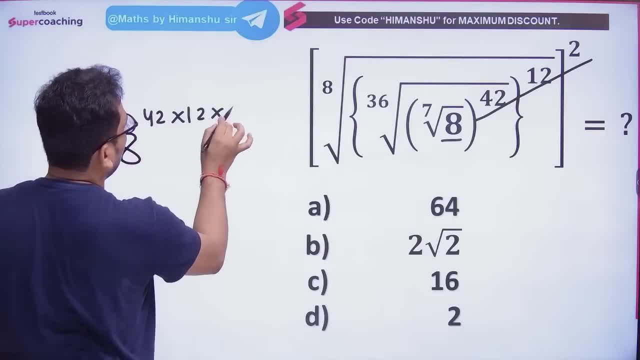 See how much is the weight of 8? 42 times 12 times 2.. Okay, son, now come down here. what do you have? 8 times 36 times 7, tell me what was the practice at this time. 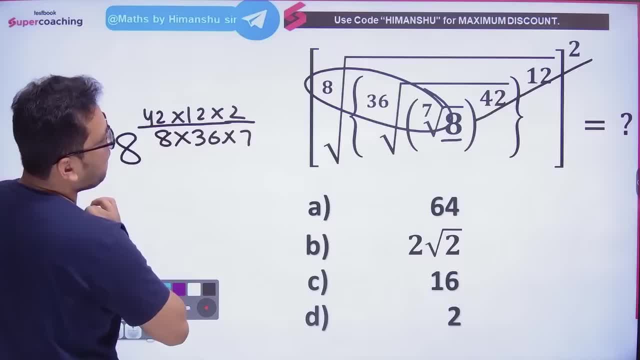 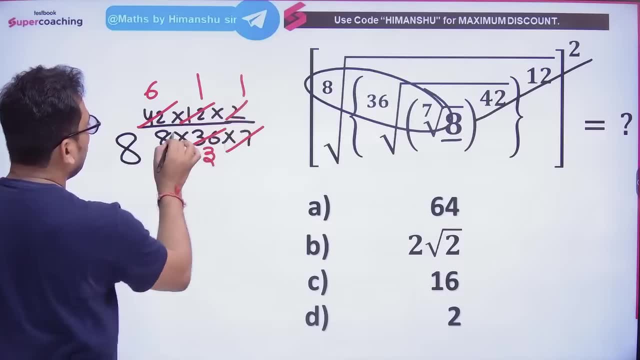 Son, I don't know how to cut. learn to cut. This is it? see: 7 times 42, okay. 12 times 12,. 12 times 3 is 36, understand. 2 times 2,. 2 times 4 is 8, understand. 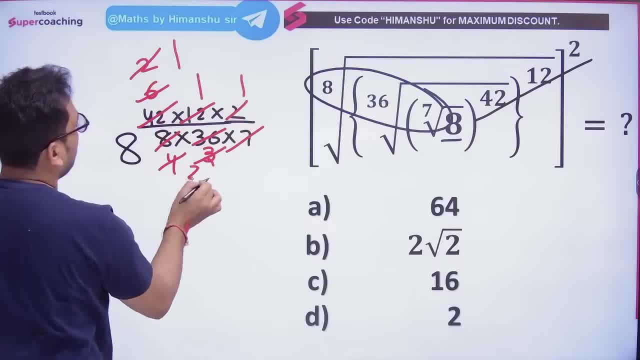 3 times 3,, 3 times 2 is 6, now 2 times 2, 2 times 2 is 4,. tell me, is there anything left above the practice? No, son, there is 1 left. what is left below 2 is left. that is, the weight of 8 is 1 divided by 2.. 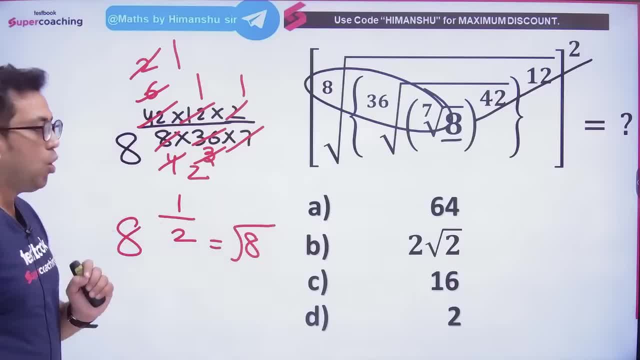 Now do you know what is the meaning of 1 divided by 2? practice? It is root 8,. and what can I call root 8?? 2 root 2,, brother, this is what I explained to you. Okay, come on, let's see the next question. 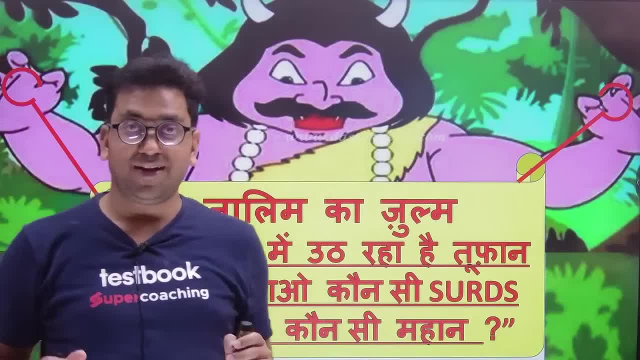 Now look here. What is the tyrant saying to you? Look at the next tyranny of the tyrant. pay a little attention. What is he saying? A storm is rising in my heart, Oh brother, a storm is rising in his heart. 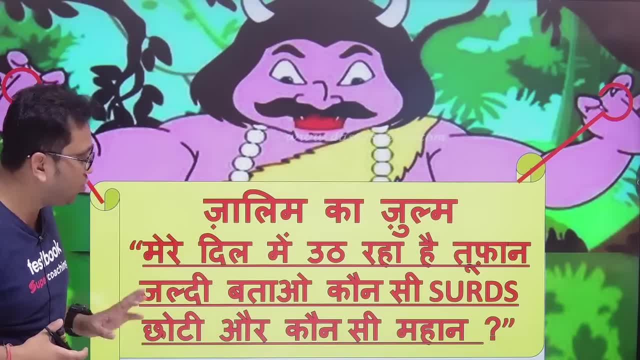 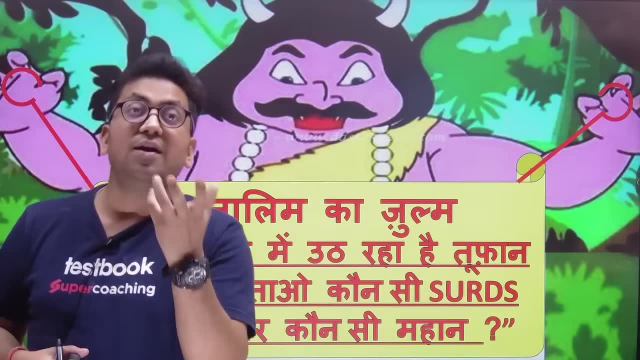 See what he is saying. Tell me quickly which is small and which is great. So what you are simply doing is coming from sad. In Hindi, we call sad as karani, Isn't it ghatank and karani. So now we have talked about ghatank, we will also talk about karani. 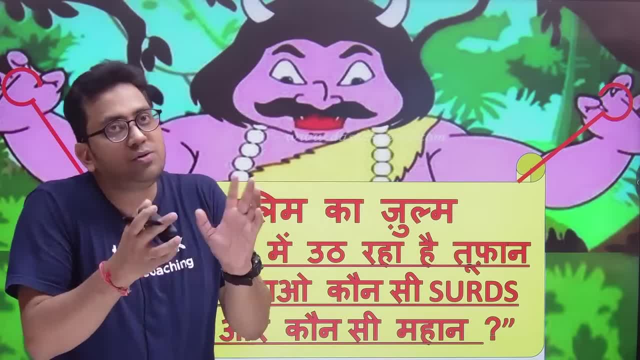 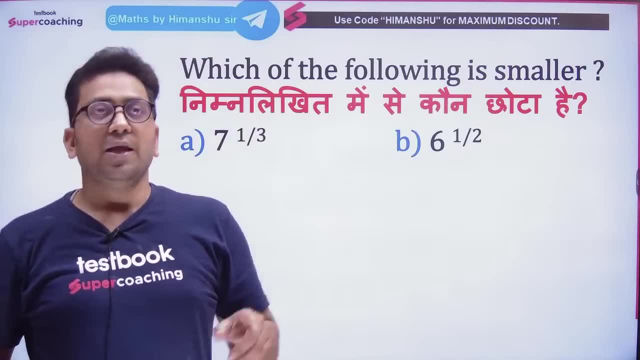 So he is saying here: tell me which is small and which is great. Now, what is this? Let's come to this. This is it. First, we will understand the concept and then we will highlight the questions. First of all, I want to ask you this question: 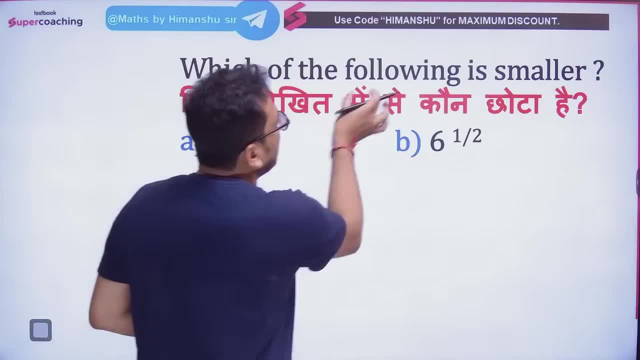 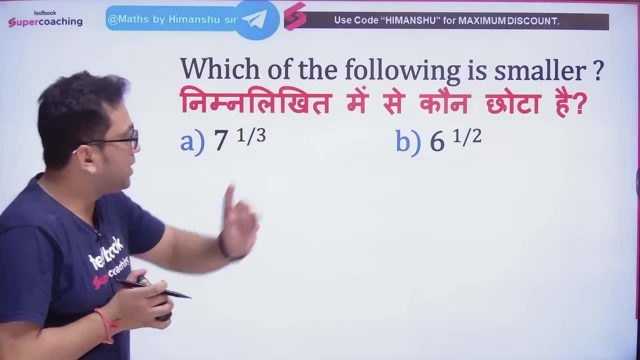 There are only two options. You have to tell me this: Which is the exception from the non-written, That is, is this an exception or is this an exception? This is 7's ghat 1 divided by 3, and this is 6's ghat 1 divided by 2.. 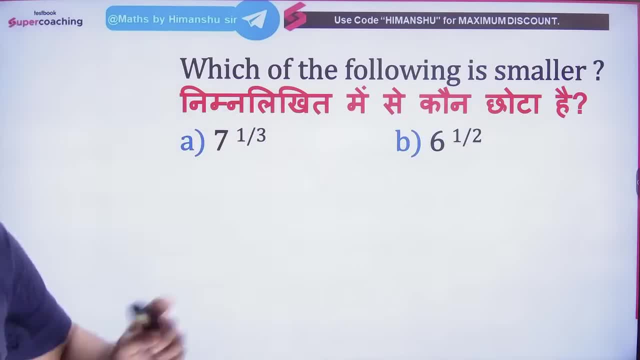 Come on, let's highlight, Tell me what will be the answer. Let's see How many children are able to answer that. which of the non-written karani is small. Which of the non-written karani is small. Which is small? 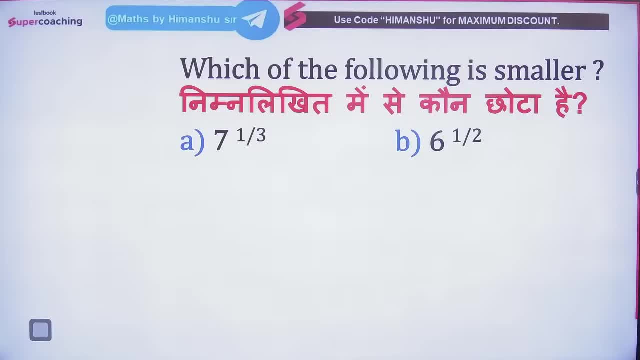 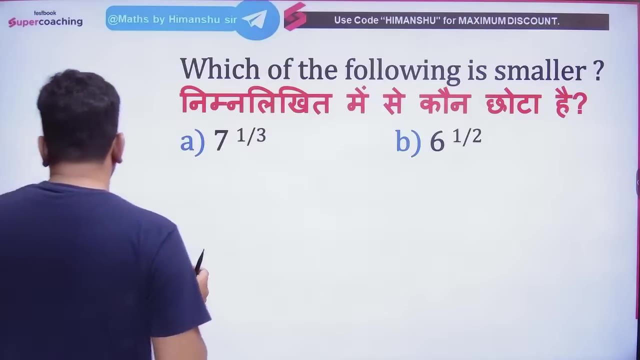 In which of them is which small? Tell me quickly what will be the answer: Everyone's and all. Tell me, tell me, tell me. Let's answer everyone's and all. child, Look, you have to tell me which of the non-written karani is small. 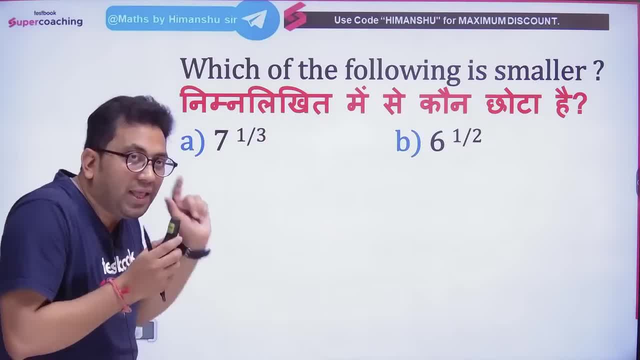 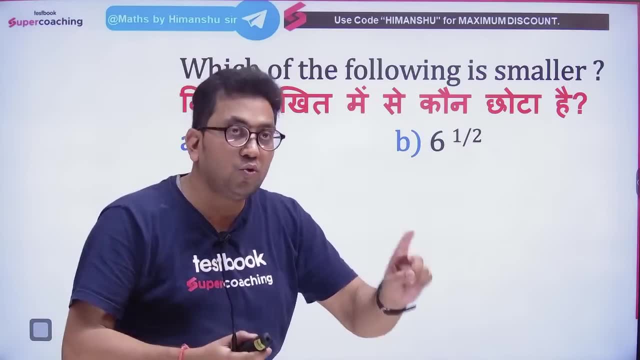 It's release. Hold the release. Catch the neck of release Quickly. tell me who is you feel release. you will be able to hold his neck, but sometimes what happens is that you can also hold the wrong neck. Why I will tell you. Look, you see carefully that if the power was the same, that is, if the power was. 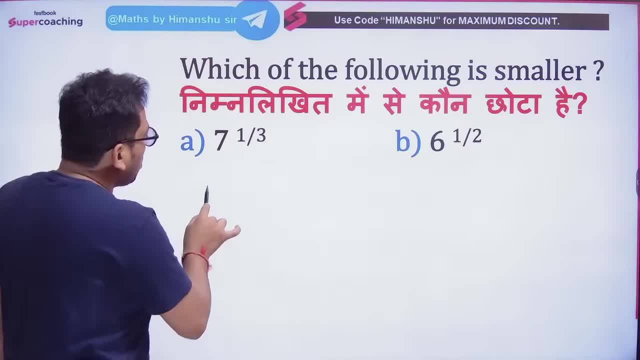 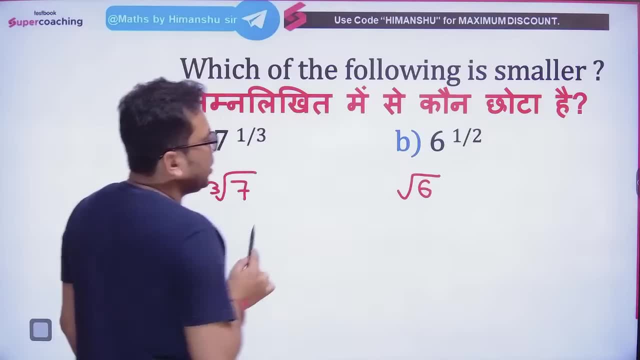 up and not down, then there was no problem, because the child does not know what will be the cube root of 7 or what will be the square root of 6, that is, what will be the class value of 6 or what will be the mass value of 7. 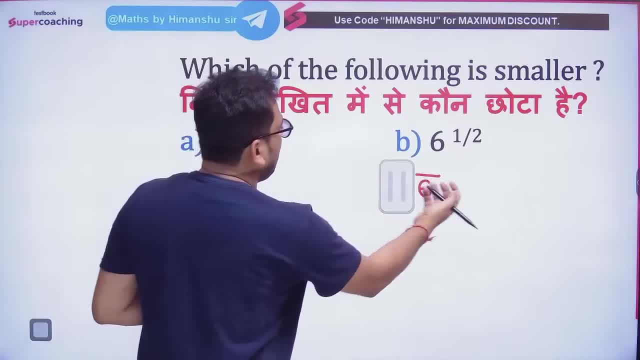 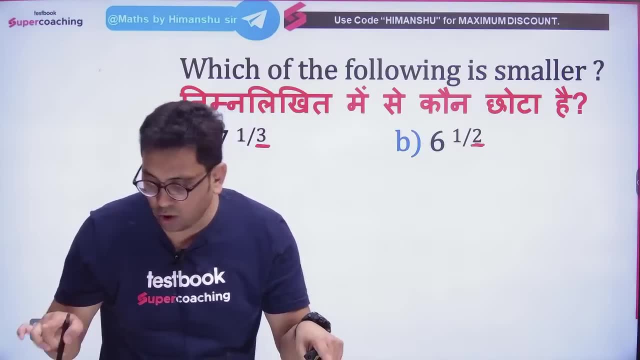 No, I don't know, I have to take it out. So what will he have to do? I am telling you what you have to do. You have to look down below 3 and what is this? 2. Look down below What is below 3 and 2.. 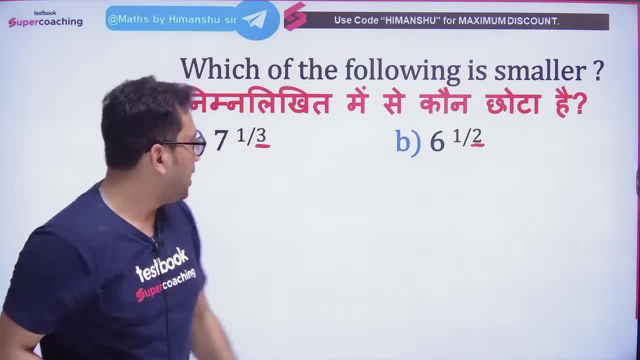 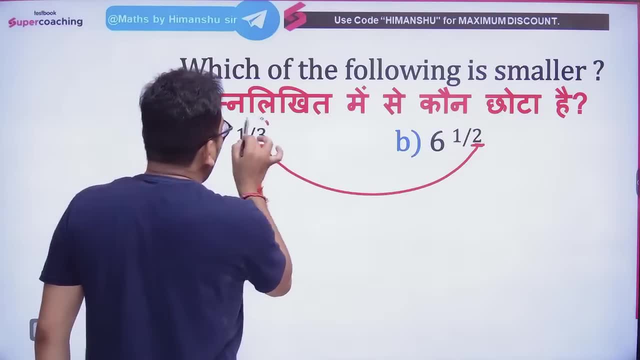 Take the LCM of those who are visible below, That is, take the LCM of 3 and 2.. He will open his mouth and come 3 times 2 is 6.. 6 LCM has come From that 6, you do the multiplication of this mass. 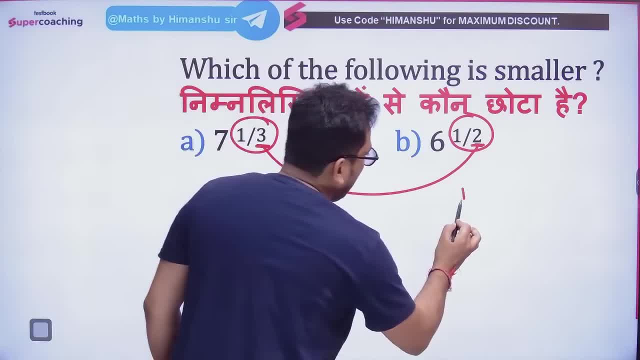 That is, the multiplication of 1 divided by 3 is 6, and here the multiplication of 1 divided by 2 is 6.. Do you understand my point? So look, if you do the multiplication, then 2 came, and if you do the multiplication here, then 2,, 3,, 6 came. 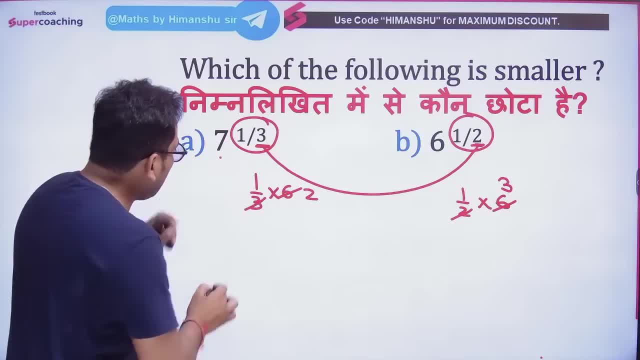 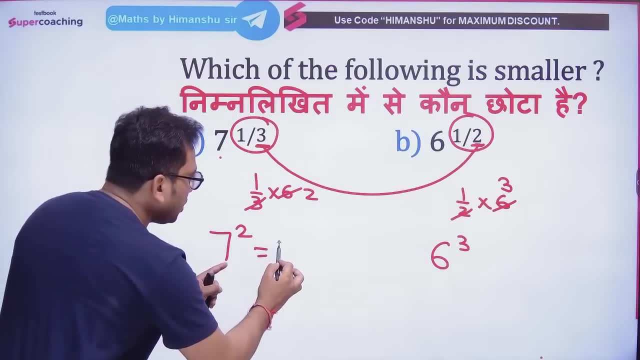 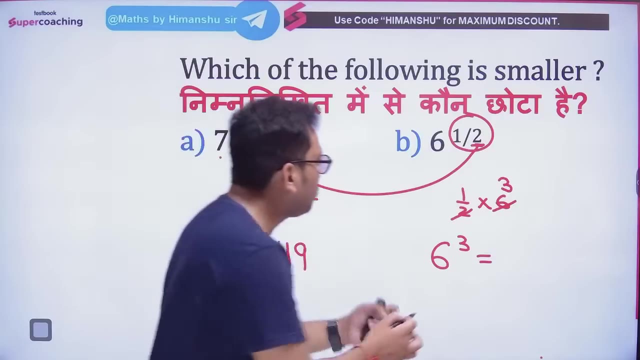 Now what has come up? it means that the mass of 7 has come 2.. It means that the mass of 6 has come 3.. So the mass of 7 has come 2 means 7, 7,, 49,, 7,, 7, 49.. The mass of 6 has come 3 means 6, 6,, 36,, 6,, 216.. 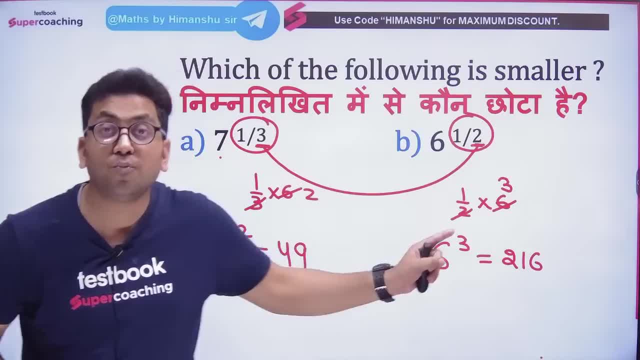 That is 6,, 6,, 36,, 6,, 2,, 1, 6.. Now tell me which one was small. It was small. It looks small, but it is small. It looks small, but it is small. 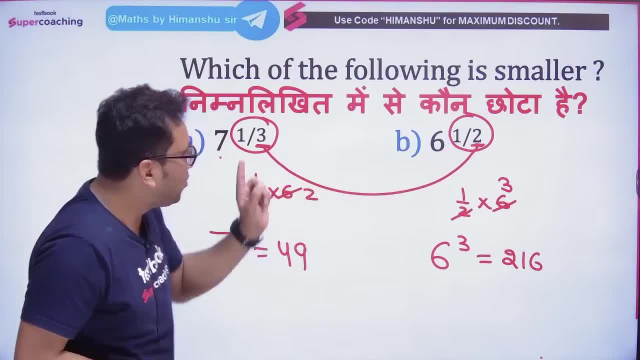 Do you understand my point? So you had caught the wrong neck. Those who had caught the neck of B, they had caught it wrong. Who had to hold the neck Of A? A is small. Do you understand my point? How to shine. 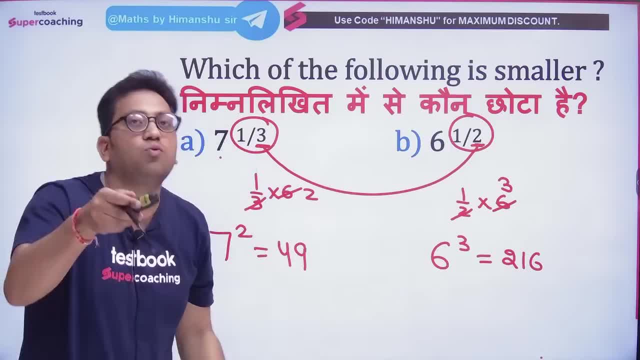 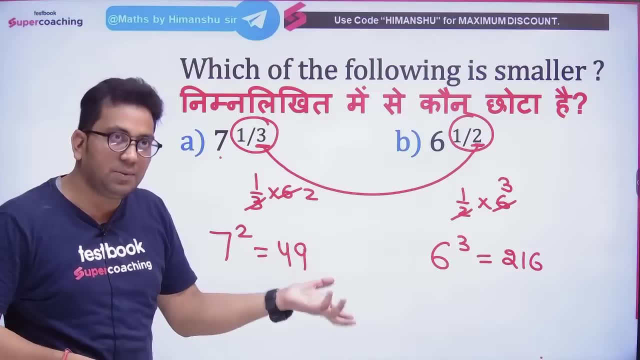 Look below What numbers are visible below. Take the LCM of the numbers that are visible below And the number that will come. do the multiplication of this mass with it and blow it. You understand right? Shall it increase further? Hey, I understood. 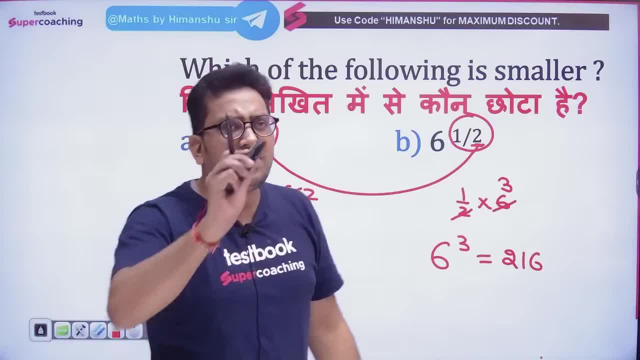 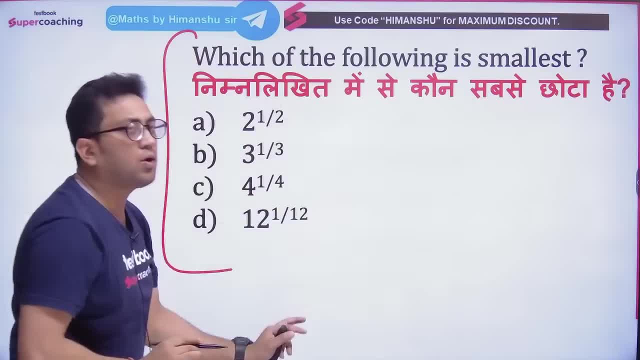 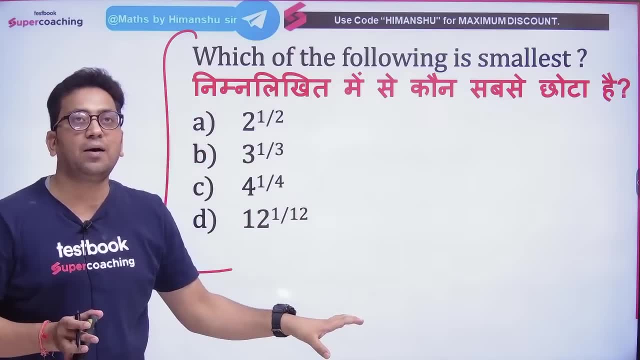 Next question is coming Here, it is in front of you. Tell me quickly, Tell me quickly Which one is the smallest among these. Which one is the smallest? I am saying that in BPSC your elementary math will come, son. 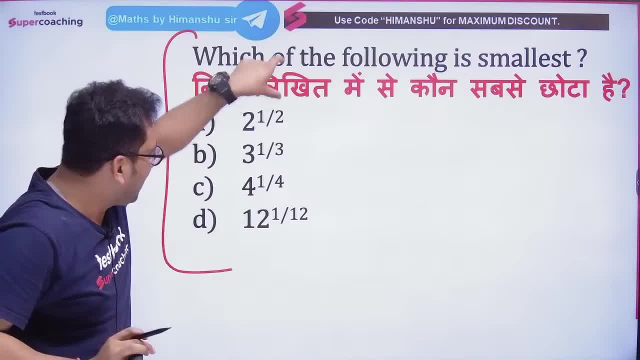 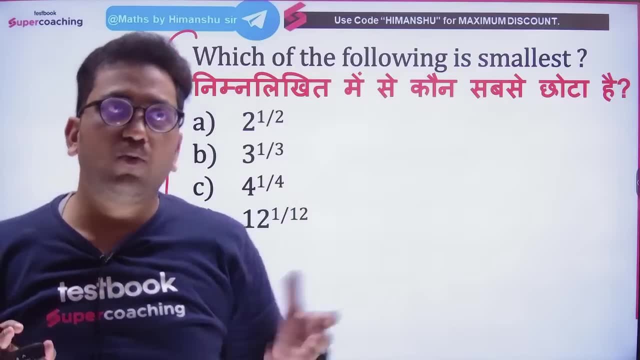 It is going to increase one level. You got to know this thing right Now. here he will ask you such a question Because this number will raise the question from the subject. He will say: the question is in the number system, brother. 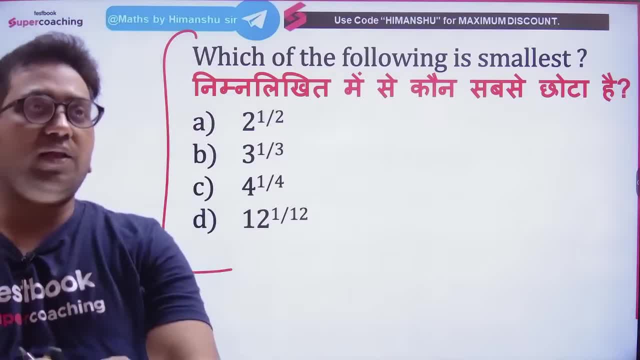 What should we do? Tell me: Okay, Come on, come on, come on. What will be the answer? With speed- See what he is saying, Sir- the numbers are different. Very good Power means the values are different. 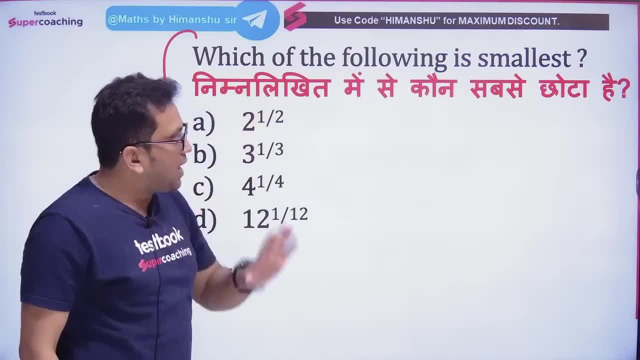 Even more good. Do you have to take tension? Absolutely not. What will we do, Sir? we will see below What is visible below son 2,, 3,, 4 and 12.. Sir, what will be the LTM of 2,, 3,, 4 and 12?? 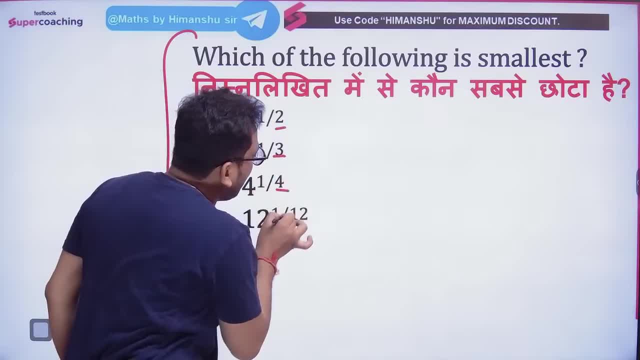 Oh, it will be 12.. Oh yes, right, Then multiply by 12.. That is, 1 divided by 2 is multiplied by 12.. 1 divided by 3 is multiplied by 12.. Sir, what is the LTM of 1 divided by 3?? 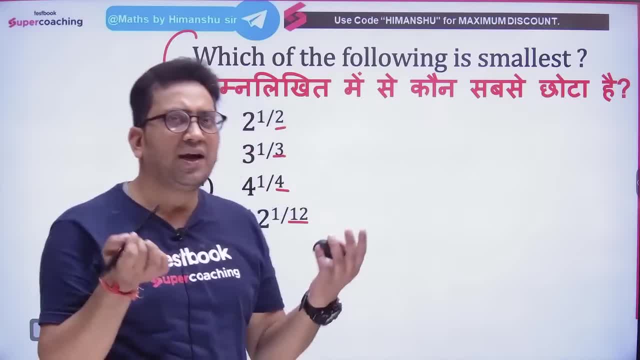 Sir, what is the LTM of 1 divided by 3?? Sir, what is the LTM of 1 divided by 3?? Sir, what is the LTM of 1 divided by 12?? Oh yes, right. 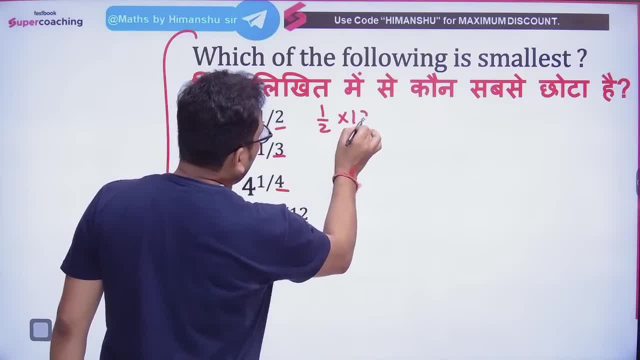 Oh yes, right, Then multiply by 12.. That is, 1 divided by 2 is multiplied by 12.. 1 divided by 3 is multiplied by 12.. 1 divided by 4 is multiplied by 12.. 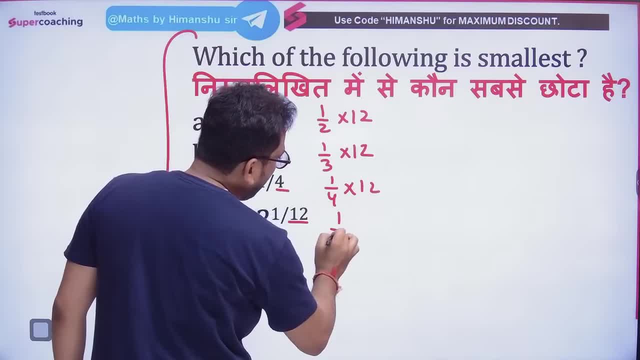 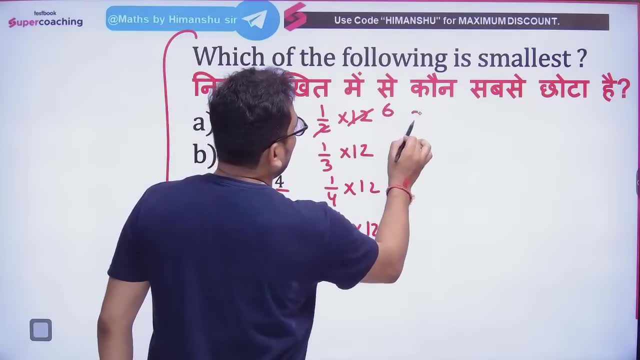 Yes, And 2 divided by 12 is multiplied by 12.. Say yes or no. Say yes or no. Now sit down, son. 226phoria12 means the LTM of 2 is 6, 324bild12 is 4.. 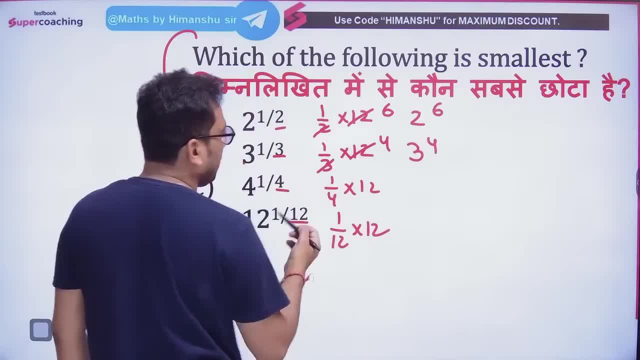 That is what I hope you understand. We will keep taught the LTM of this first. The LTM of 4 is 12.. So the LTM of 4 is 3.. If 12 is less than 12, then will not be the LTM of 12.. 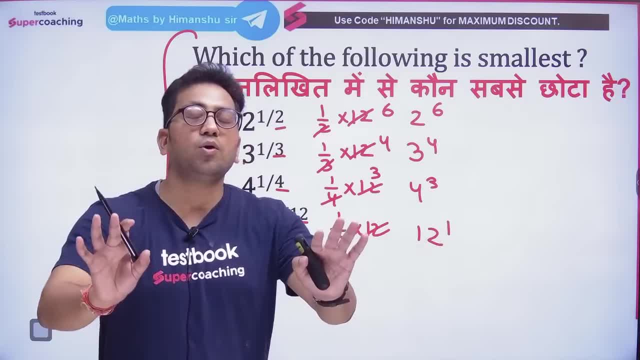 Now see what will happen of 12? Yes or No? I mean, if there is a blind person, he will tell you by touching. he will tell you by touching: this is small, this is small. he will tell you by touching: this is small. 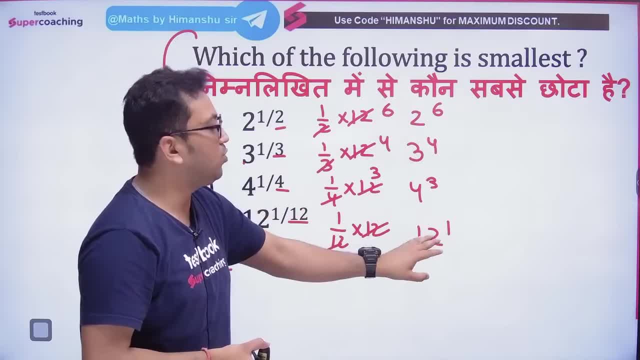 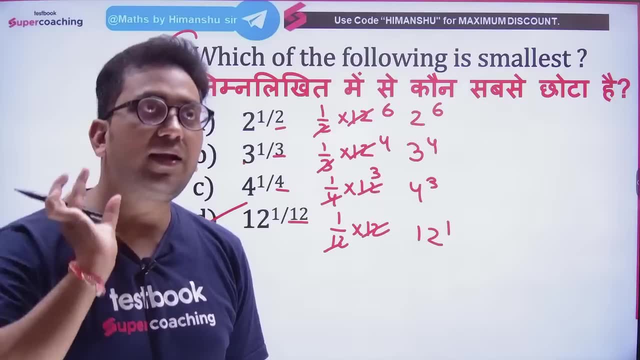 Why There is only one limit of 12,. if you solve any problem, it will increase. So this is our answer. that is, D will be our answer. D will be the right answer. Are you understanding? Are you understanding the thing? 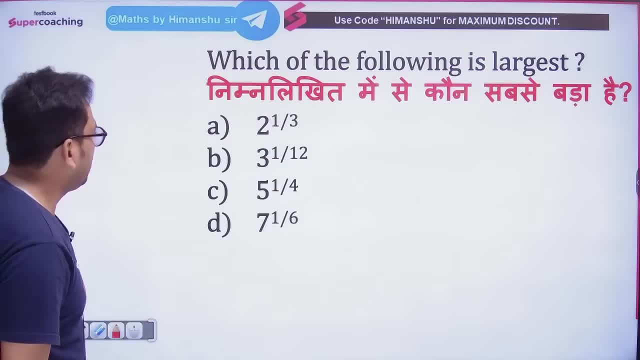 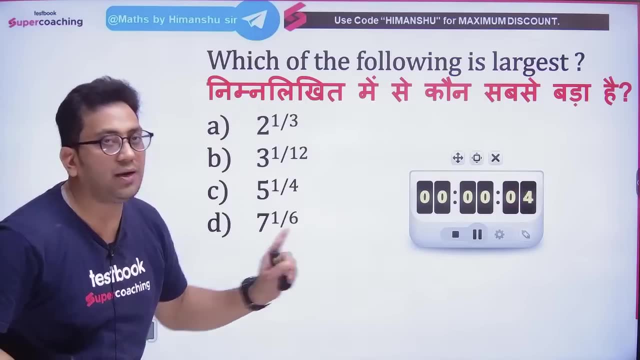 Let's move ahead. next question. next question: Chamkao Mindalal. I want an answer from every child, the child who is watching the session. each child will answer. I am giving time of 30 seconds. 30 seconds. every child should get an answer. come on, tell me what will be the answer, all of you. 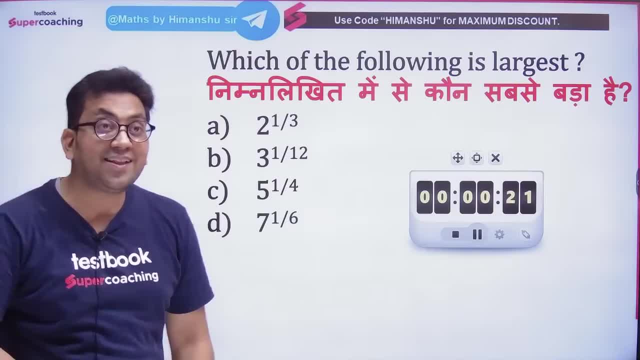 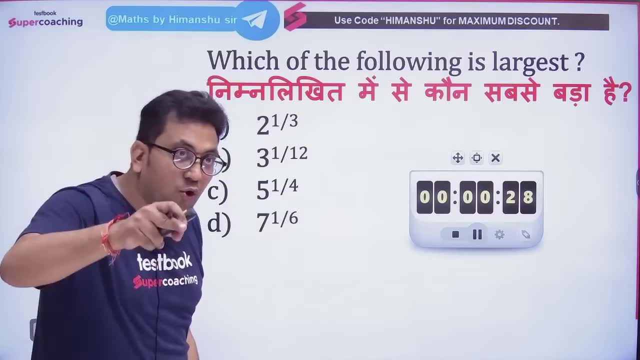 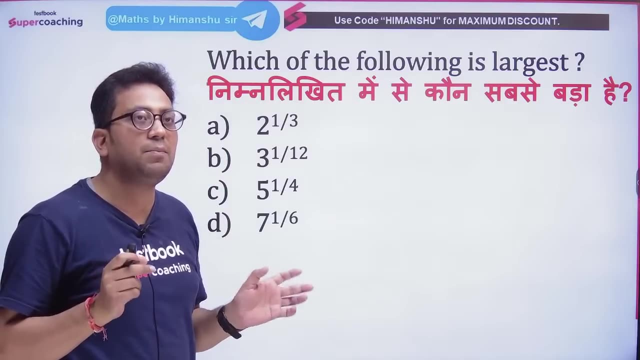 What is being said: look down, look down. that child used to say: look back, look back. I am saying now, look down, look down, look down. what is down. take the LCM of whatever is there and do the calculation of that LCM. here the time is ending. I can see the child A B D. A B D. 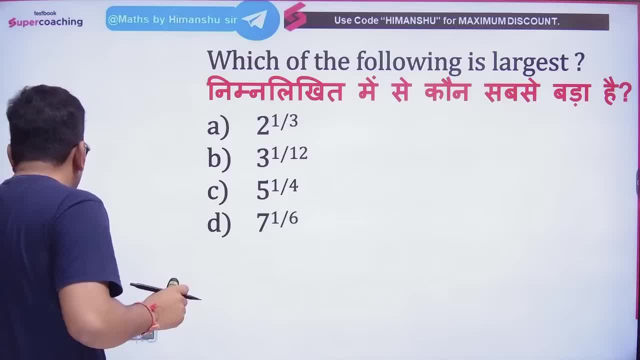 now there are a lot of children going towards B. some are answering A, D, A, D. come on, brother. there are 3 below, there are 12, there are 4, there are 6, then take the LCM of them. 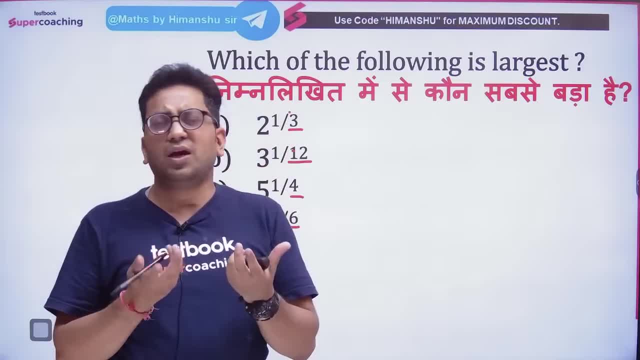 Sir, how do we get the LCM of 3,, 12,, 4,, 6,? Sir, we don't know. I say: look at the big number at this time. which one will you say 12,. 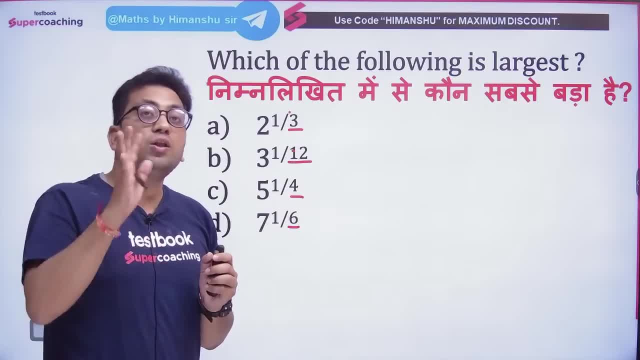 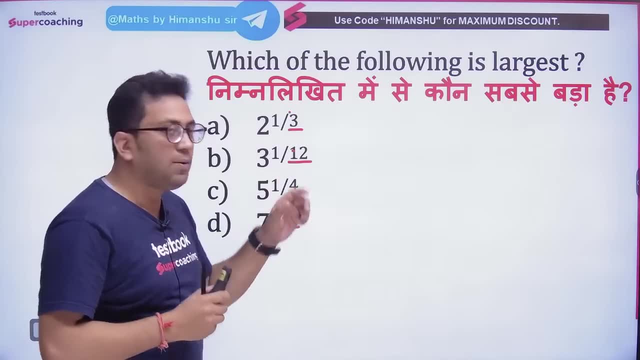 then read the mountain of 12, 12 times 12. And see if it also comes in the mountains of other numbers like 12 comes in the mountains of 3, 3 times 4 is coming, 4 times 3 is coming, 6 times 12 is coming. that means 12. LCM is there. 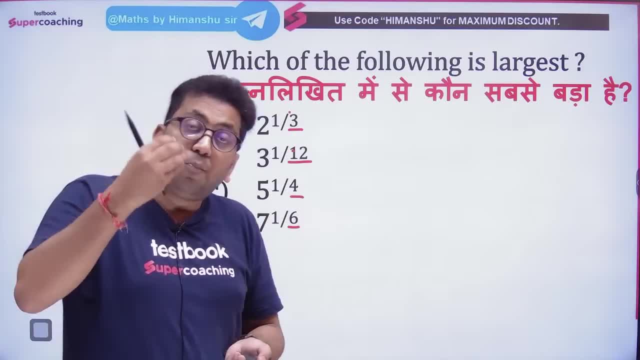 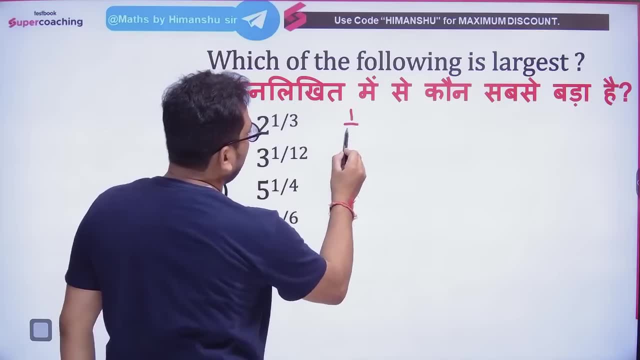 do you understand what I am saying? 12 LCM is done. you can find it very easily by taking the big number and reading the mountain. now 12 has come. now our child will multiply 1 divided by 3, by 12,. 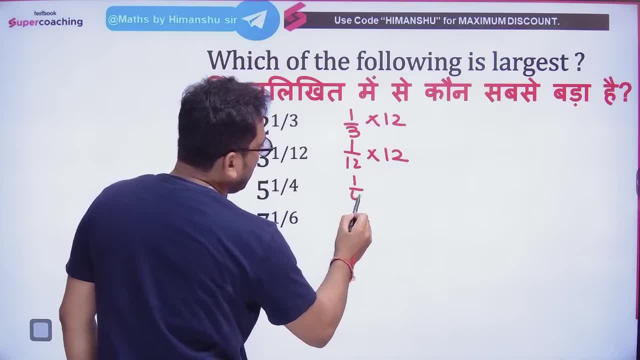 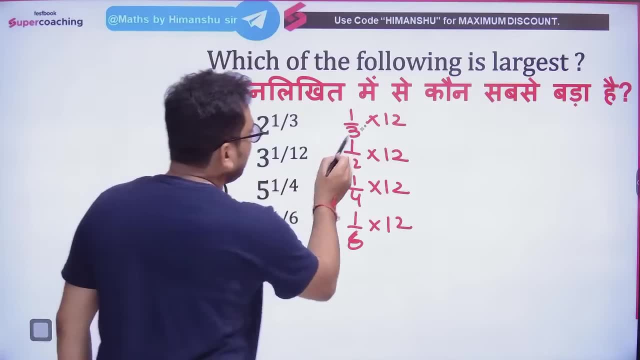 then 1 divided by 12 will be multiplied by 12,, then 1 divided by 4 will be multiplied by 12, and then 1 divided by 6 will be multiplied by 12, say yes or no. What will you say, Sir? 3 times 4 is 12, that means the value of 2 is 4,. 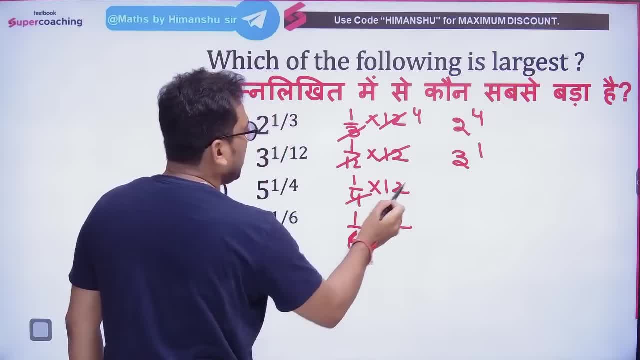 Sir, 12 times 12 is gone. that means the value of 3 is 1,. Sir, 4 times 3 is 12,. that means the value of 5 is 3, and 6 times 12, that means the value of 7 is 2,. 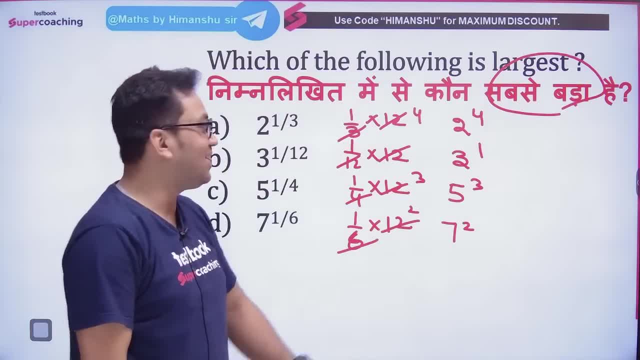 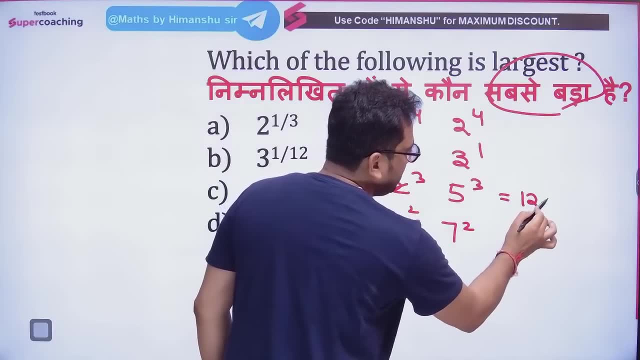 he is saying the biggest. now, see, you will know the difference as soon as you see. yes, this is the difference, but see which is the biggest. so see, the value of 5 is 3, it will be 125,. 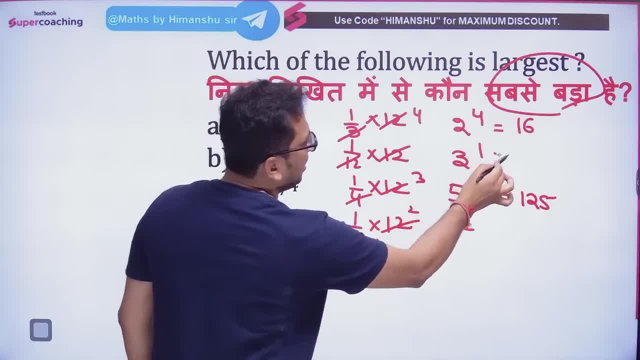 the power of 2 is 4, 2 times 4 is 8 times 16,. the value of 3 is 1 is 3, and the value of 7 is 2 means 7 times 7 is 49,. 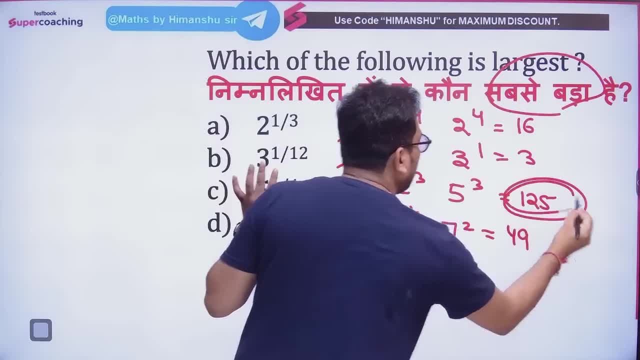 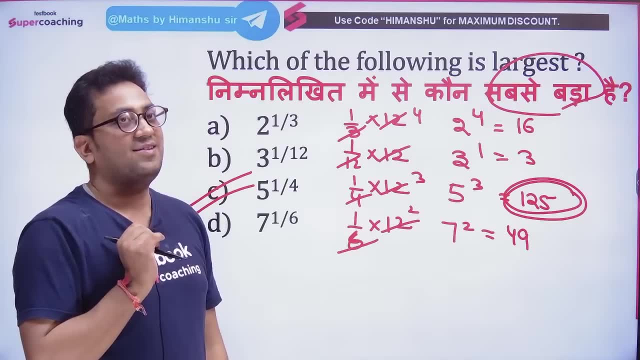 so you will clearly see that, yes, this is the big one. this is the big one. that means the option C will be answered. son, there is no A, there is no B, there is no D. the option is C. what is the option? it is C. 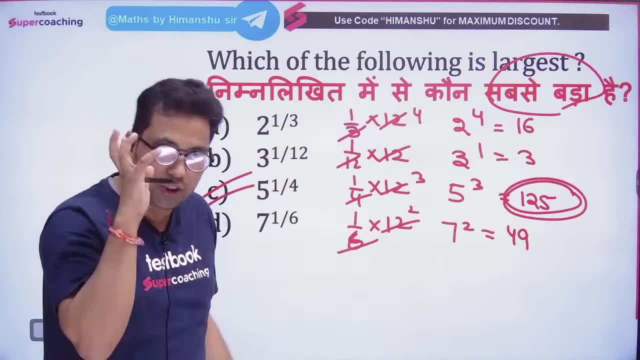 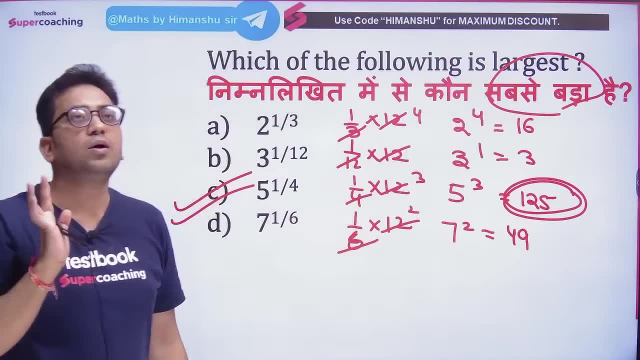 you have missed the small one. you had to miss the big one. read the question carefully. what is the question? if the big one says, then catch the big one. if the small one says, then catch the small one, why are you making a mistake, son? why are you making a mistake? 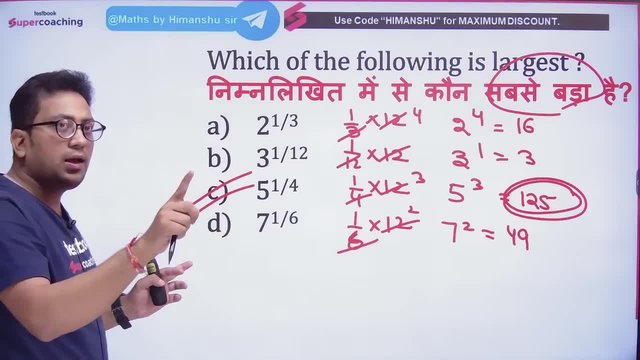 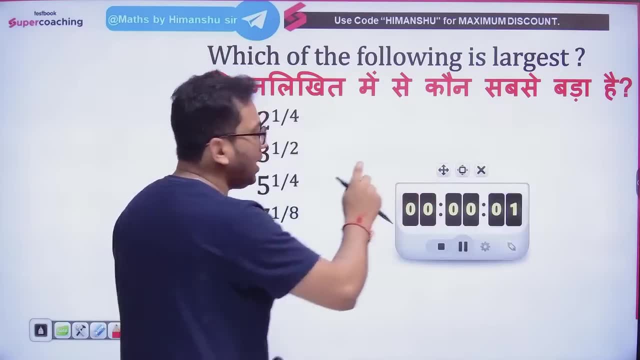 you don't do it like this, right? if you understand, then you have to do it right. okay, C is very good. let's move on to the next question. next question: let's see how many children are shining. what did I say? don't be afraid to take the LCM. 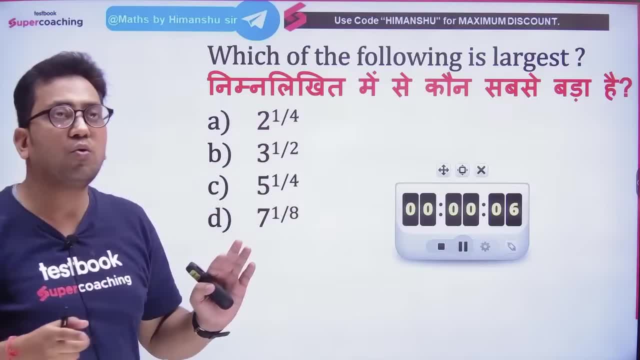 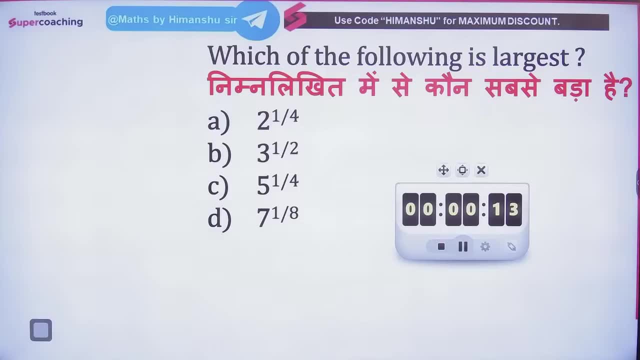 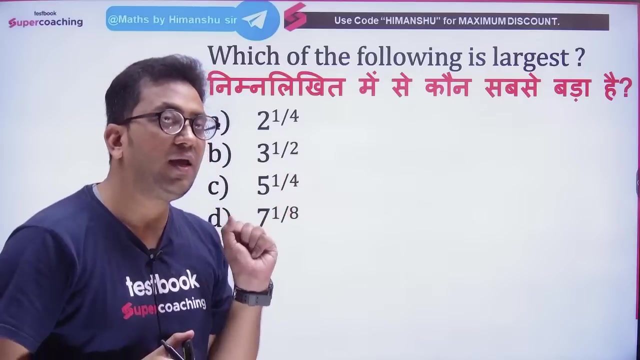 open your mouth and mark the LCM. look at the big number. read its page quickly. tell me what the answer will be. take it quickly posted. come on six seconds over. answer me quickly. I want the right answer at all costs. don't get it wrong. 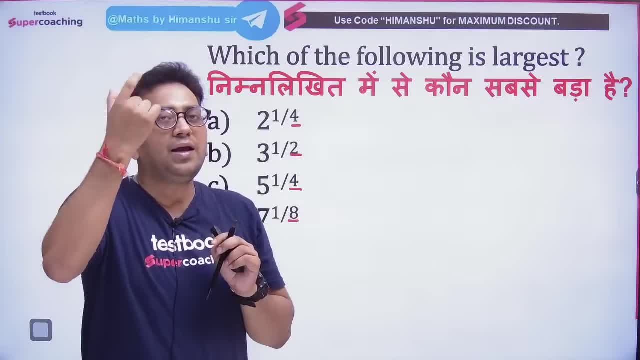 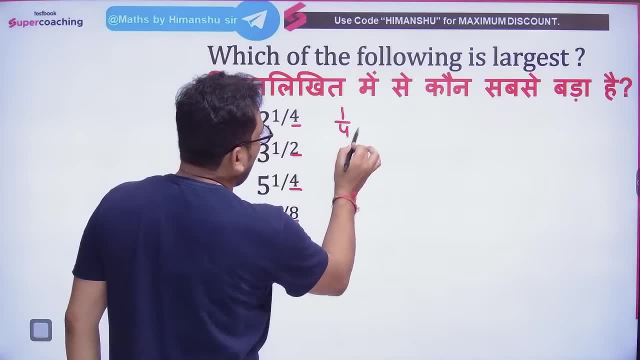 must raise the grand. must raise the grand. tell me quickly, must raise the grand. you see, four, two, four, eight. google the number 8, read the page năm 8,. So 1 divided by 4 is equal to 8,, 1 divided by 2 is equal to 8,, 1 divided by 4 is equal to 8, and 1 divided by 8 is equal to 8.. 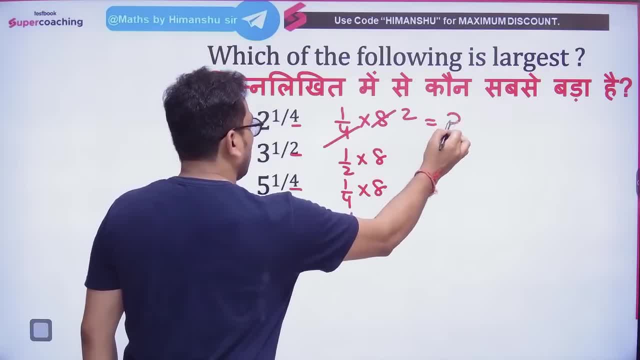 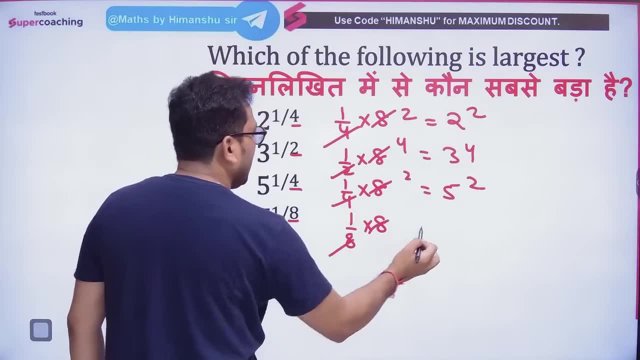 And just start cutting. 4 times 8 is equal to 2,, 2 times 4 is equal to 8,, 4 times 8 is equal to 5, and 8 times 8 is equal to 7.. What we want is a bigger number. We can see the difference between small and big numbers. 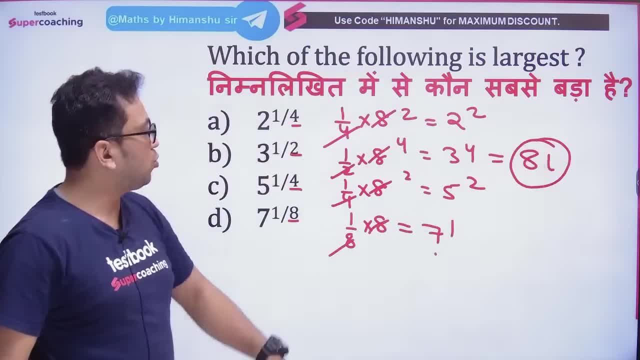 We can see that 3 divided by 4 is equal to 81, because 2 divided by 2 is equal to 4, and 5 divided by 2 is equal to 25.. This means that this is the biggest number, So our solution is also our answer. 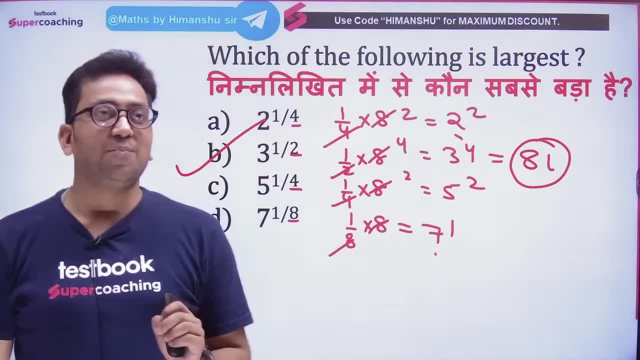 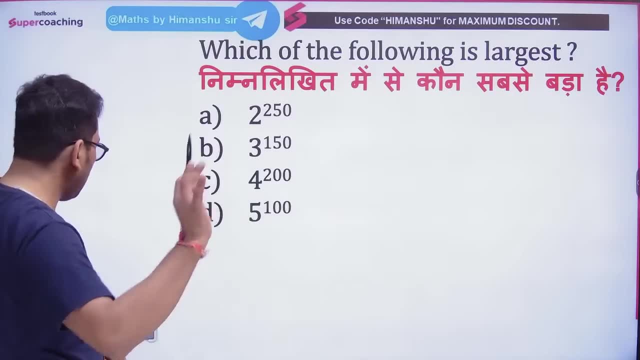 Hey, tell me, did everyone get it? Everyone is shouting B, B, B, B. Very good, It is fun. Everyone is understanding this thing. That means everyone's answer is correct. Now look at this. So far we have seen that we have been given such questions. 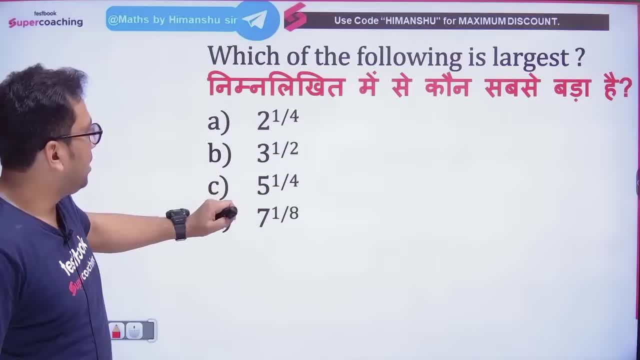 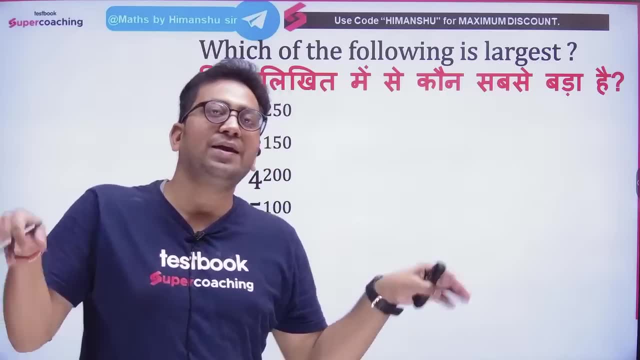 But here the question is given in this way. That means understand. he is saying that I gave you power above, you don't have to look down. You were getting worried, weren't you? You were looking down, then you were taking LCM. 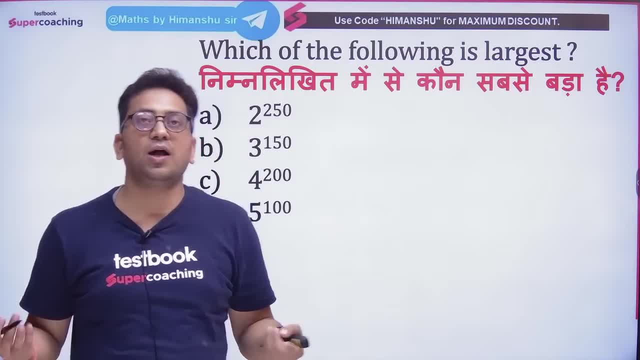 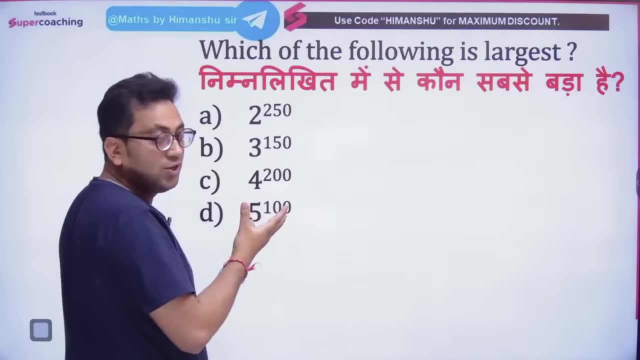 Don't look down, don't take LCM. I gave you power above solve it. The child gets scared to see. He says that 2 divided by 2.5 is equal to 200, 3 divided by 3 is equal to 150, 4 divided by 4 is equal to 200, 5 divided by 3 is equal to 100. 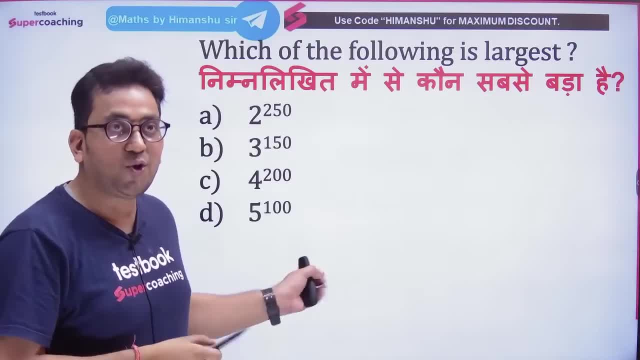 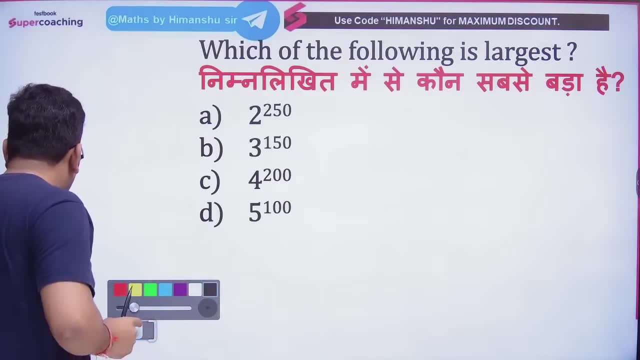 Sir, it is better to solve this. I will leave it, But you don't have to leave it, You have to hold it. Look, son, how to answer such questions. Tell me one thing: When someone troubles you, what do you do? 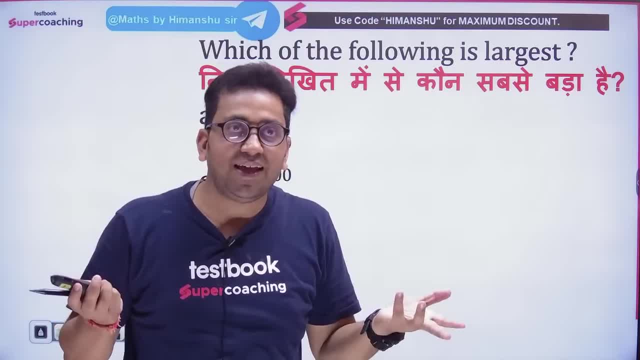 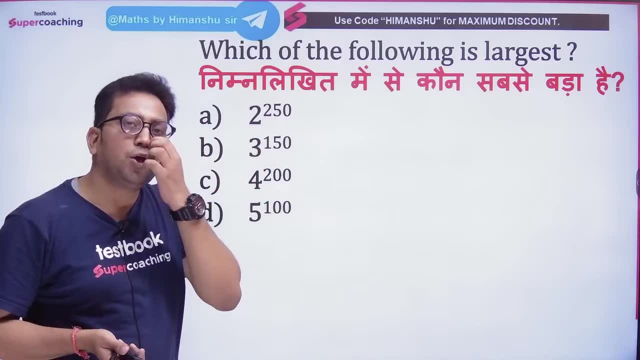 Do you throw it out by taking it out? That's what happens. Isn't it Push? isn't it Remove it? remove it. You do it outside. You also have to do the same here. The one who is troubling you throw him out. 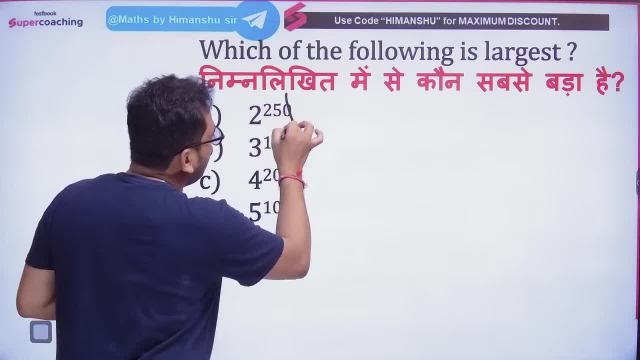 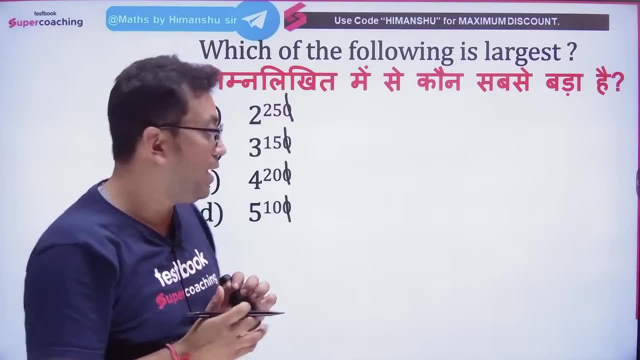 Take him out. See how. What do you do See: zero, zero, zero, zero. Cut all zeros. You have divided everyone, But the condition is that you have to divide everyone by the same number, Like I have divided everyone by 10 here. 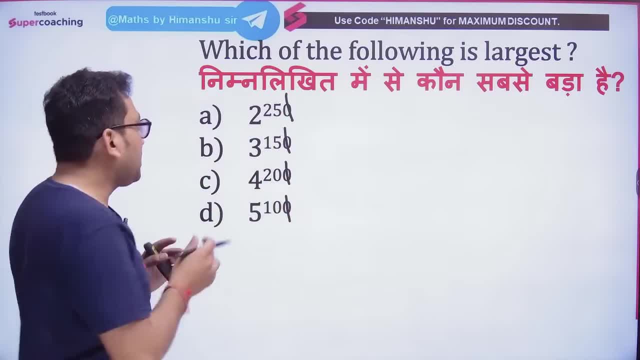 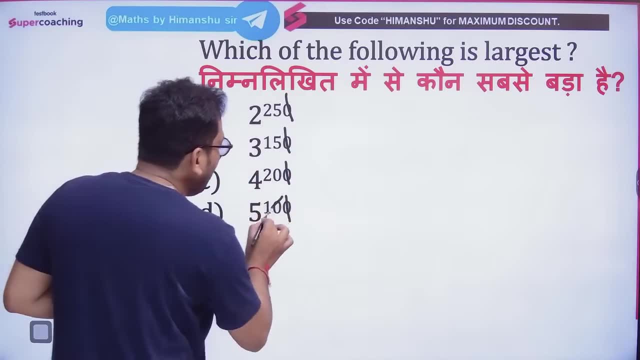 That's why one zero is cut. Now what is left? 25,, 15,, 20,, 10.. Tell me which number comes in the mountain, In the mountain of 5.. Then cut it 5 times 10,, 5 times 24,, 5 times 15,, 5 times 25.. 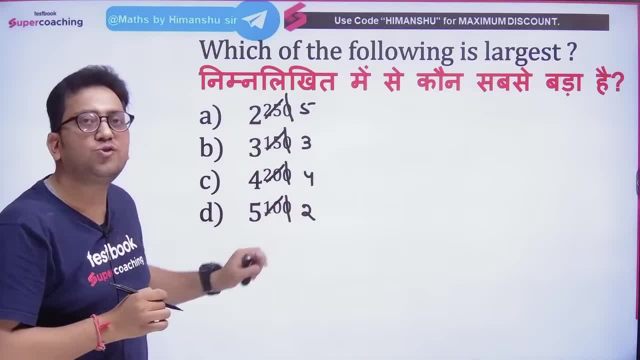 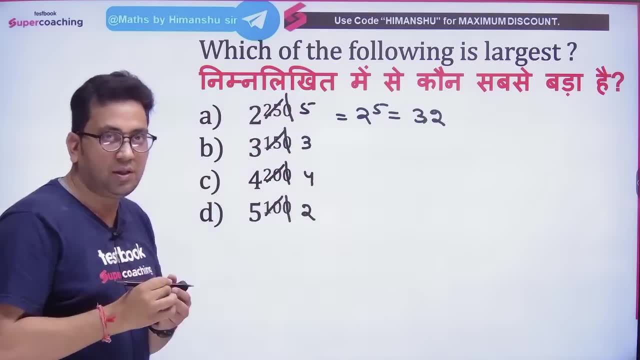 You were troubling me, didn't you? You have done it. Now tell me, can't you solve the problem of 2 times 5?? You will say 2 times 4 times 8 times 16 times 32.. 2 times 5 means 2 times 4 times 8 times 16 times 32.. 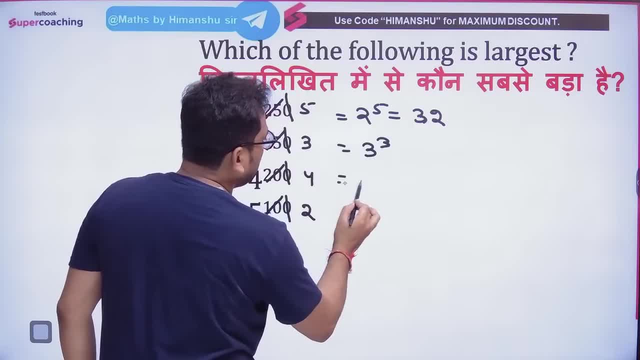 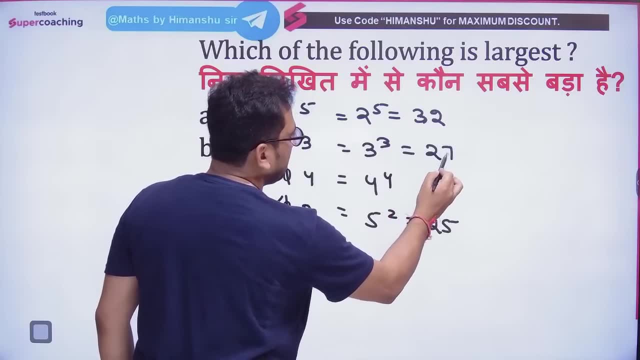 Do you understand, son? 3 times 3 comes. Similarly, 4 times 4 comes here. 5 times 2 comes here. So 5 times 2 means 25.. 3 times 3 means 27.. And 4 times 4 will be very big. 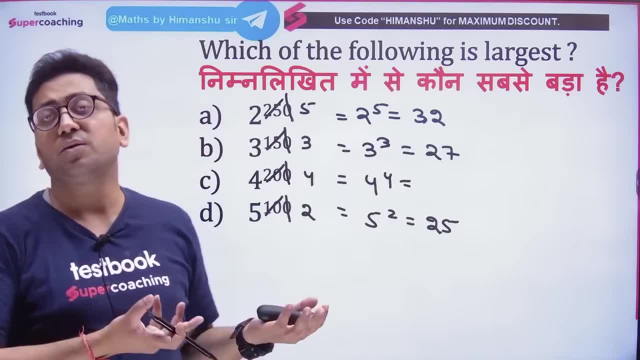 Here too, you will touch it and see that it is the biggest. It will be 256.. 4 times 4 is 4.. 4 times 4 is 16.. 4 times 4 is 64.. 4 times 4 is 256.. 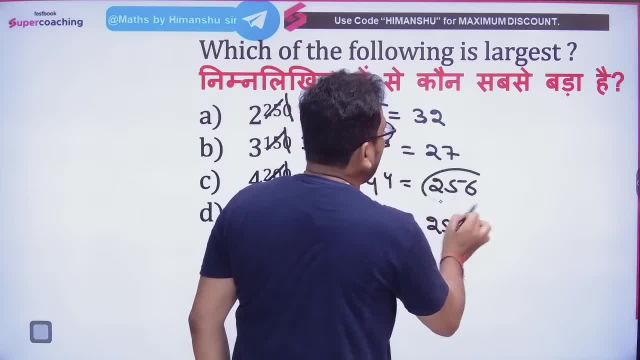 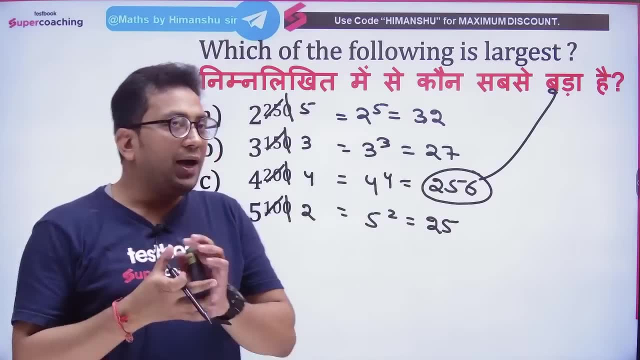 It is very big, sir, It is very big. They will not get it. They will not get it. It is very big. So option C will be our correct answer. So if you give the numbers above in the mountain and give very big numbers, 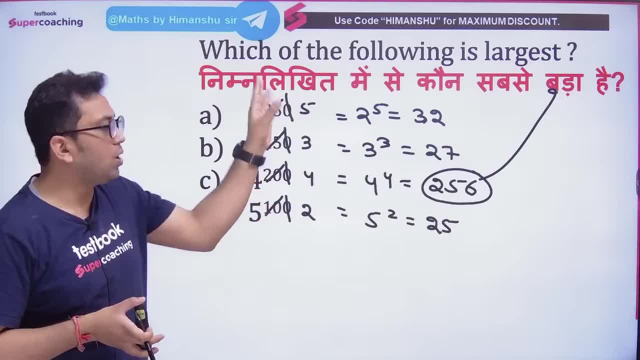 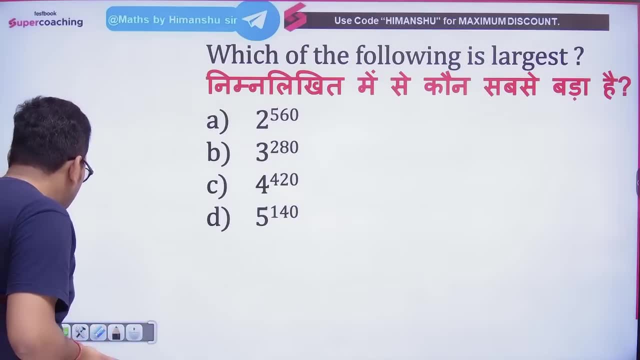 then take only one way, that I have to cut them all and make them smaller. It is very troubling. So you will make it small, right? You will do it like this. Next question, son. Next question: Tell me quickly what will be the answer. 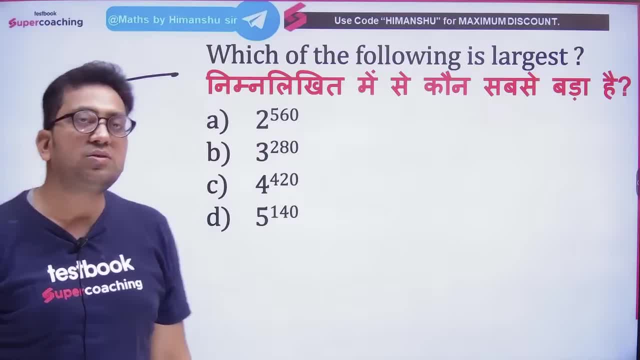 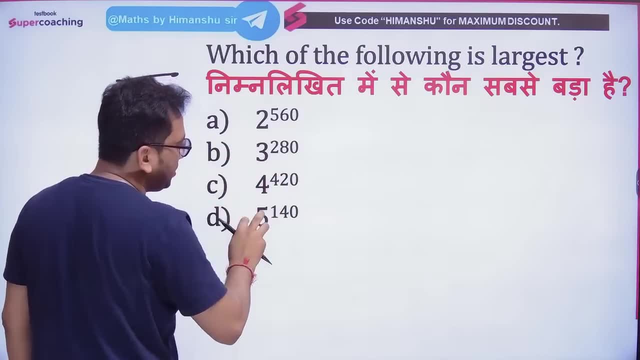 Answer with speed Which one is the biggest among the numbers? Answer quickly: 2 times 5 is 560.. 3 times 2 is 280.. 4 times 4 is 420.. Or 5 times 5 is 140.. 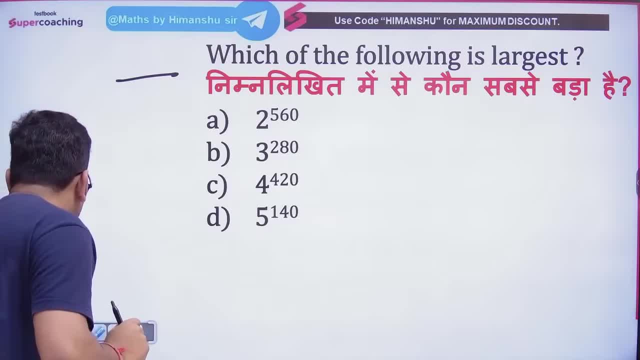 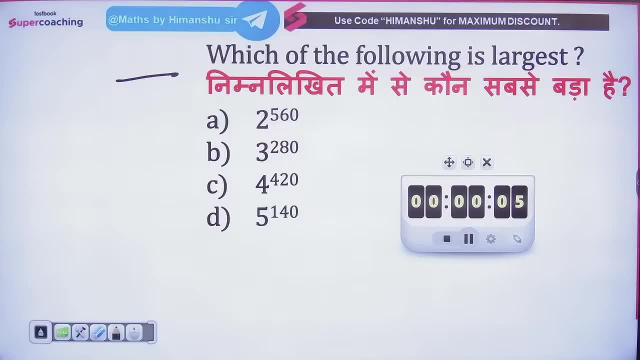 Fly quickly. Come on, let's give you time. Take it Time of 30 seconds for all of you Fly. Tell me what will be the answer. Come on, 1-2.. Which one is the next question? 1-2.. 5-6.. 4-6.. 5-7.. 3-8. 3-6. 5-7. 1-2. 3-6. 1-2. 5-7. 3-6.. 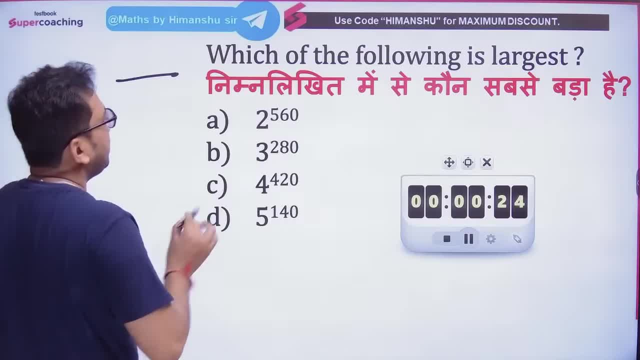 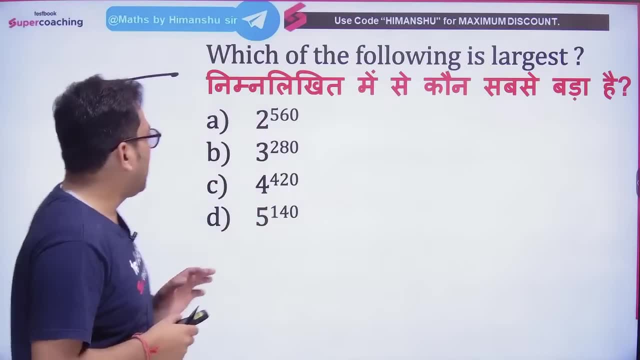 5-8.. 3-6.. 4-6. 5-7.. 1-2. 3-6. 5-7.. 3-7.. 5-7.. 1-2. 5-7.. 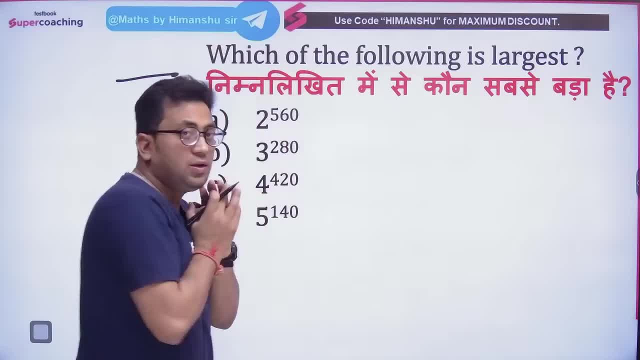 1-2.. 5-7.. 5-7.. 5-7.. If you think it is increasing, then reduce it, Reduce the power. You will say 0, 0,, 0, 0, cut it. 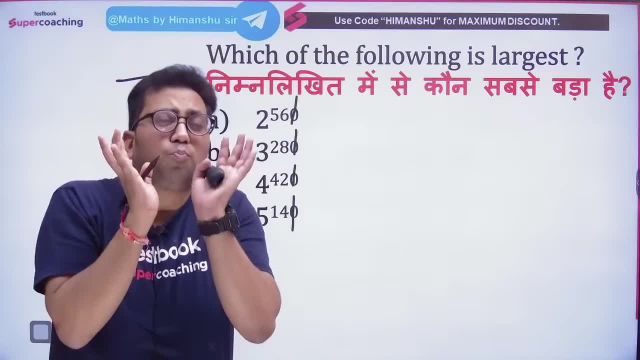 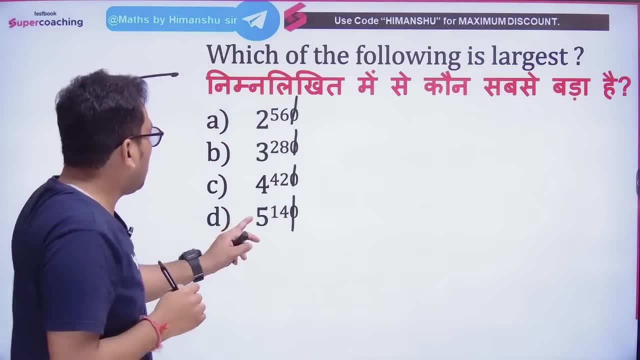 Now the mountains. at least, at least I am saying at least, at least, at least you should remember- till 25.. If you think 25 is too much, then do it till 20.. So see, you all know the mountain of 14.. 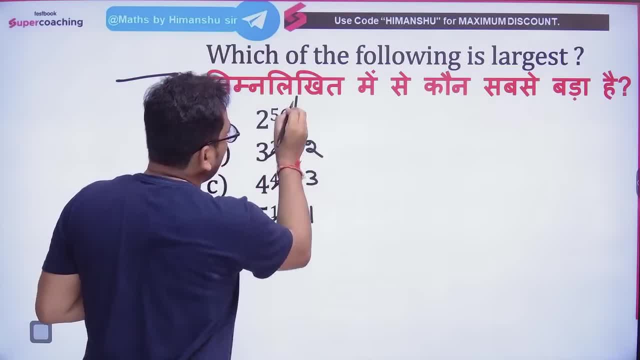 14 is less 14,, 14,, 32,, 42,, 14,, the world is 28, and 14 is square 56. If it comes from 14,, then you will cut it straight. Otherwise, first you will cut it from 2, then from 7.. 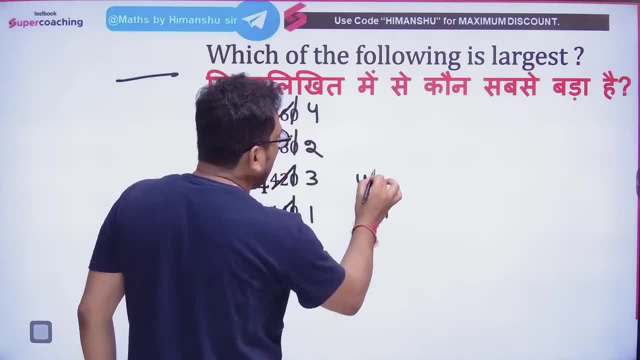 So you will say 5 to the power of 1 came, 4 to the power of 3 came, 3 to the power of 2 came, 2 to the power of 4 came. What did the big guy ask? 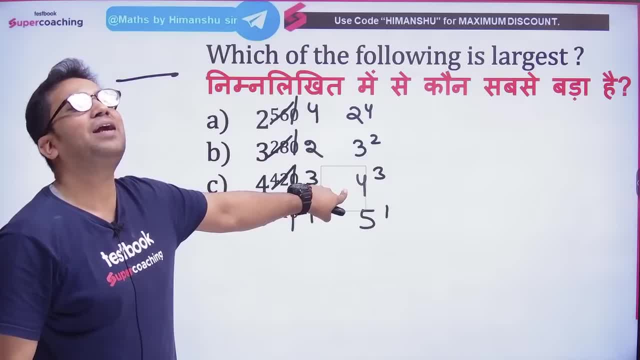 Now the big guy. as soon as he saw, he said: here, I have caught it. I have caught it. 4 to the power of 3, I have caught it. that means this is 64.. 4,, 16,, 64,. the rest will come less right. 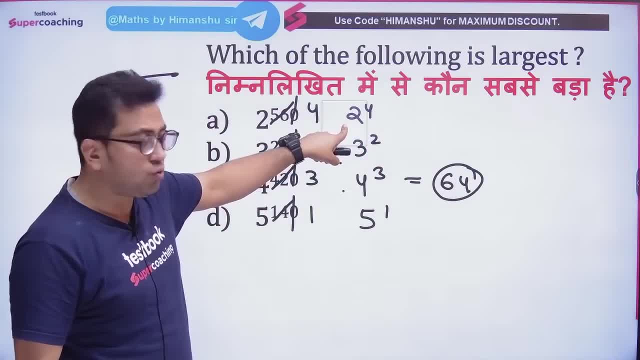 3 to the power of 2, 3,, 3, 9 will come, 2 to the power of 4, 16 will come And 5 to the power of 5, 5 will come. Then our answer will be C. 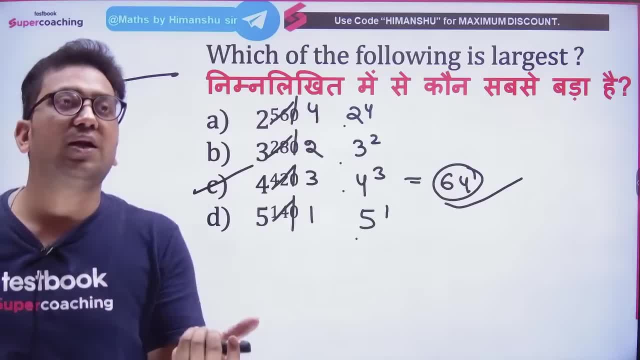 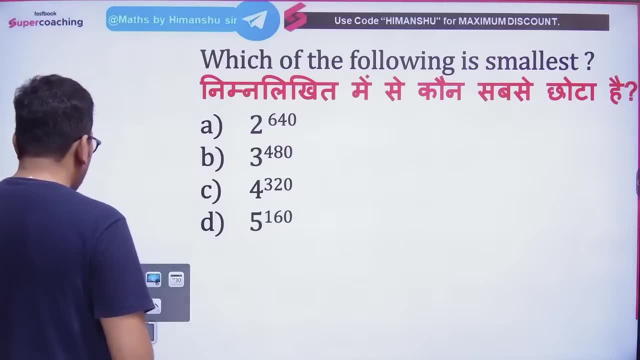 That means C will be our answer. 4 to the power of 3, that means C will be our answer. Very good, Let's move on to the next question. Next question: do it carefully. Let's give you 30 seconds. 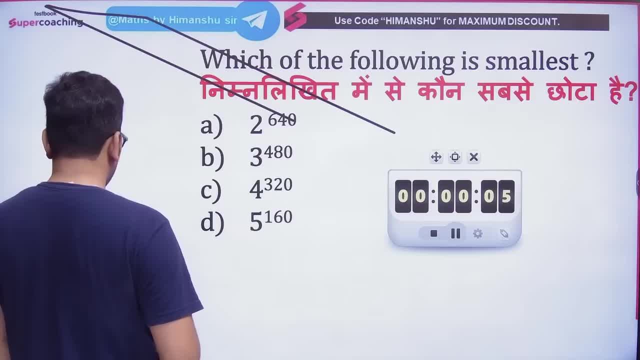 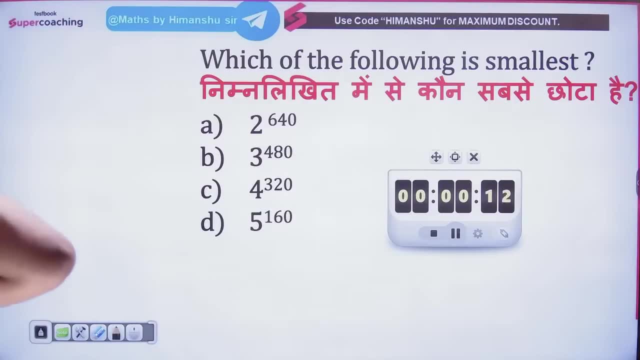 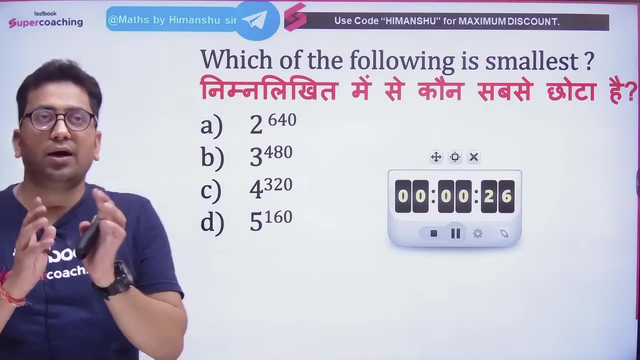 Tell me what the answer will be. Come on, answer me. Tell me what the answer will be. Tell me All of you. answer me 8 seconds. Every child is watching the session. every child's answer is correct. The child who finds the math difficult. 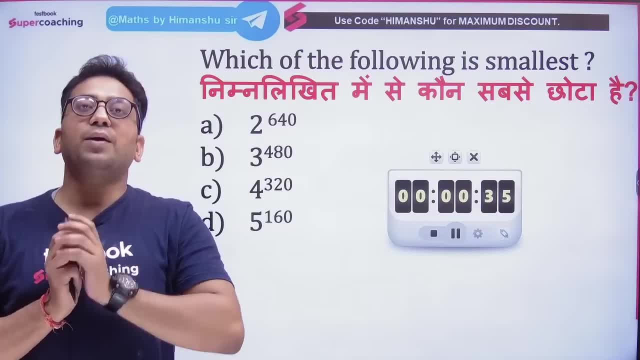 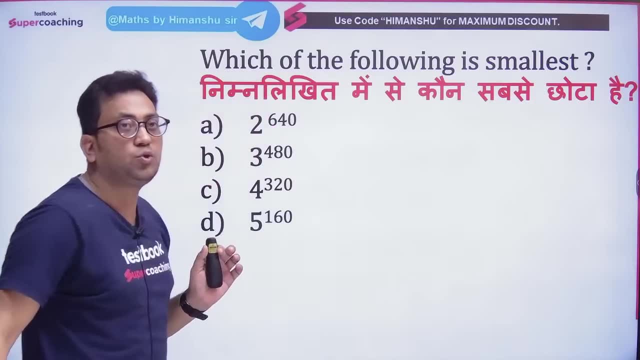 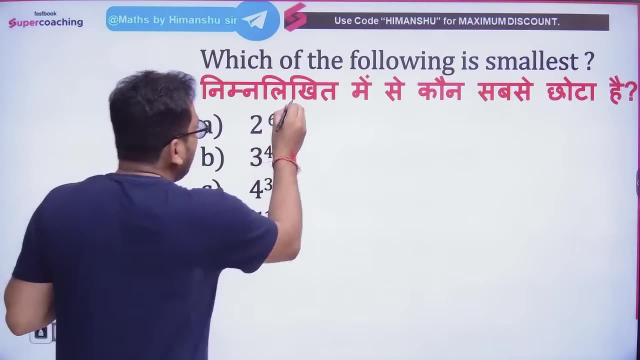 I say: come at 12 and join. I will change your thought. I will change your thought. Okay, Very good, The time is up. The children are going towards option D. If it is correct, then my hard work will be successful. 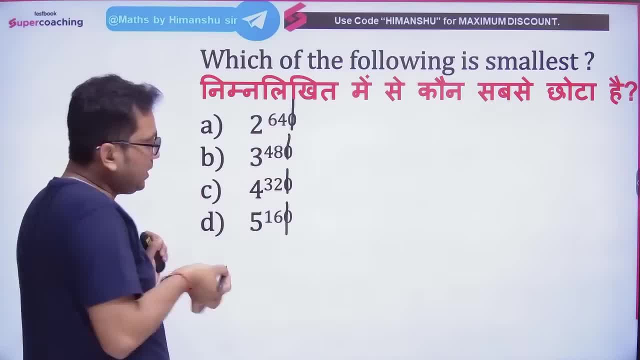 I have got 0 0, 0. Now all these will be deducted from 16. I hope you can see 16 1 x 16, 16 2 is 32, 16 3 is 48, 16 4 is 64. 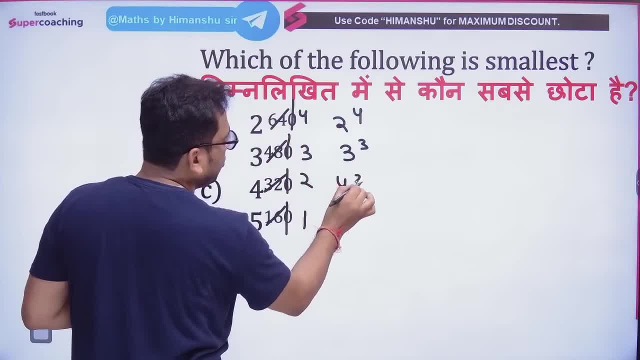 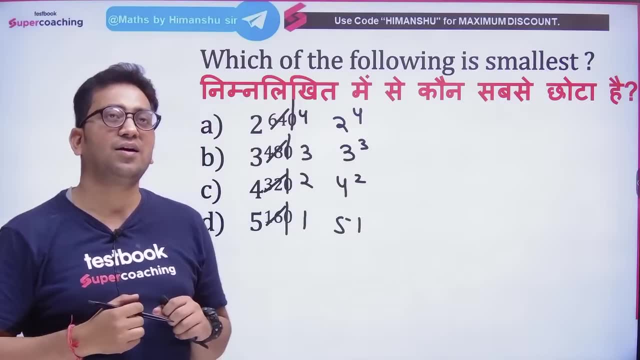 Sir, 2 x 2 is 4, 3 x 3 is 3, 4 x 2 is 2, 5 x 4 is 5. Oh, great, You have guessed. amazing From where AB got Right answer was coming. Oh, we are asking for a small number. 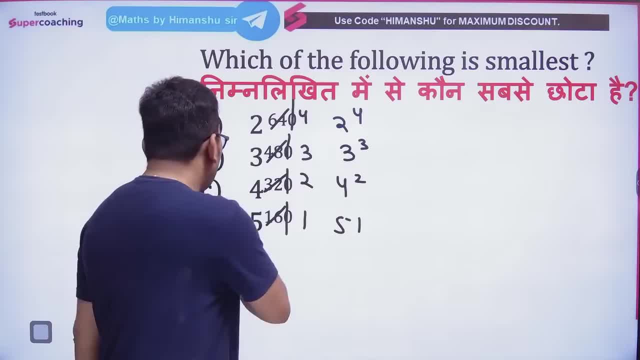 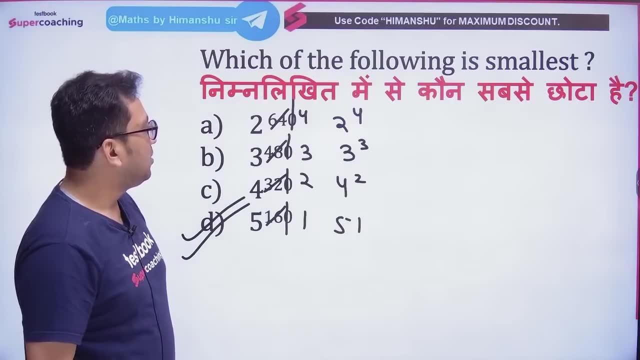 Will understand in a moment. 5 x 4 is the smallest number. Do we need to think? Yes, D answer should be coming right. Where did the B come from? Don't do this, Read it. What have you asked? Chutka, Chutka, Chutka. 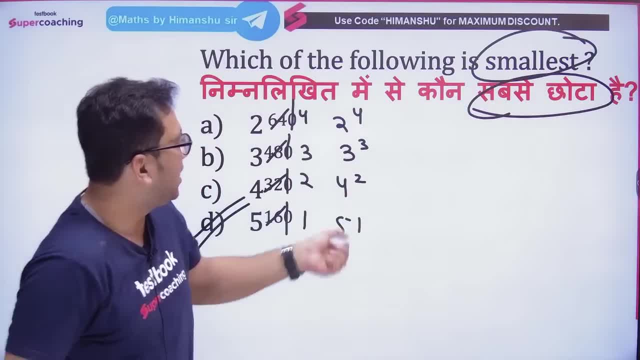 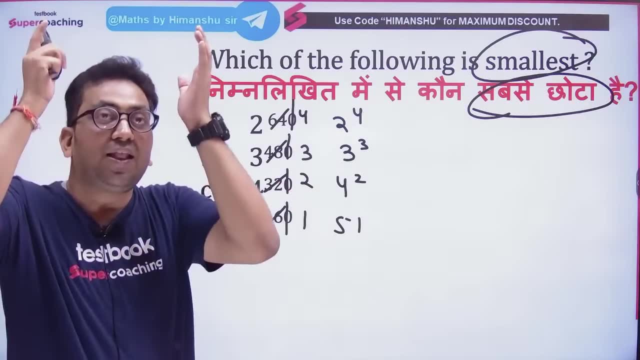 Wherever the elder asks you hold the head of the Chutka. Wherever the Chutka asks you hold the head of the elder Brother. see what you have asked Chutka has asked. It is written as big, smallest. 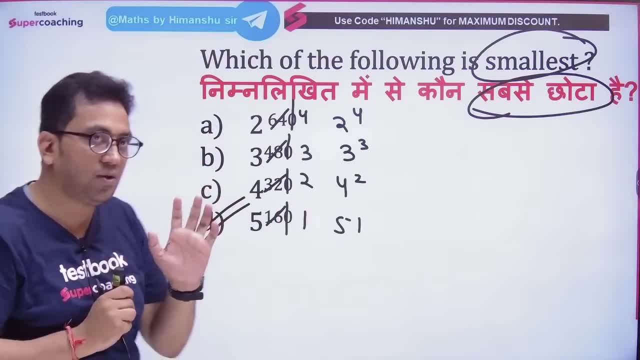 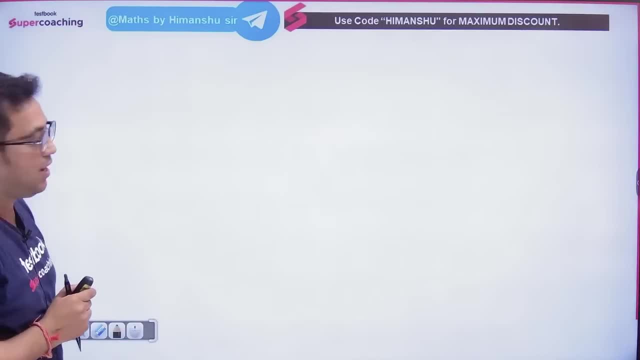 Still, you are saying big, big and D will be our answer. Absolutely, The answer of the children who are answering D is correct. Next question: Let's see, brother. the next question is: The next question is No, brother. the next one is a mess. 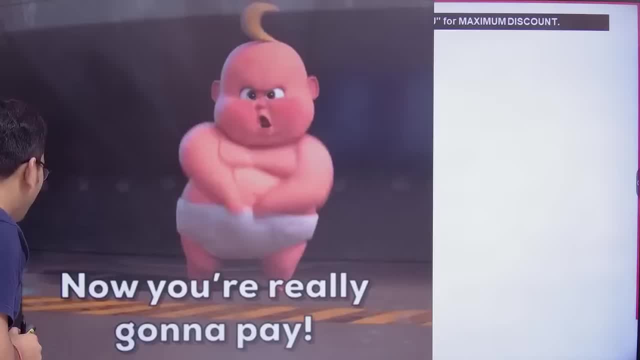 Hey, hey, hey, hey, see who has come, See who has come, son, who has come, See, see what he is saying. Huh, who has come? This is Zoravar. Do you know his name? 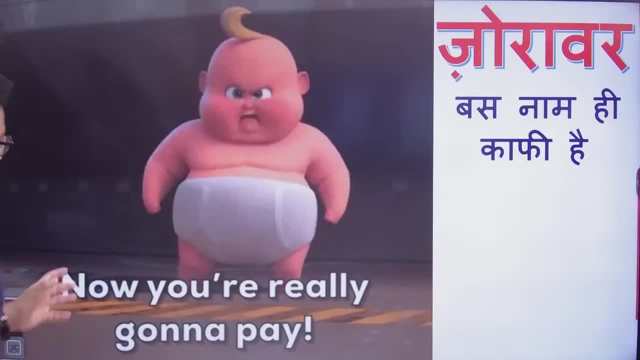 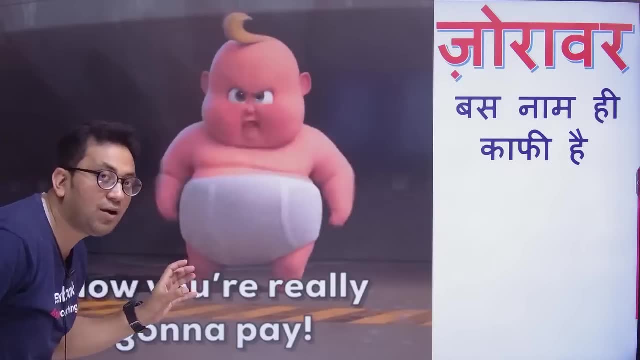 Zoravar. Just the name is enough. This one who showed you the cruel right. This is his third child, Isn't it? This is his third child, son of the cruel. This is Zoravar. Now see the cruelty of Zoravar. 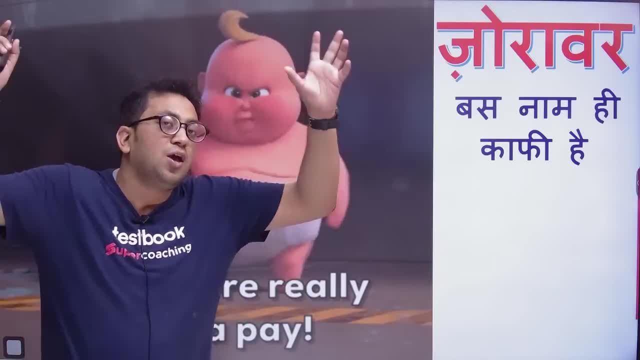 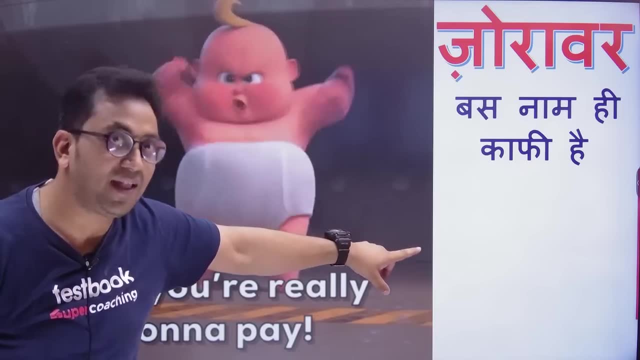 See how you have brought the question for all of you. He has brought a very amazing question. He is angry. He has become red. Now let's make his questions red. Come son, Come Zoravar, We will make his questions red. 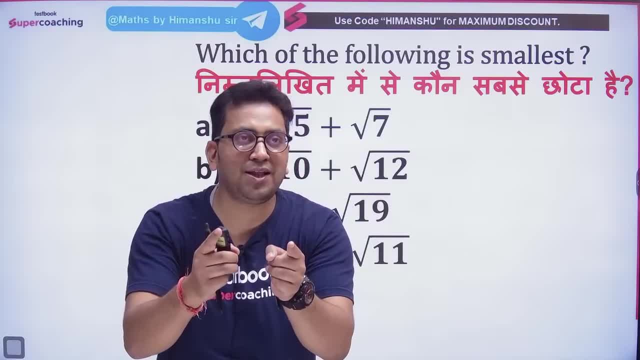 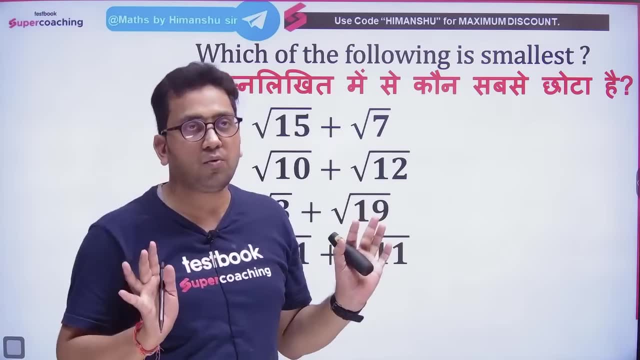 Huh, Be ready. My red, my yellow, my blue, Be ready. Now see how we will make this question red. First I will explain you the concept And then I will tell you how to shine. Okay, So first of all, be ready to understand the concept. 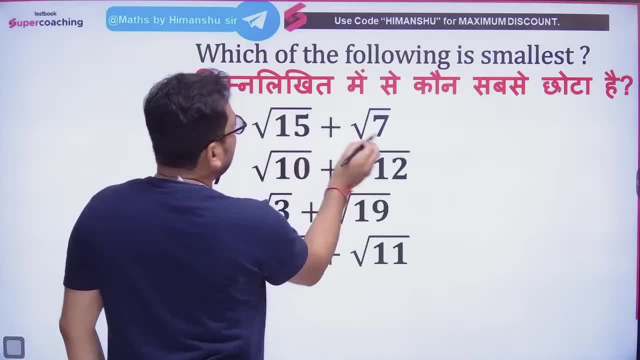 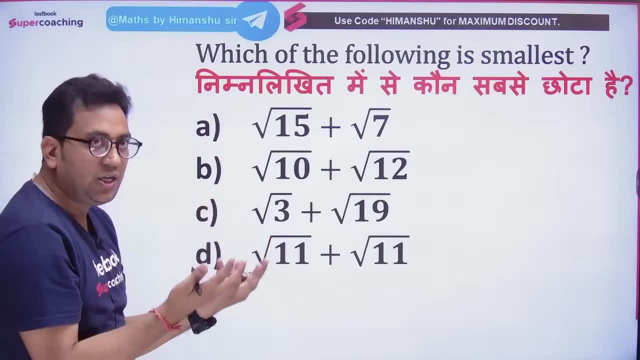 Have patience. Have some patience Come Zoravar. This is the question He is asking you tell me which one is the smallest among these. See the way to do this: the tradition, the traditional approach, the conventional approach. what is that? 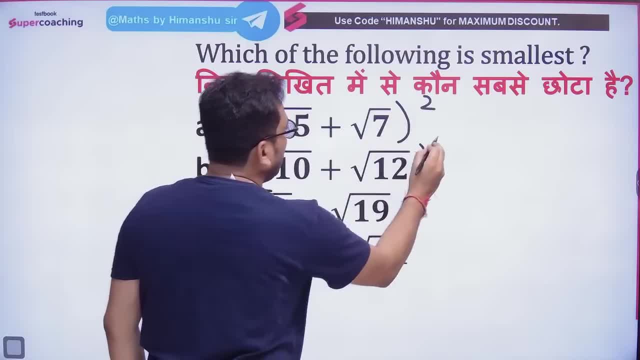 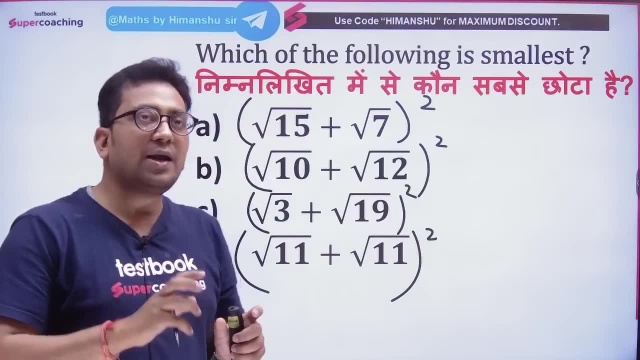 That you make everyone's whole square. That is here also, here also, here also and here also. Why do you make the whole square? Because this group is troubling. So if it is troubling, then the root will be removed when you make the square. 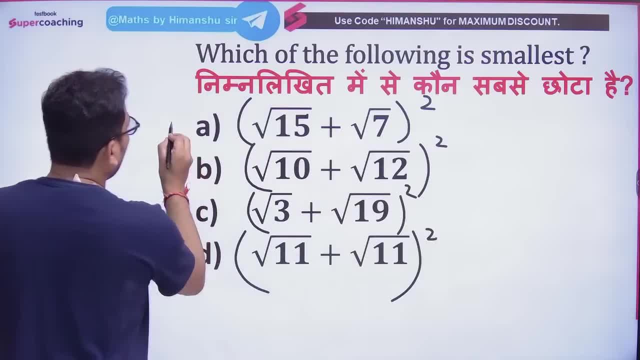 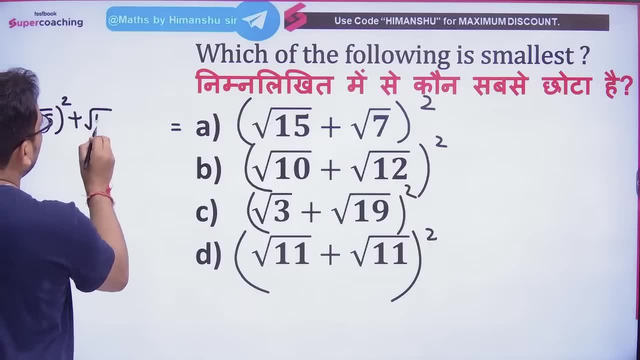 Make the whole square. Now see what is the whole square of a plus b a square plus b square plus 2ab. That is the child. Our here does root 15 square plus root 17 square. Okay, In the same way, plus 2 into root 15 times root 17.. 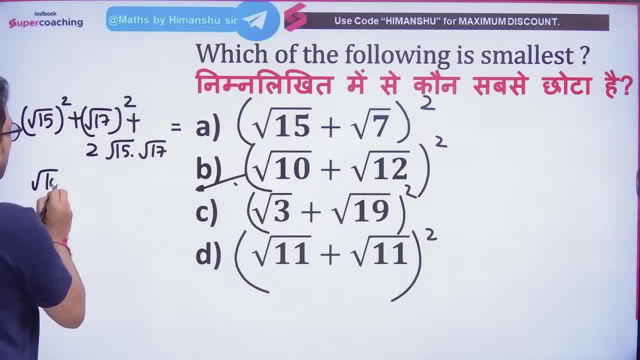 In the same way. he will write it in the same way That root 10 square. Now just understand. I will tell you how to shine. You will remove this question in 1 to 2 seconds. But now understand. Plus 2 times root, 10 times root, 12.. 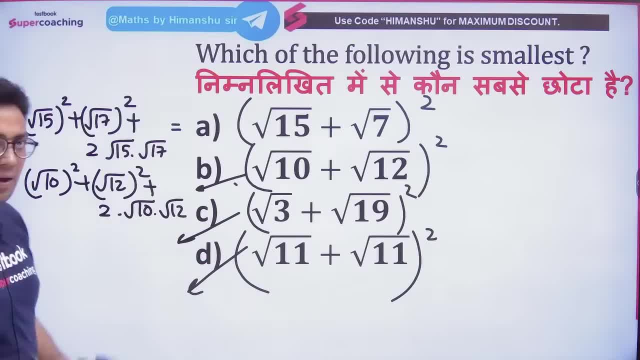 In the same way. the child will do it with c. In the same way he will do it with d. I am not doing it, Just understand it. This will come to you, Isn't it? Then the child has to solve this whole. 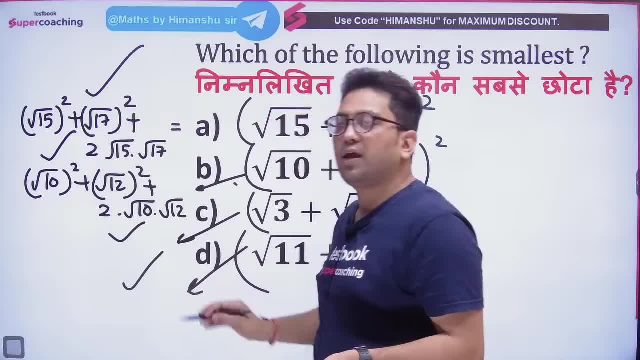 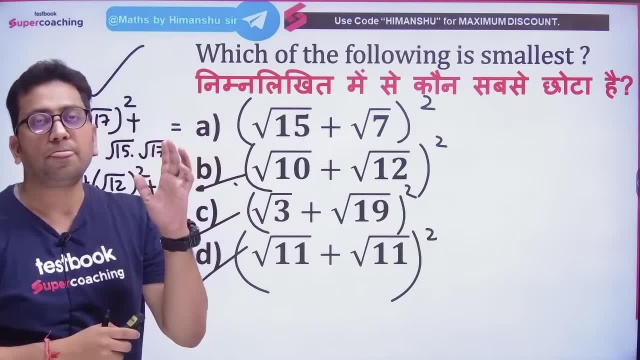 This also has to be solved. He will solve c too, Then he will solve d, And then he will see who is the smallest among them, The one whose smallest value will come. he will tick that square, But if you do this, then the exam will be at night. 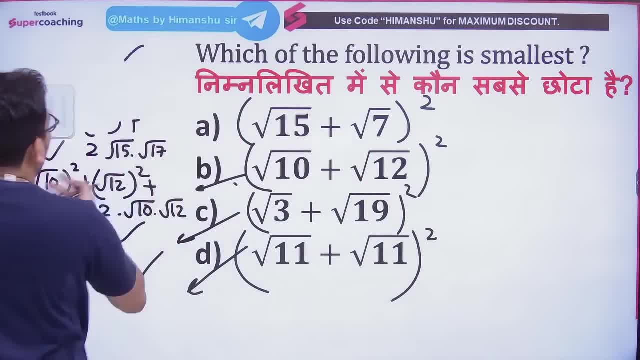 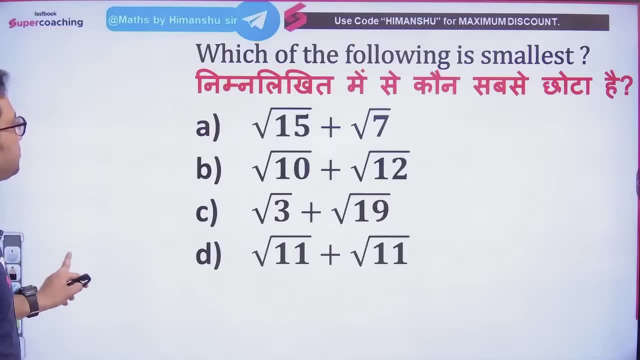 The exam has to be given in the day, Isn't it? So you will not do this. What will you do? You will shine, son. What will you do? You will shine, my dear. You will shine, Absolutely, Okay. 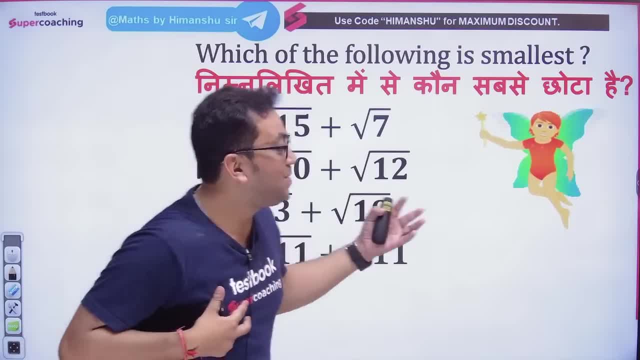 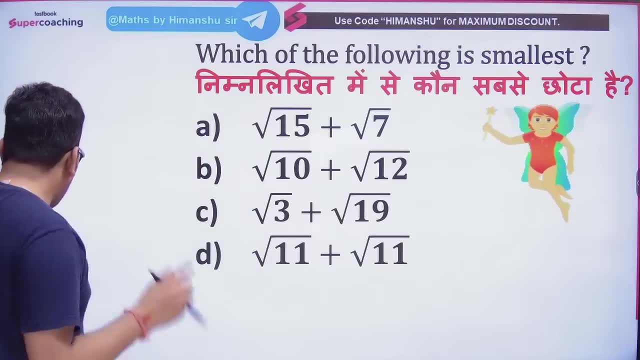 And who will come to shine? Oh, not us. Papa's friend will come. Papa's friend, He will shine, He will tell us how to shine. So come a little. You just have to see, son, that their Yogfal is how much it is coming. 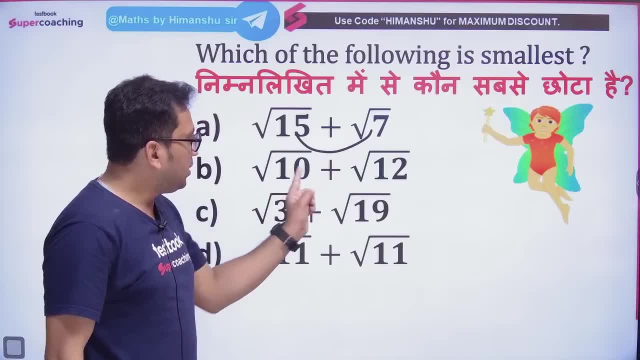 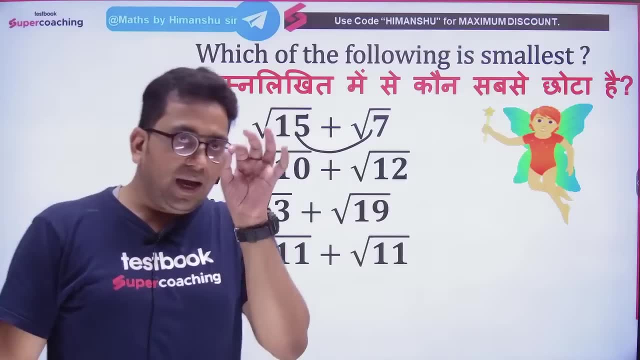 It is coming here equally: 15,, 7,, 22.. 10,, 12,, 22.. 19 and 3,, 22.. 11 and 11, 22.. Yogfal is equal. And if Yogfal is equal, then only. 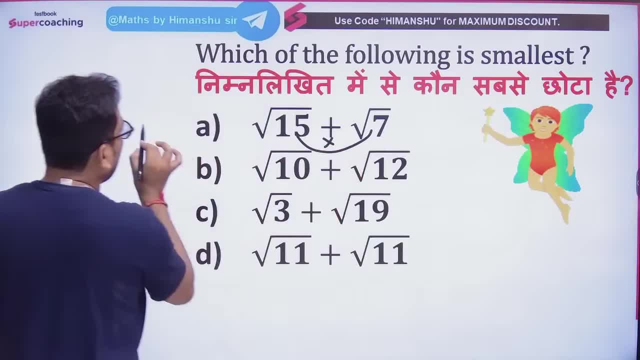 So you have to see by doing the math that how much is 15, 7, 105.. How much will you do with 10 and 12, 120.. How much will you do with 19 and 3, 57.? 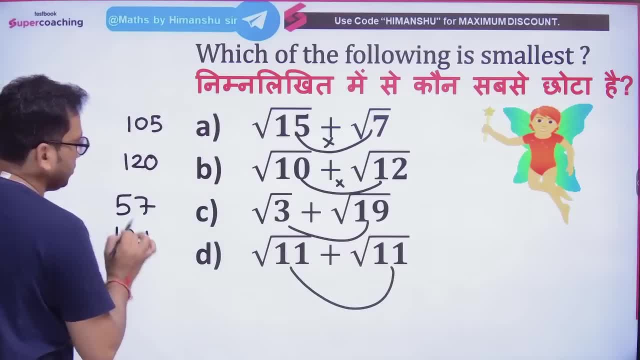 And if you do the math with 11 and 11, then 121.. Say yes or no. Now tell me which one is the biggest among these, The smallest one, Which one is the smallest? So you will say 57 is the smallest. 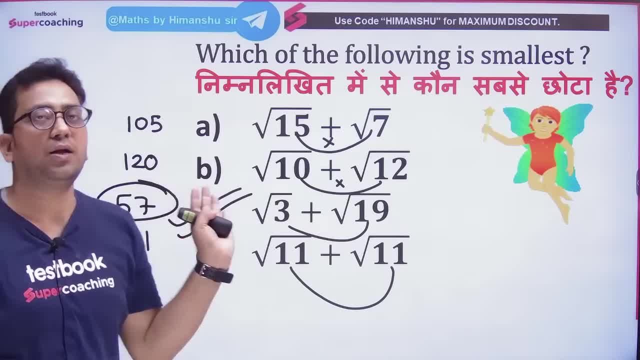 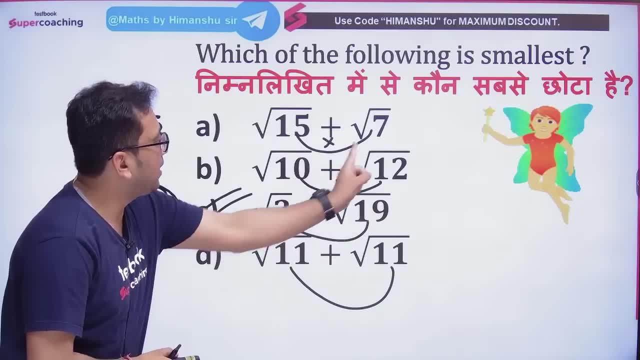 If this is the smallest, then our answer will be C. End of story. Understood My point. That means you don't have to do anything. You just have to do the math and see What to do. Do the math and see. 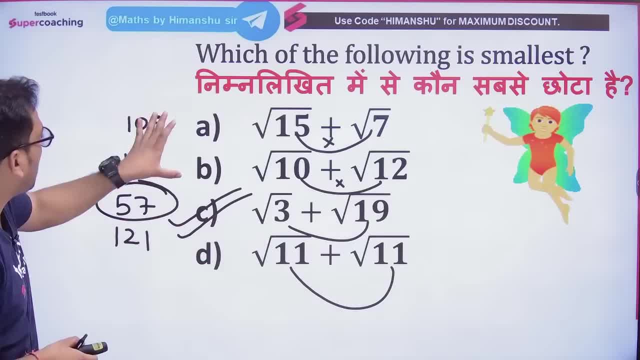 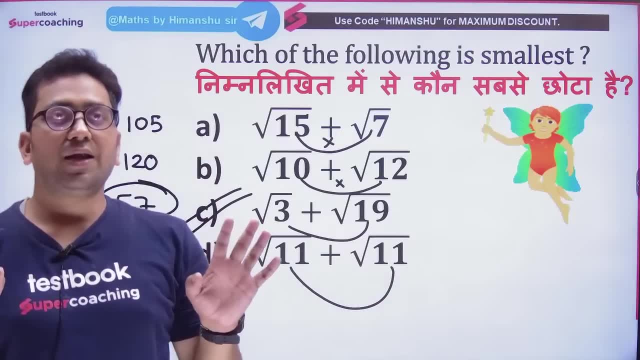 And where the smallest came. that is the smallest Where the biggest came. if the biggest asked, then the biggest of 101 is that is. this is the biggest. Every child got it. Got it Now, sir. if the father's son got it, then we will get it. 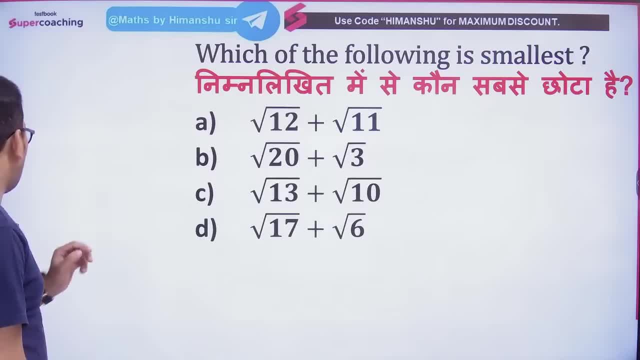 Isn't it? The next question is coming, son. The next question is coming in front of you. Fly quickly, Tell me, let's see how many children are flying the question. We give you time: 20 minutes. There is a time limit of 30 seconds. 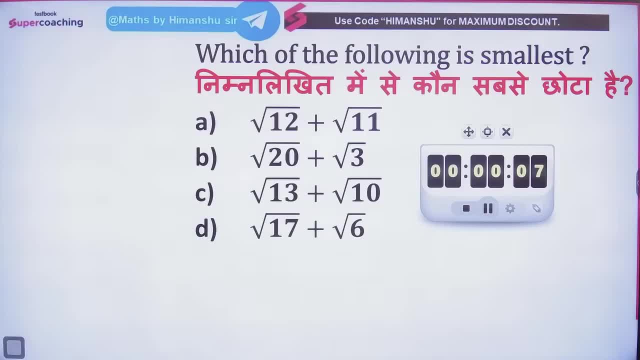 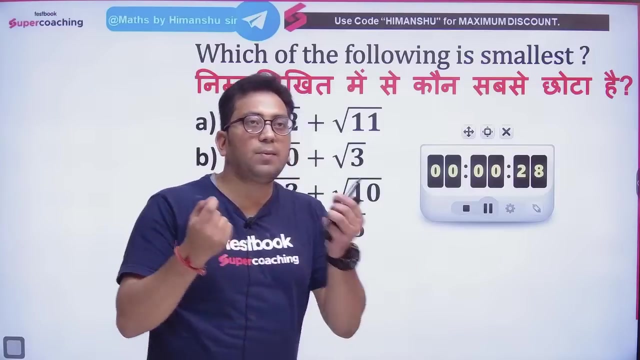 Fly, son, Tell me what the answer will be. All of you, All children. once click on the button of like, I can see that the likes of you people are very less Okay. Like the session, son, It's fun. 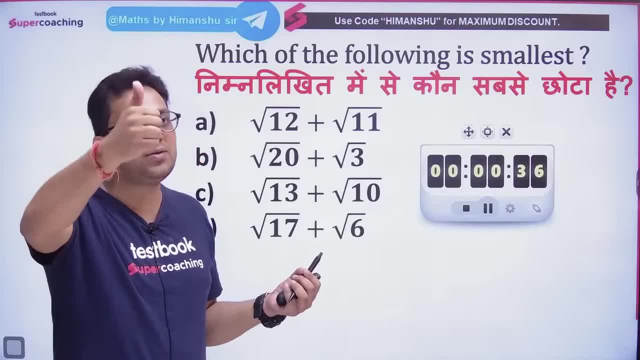 So once, all of you, my lion and lioness- definitely click on the button of like once, Isn't it? All of you? all of you definitely click on the button of like. Okay, then let's move forward and talk about this question. 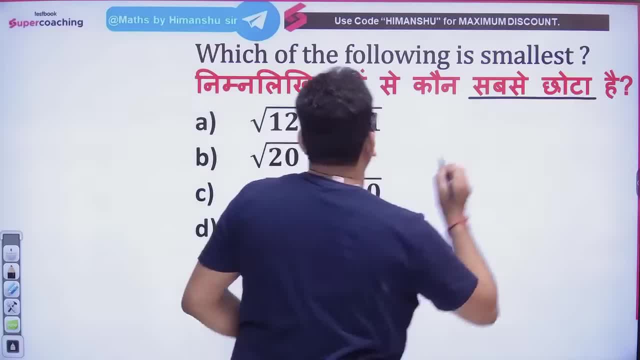 I have asked you the smallest, the smallest, I have asked you son. So what will we do? We will see first That, yes, the Yokeful 23,. here also 23 is coming. here also 23 is coming. here also 23 is coming. 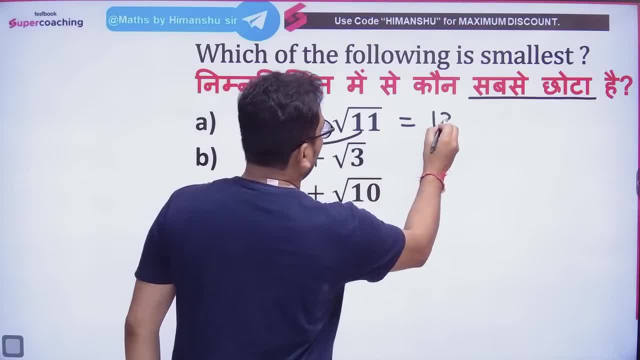 Means you have to do the math. So if the child will do our math, then here it has come, 132.. If the child will do the math of 20, it will do the math of 3,, 20 or 60.. 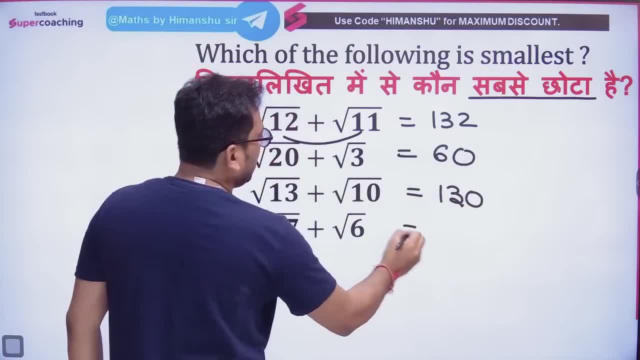 If the child will do the math of 13,, it will do the math of 10,- it has come 130.. And if the child will do the math of 17,, it will do the math of 6, it has come 102.. 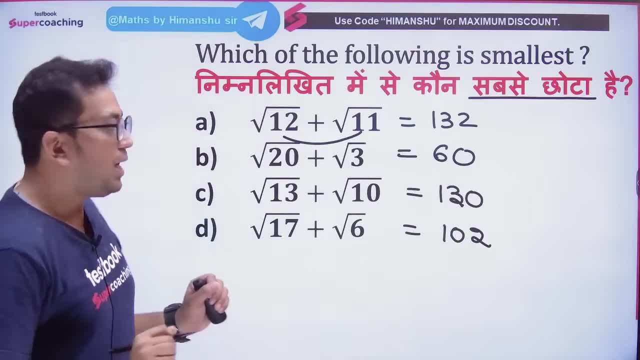 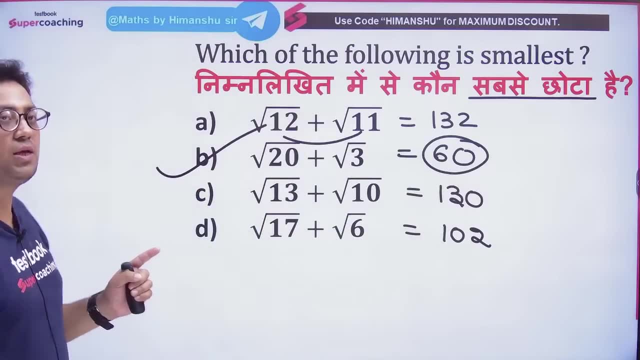 Say yes or no. End of the story. Now you are seeing the smallest, So the smallest is this, sir. So B will be our answer. B is everyone's answer. Very good, B is our absolutely correct answer. 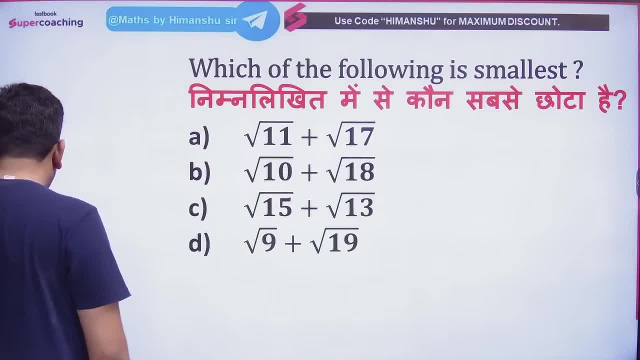 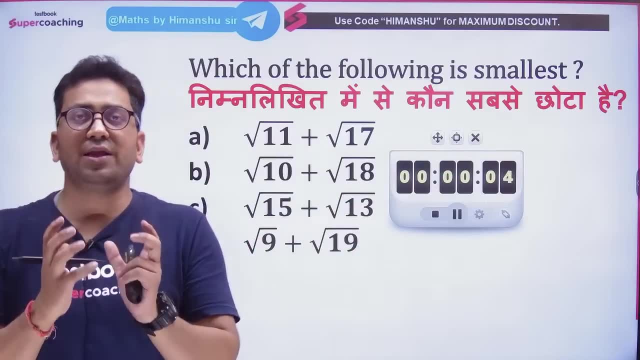 Let's move on to the next question. Next question is coming. Fly the question. Tell me what will be the answer. I will keep on changing the question slowly And today I will solve all your problems. Okay, Quickly Fly the question, son. 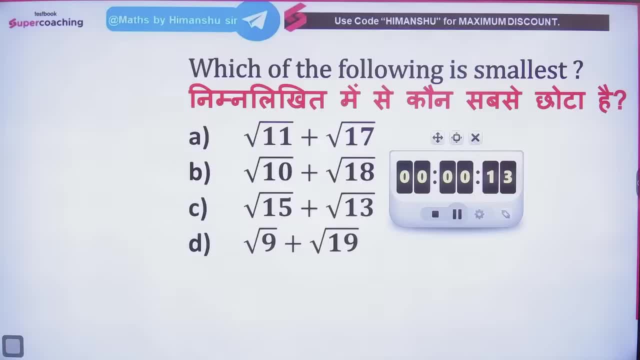 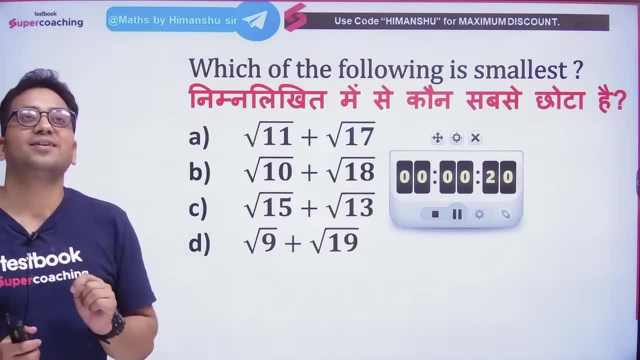 Tell me what will be the answer. Because look, joint quality, part reduction. This is what every child does, But when such questions come in the exam, then they give problems. Now we will not give. Tell me quickly what will be the answer. 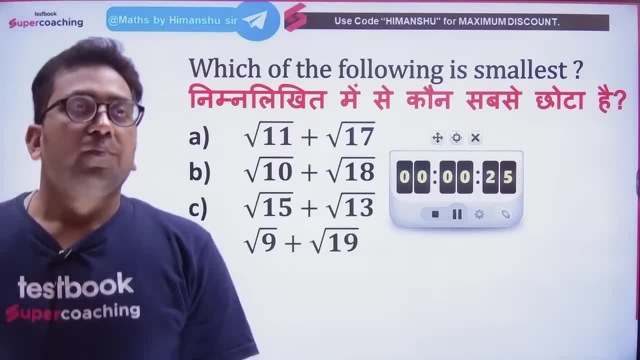 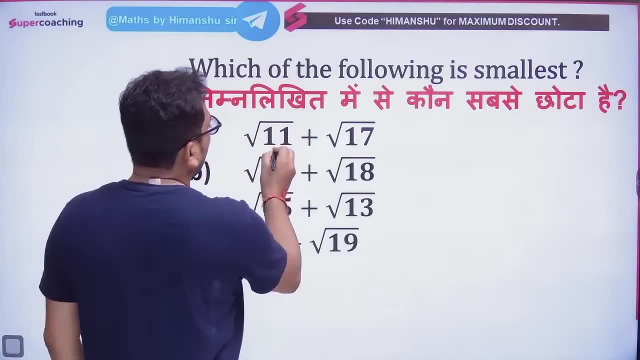 All of you Going towards B here too, Okay, okay. okay, Come a little. Look what will we do. first, Yoke ful. 1 and 7, 8.. 1 and 1, 2.. 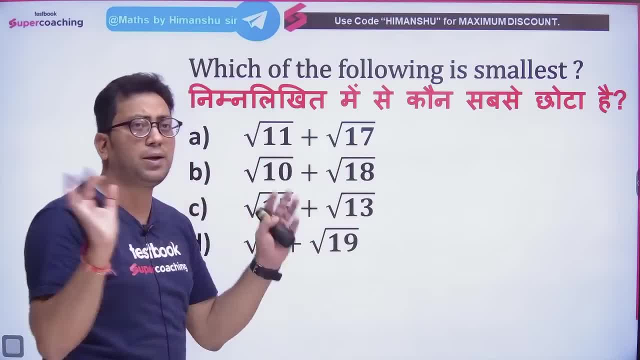 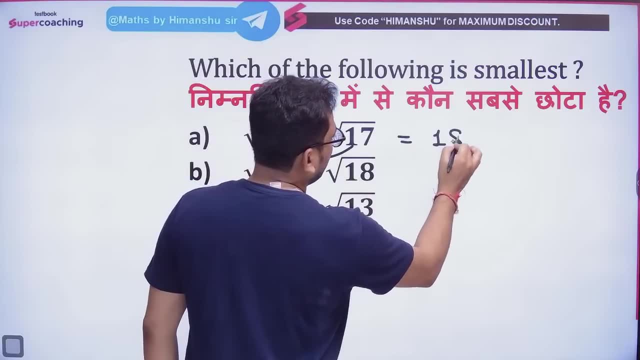 28., 28., 28., 28.. All of them are 28.. All of them are 28.. That means what you have to do now is to multiply. So when you multiply, how much will it come? 187.. 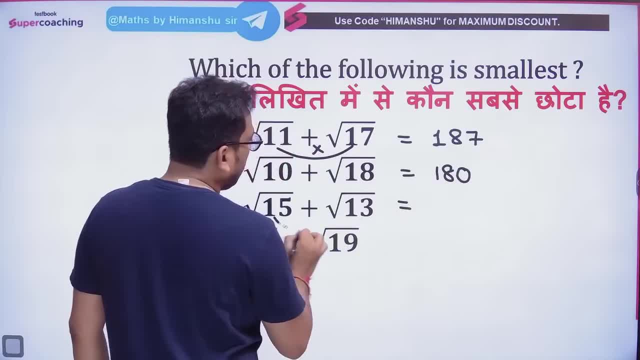 When you multiply here, how much will it come 180.. When you multiply here, how much will it come? 15, 3,, 45,, 4,, 15,, 15,, 15,, 4, 19.. 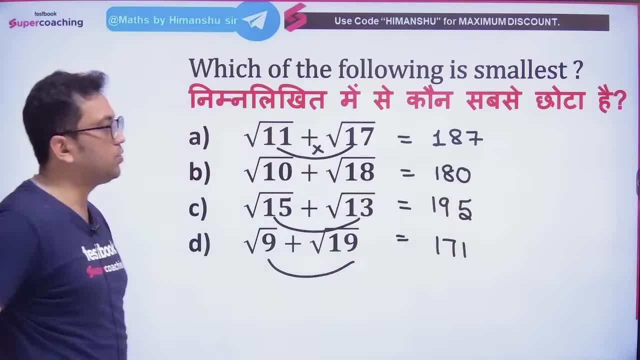 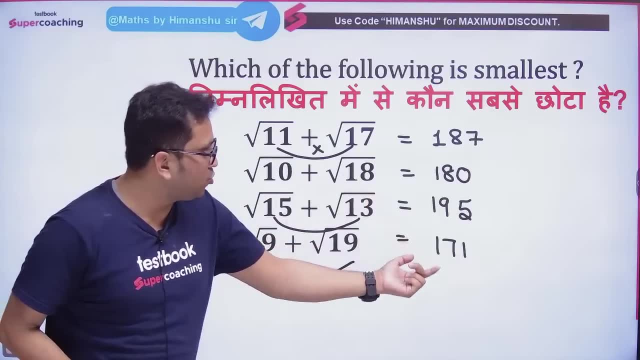 And when you multiply here, how much will it come 171.. Do you understand what I am saying Now? we have to see which is the smallest in this. We have to pick the smallest. So, brother, tell me which is the smallest in this. 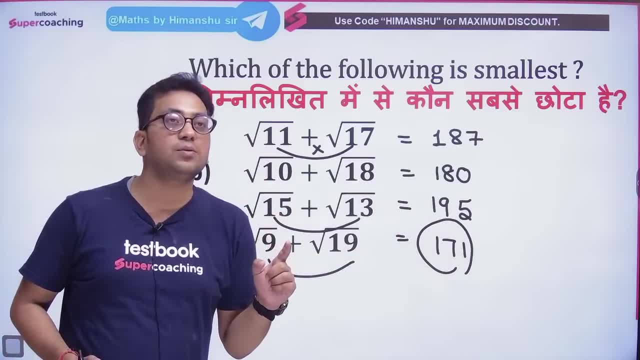 So this is the smallest. That is, which is the smallest? D is our answer. Is D the answer for all of them? D should be the answer. Where is B coming from? B is big, isn't it? B is big. 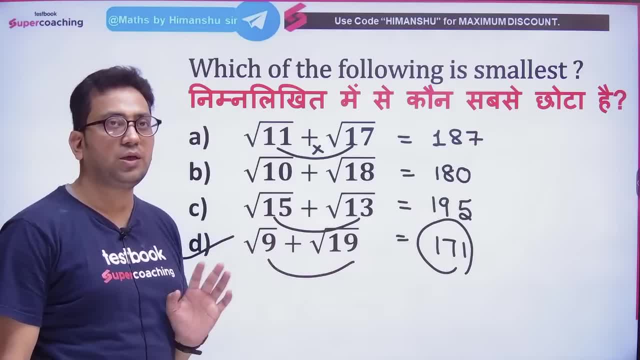 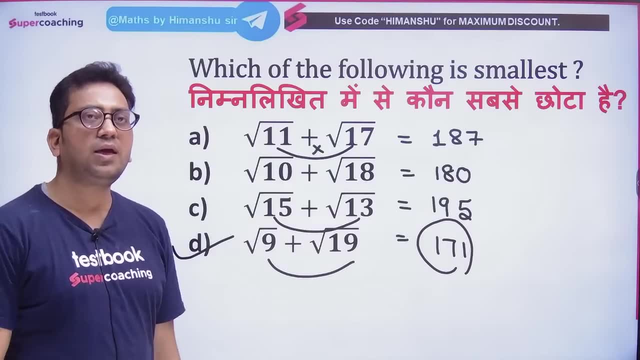 A is also big. If you have asked a small question, then D should be our answer. Okay, Now, why are you making a mess? Don't do this, Okay, Yes, Okay, isn't it? So D will be our answer. 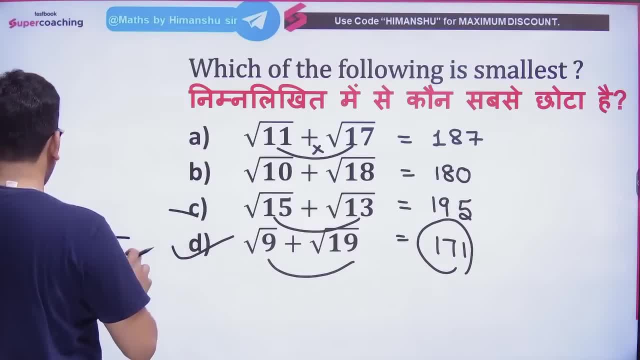 Son, this is the smallest Next question. Next question is coming in front of you. Look at the next question. Come on, make this question shine. Come on, make this question shine. Let's see how many children are able to answer. 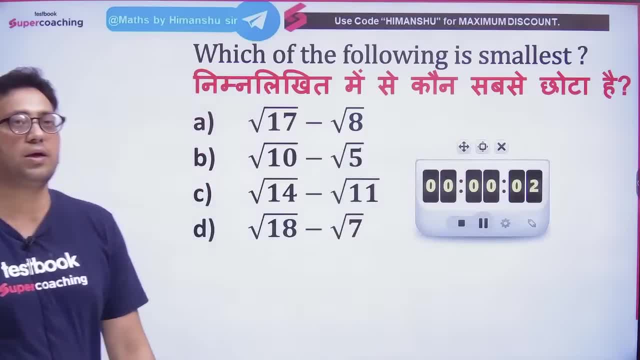 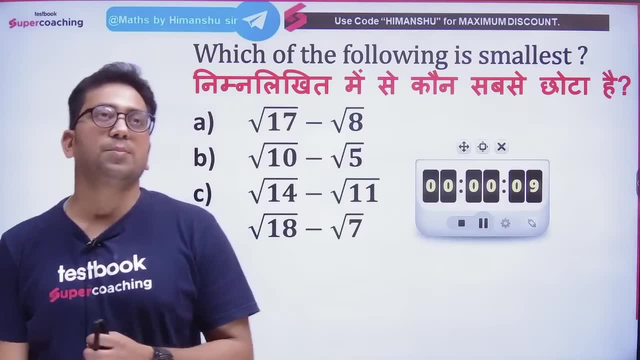 Okay, Let's set the timer for all of you: 20 seconds. 20 seconds Answer All of you. Come on. Manju Hina, Babita, Muhammad Baris, all the children. Ruchi Kishore, all the children. 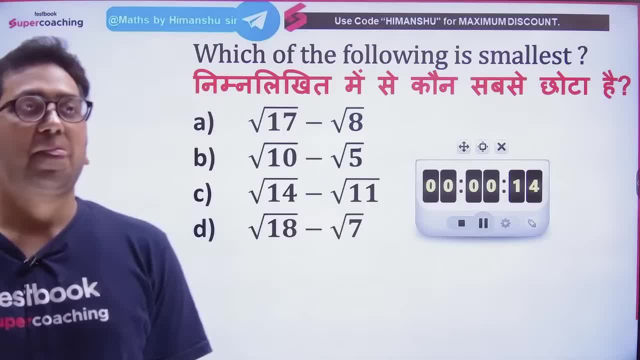 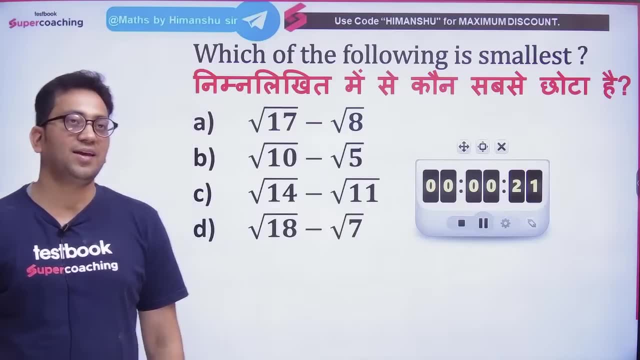 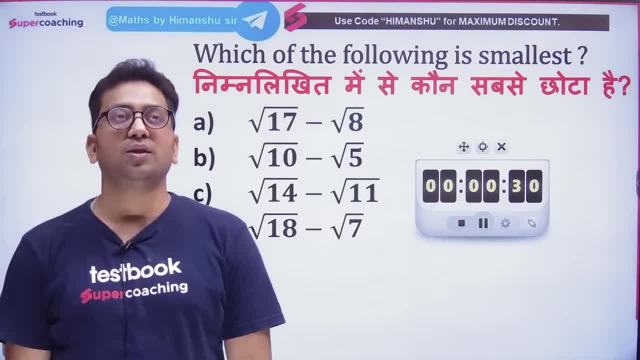 Then it is equal to performance. One or the other thing is same: Either Yoke Fals or Performance Fals. Okay, So we will also explain that too. Why are you getting worried? We will tell you all the things. 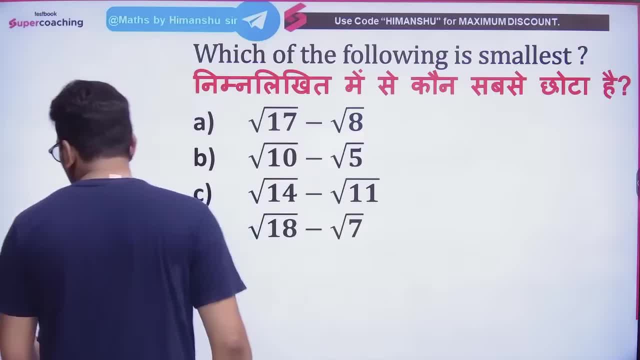 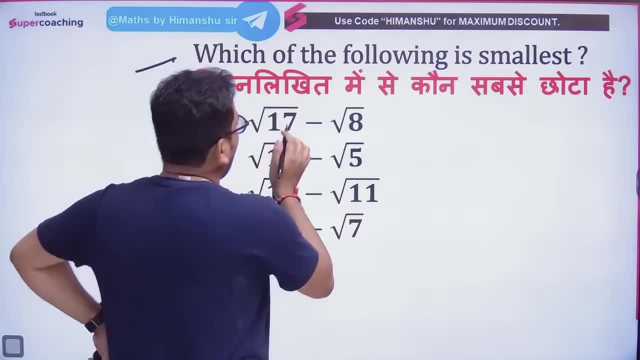 Have you ever left anything? Tell us, Tell us. Say it fast, son. What will be the answer? Yes, So we are going to B. Many children are okay. Now let's see. You saw, we add 17 and 8.. 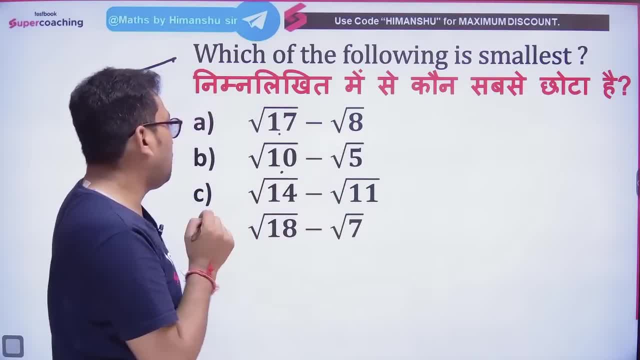 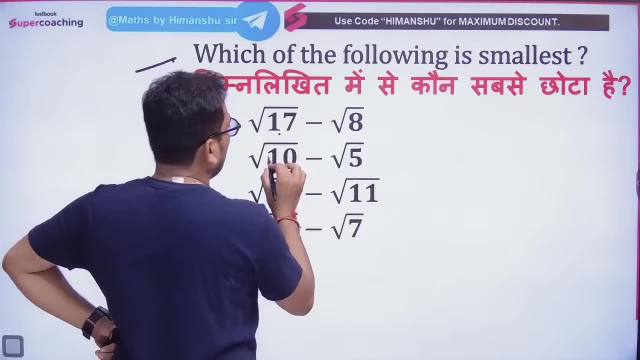 So how much does it come 25.. We will add 10 and 5. This is 15.. Yes, here it went wrong. You do like this, you can do 15. sorry, you can do it like this because I have to tell you the concept. 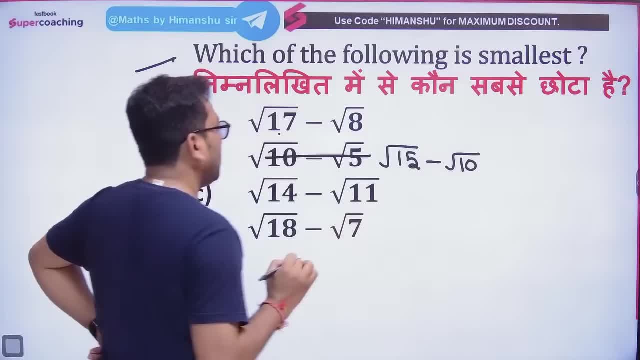 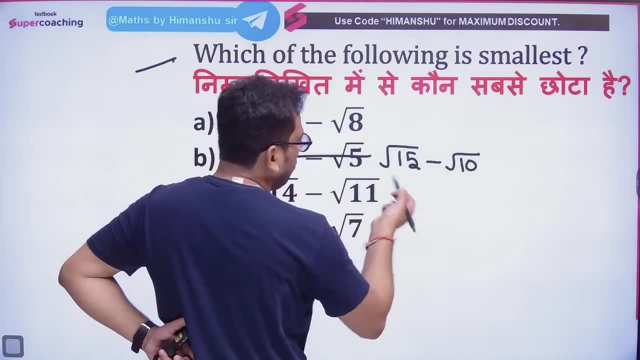 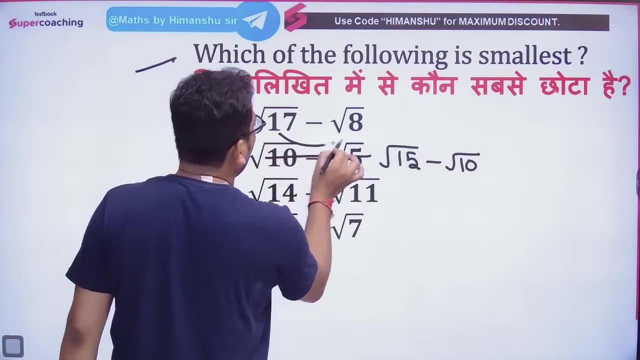 there is a mistake here. do 15 and 10. do 15 and 10. do correction in this, no problem. then 14 and 11 will be 25, 18 and 7 will be 25. that means the result is same here. now our child will do the multiplication. 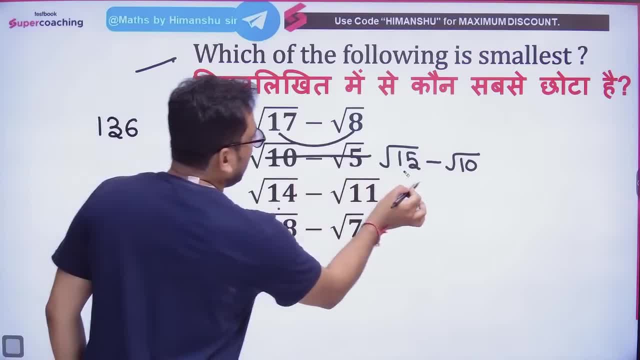 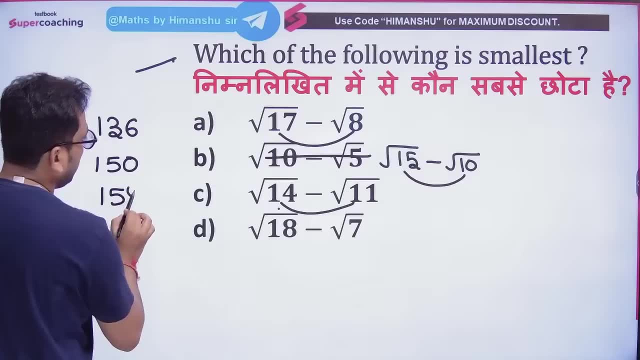 17 multiplied by 8 is 136, then 15 multiplied by 10, that means the result is 1.5. then 14 multiplied by 11, that means the result is 154, and 18 multiplied by 7, that means the result is 126. 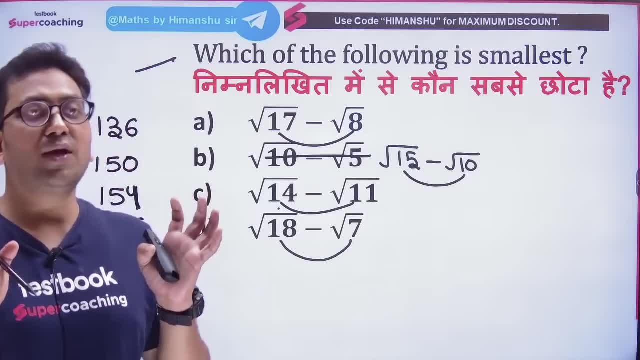 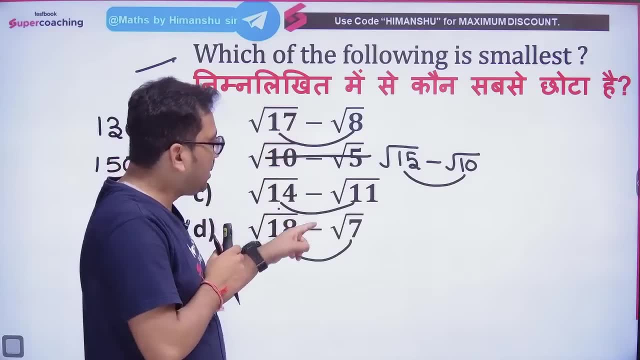 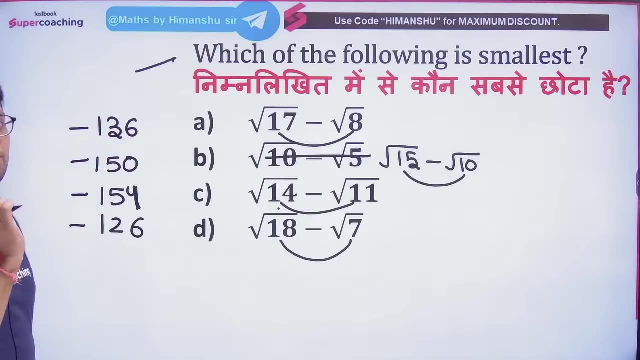 do you understand? did you understand or not? now try to understand here one thing: you have to keep in mind that there is no plus, there is minus. so you put minus sign here, here, here, do you understand? you put plus sign if there is minus. 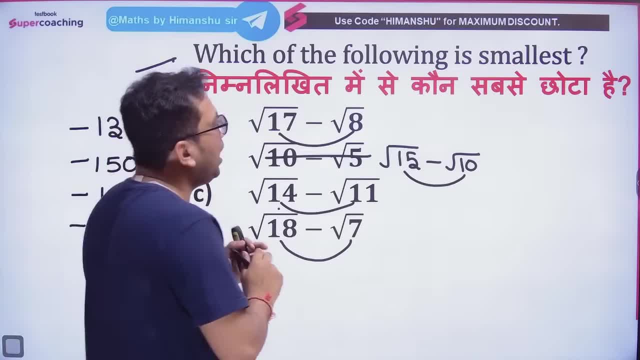 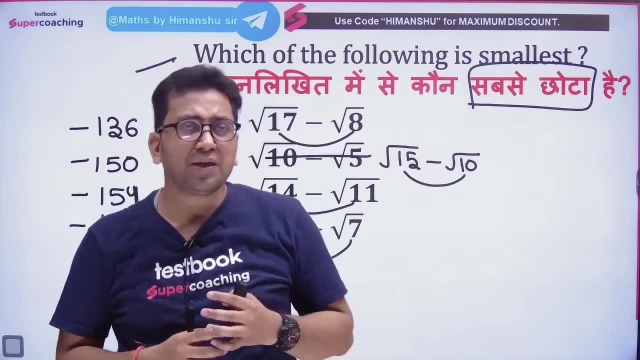 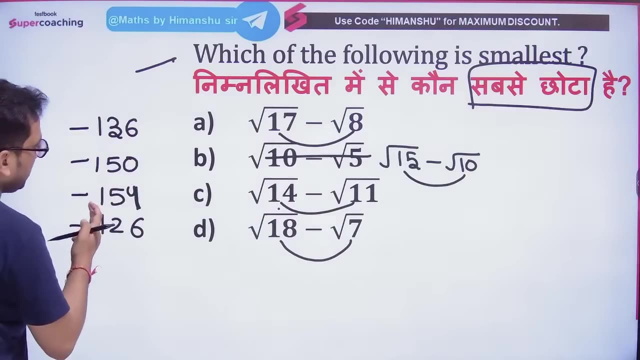 then there will be minus sign and all of you know that the smallest will be the one which is bigger in minus. the more the minus, as it is said, the more the negative. the smaller is the minus, the more the negative. say which one is more negative? this one is more negative. 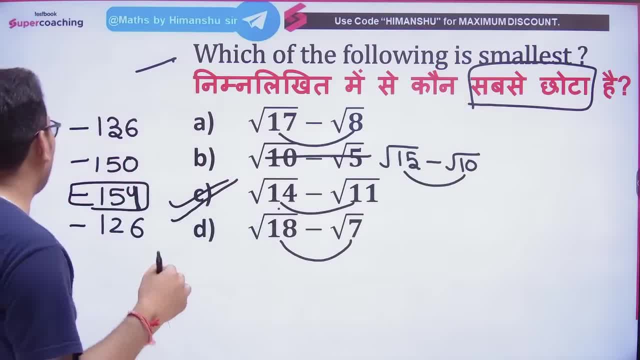 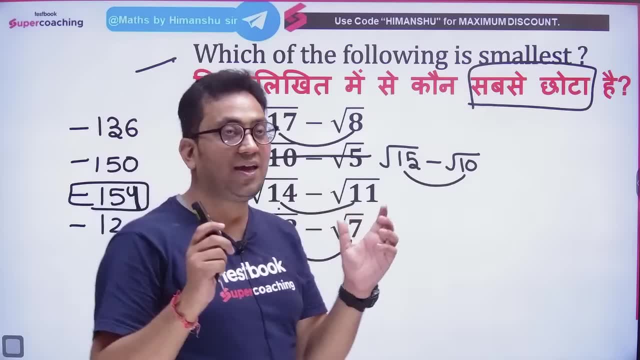 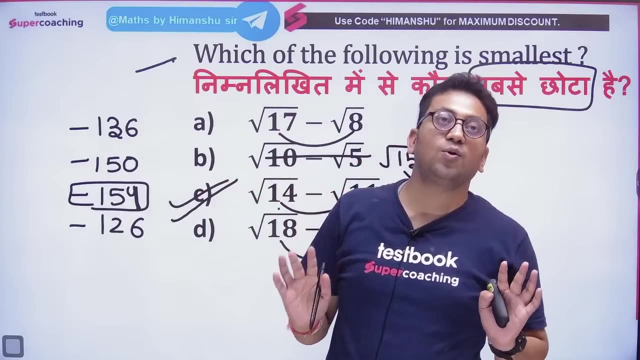 so this is the smallest. so C will be our answer, but not this why? because here there is a minus sign, here there is a minus sign, where there is a minus sign. you will put minus sign in front of all and then you will see the one which is more negative. 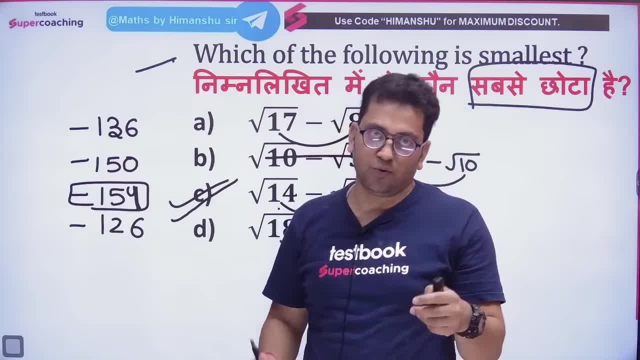 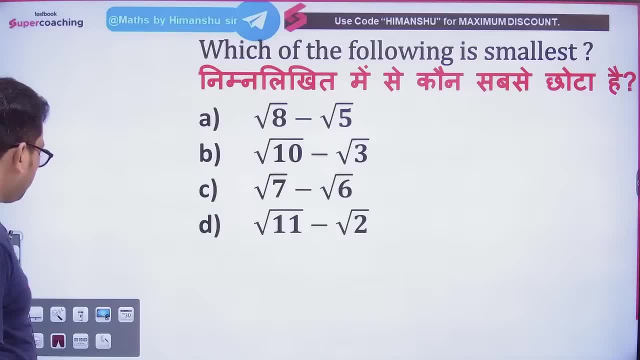 that is smaller, the one which is less negative, that is smaller. do you understand? next question: tell me what will be the answer. answer all of them. you are able to answer all the questions you are able to shine. do it boundless, not only one, whatever you would ask. 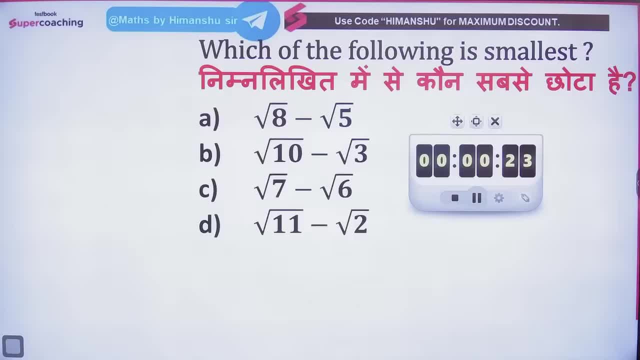 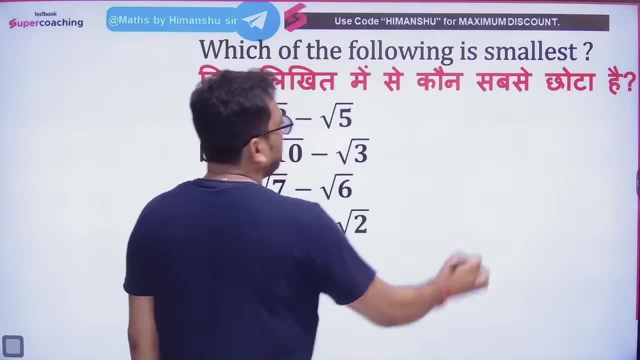 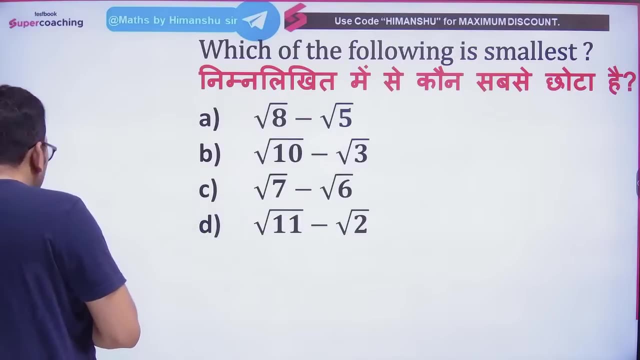 that C, this is the bananas, given the name boundless. so it gets gold. and Ok, let's see what we will do. we will do the multiplication. Look, the equivalent is the same as 8 and 5 is 13.. Ok, here you have to do the equivalent. don't look at the interval. 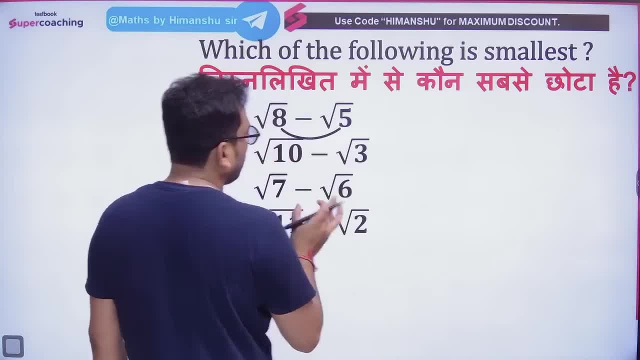 The equivalent should be the same: 10 and 3 is 13,, 7 and 6 is 13,, 11 and 2 is 13.. This is also a concept, because when we do whole square, then this term remains positive. 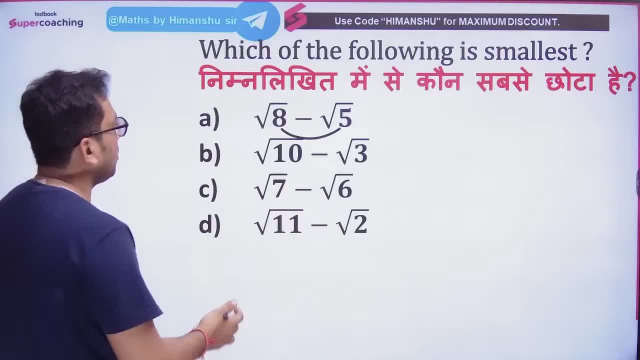 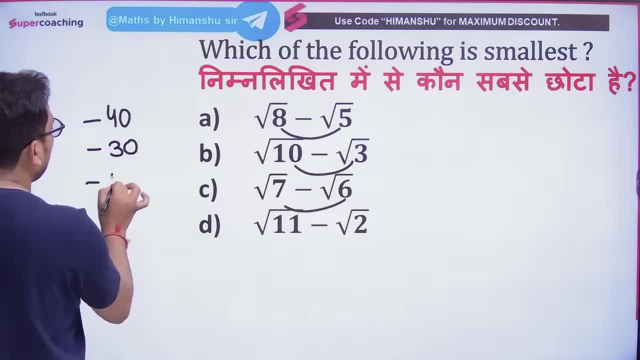 Just minus 2a also comes. that's why I am multiplying them. So 8,, 5, 40 is in minus 10, 33 is in minus 7,, 6, 42 is in minus 11, 22 is in minus. 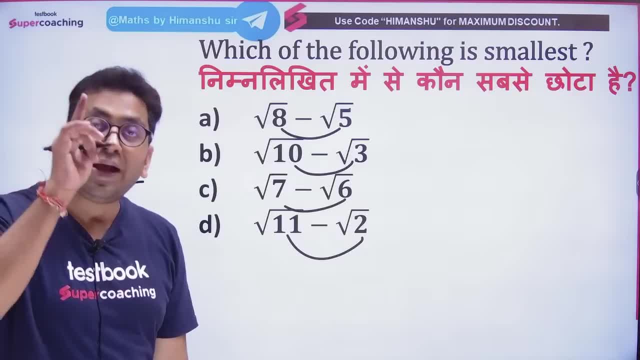 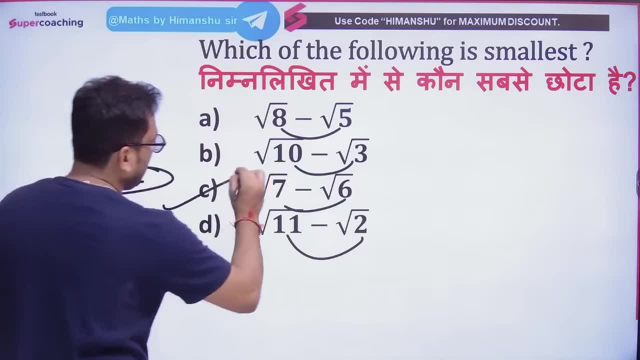 What did you ask? The smallest, The one who is the biggest in minus the one who is more negative? that is the smallest. So which is more negative? This is more negative? Here also, C will be our answer. C answer is coming. everyone's answer is very good. 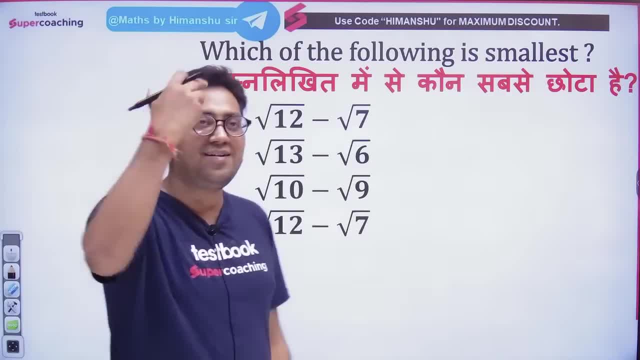 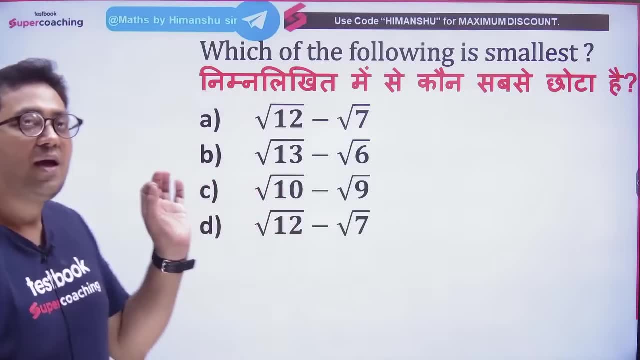 Look at this. I mean you are answering, See, do you understand? There is no such child who is answering wrong. as I can see, Everyone's answer is C. The next question is coming. All children answer. tell everyone correctly. 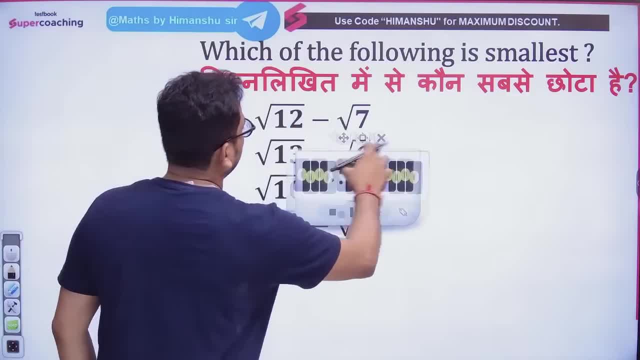 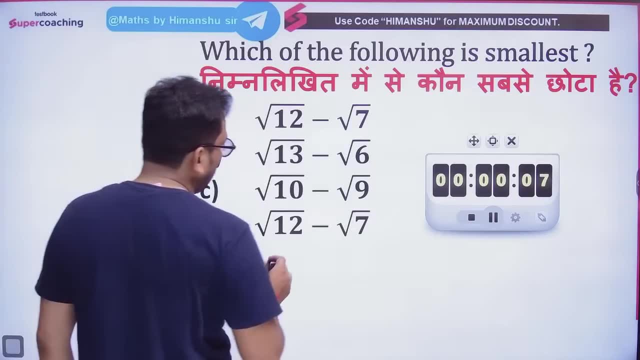 what is the answer? Let's see how many children are able to answer. Answer: son A and D are the same. right, A and D are the same. let's change it a little. Okay, let's change it a little. 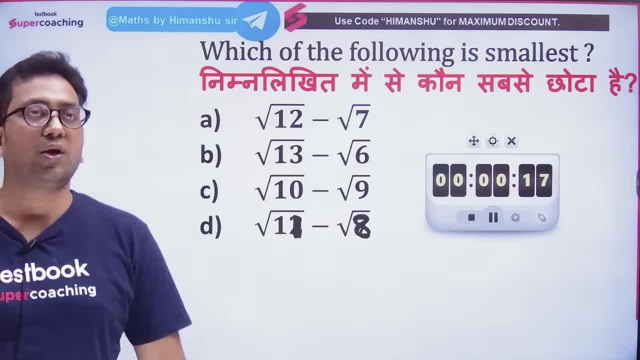 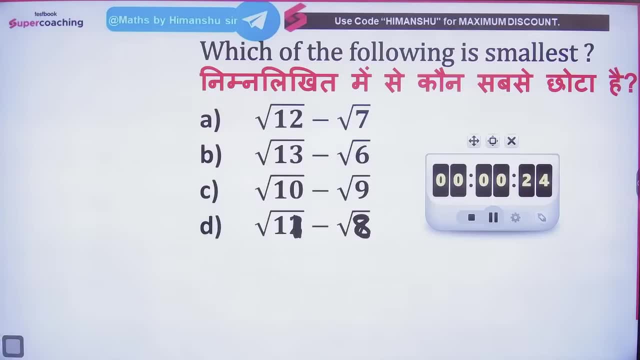 So do 11 and 8.. A and D were the same. we have changed it. 11 and 8 have been done. Come on quickly tell me what the answer will be. You have to tell which is the smallest among them. 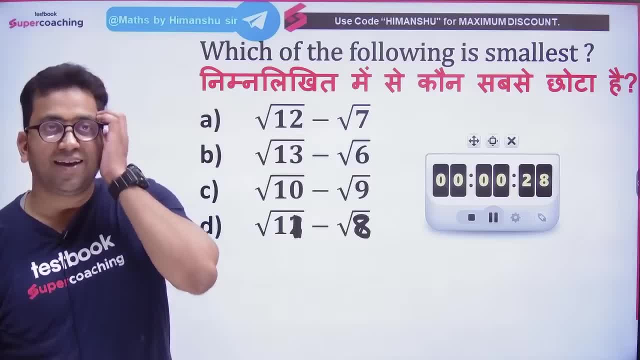 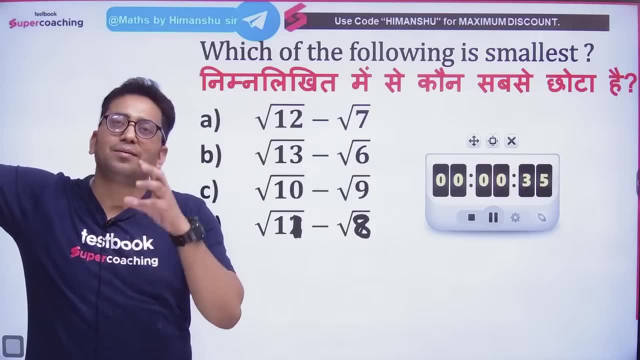 Okay, A and D are perfect, C and E come and M. That is the question. You didn't finish because everything was wrong. Ah, okay, then just write it down. These are the questions that I was talking about here. Everything is in that thisqui. 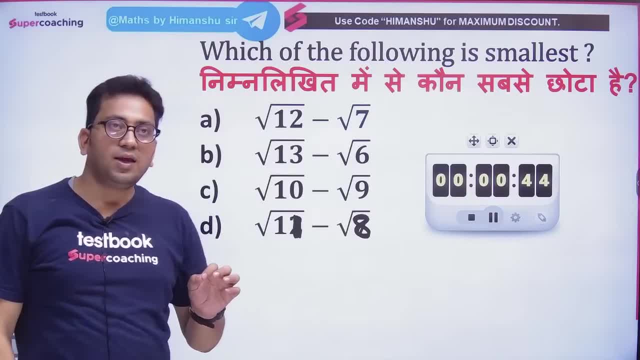 is not thisqui, thisqui is this culpa? Everything isexcept under nature, Because every child is a child, Not really no children'. Oregon issues less subject fields, which means have more than our child, and where we also have many students. 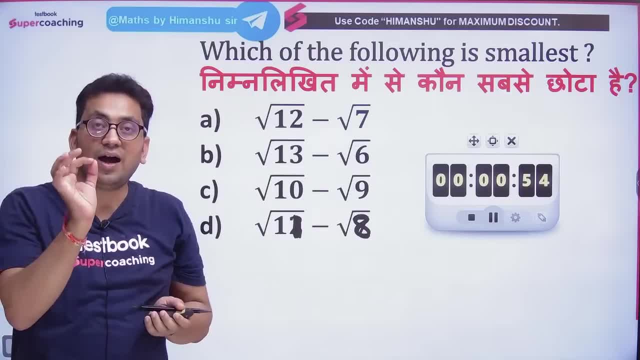 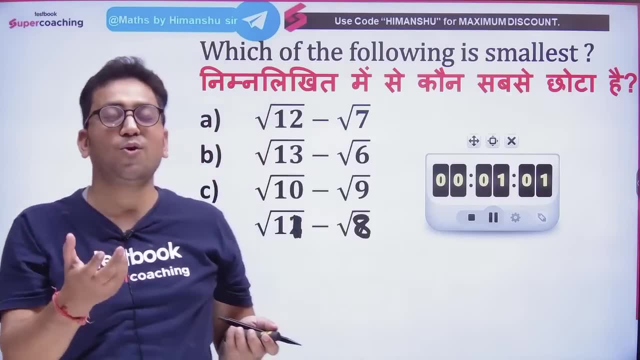 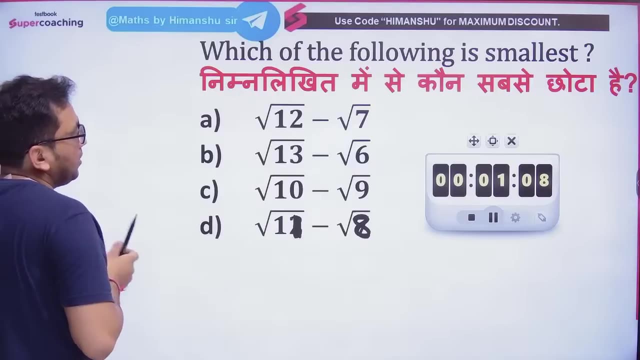 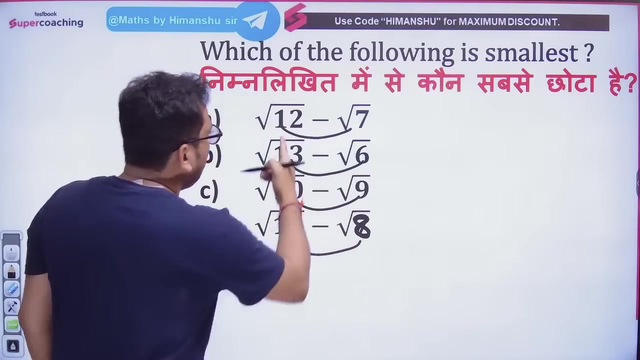 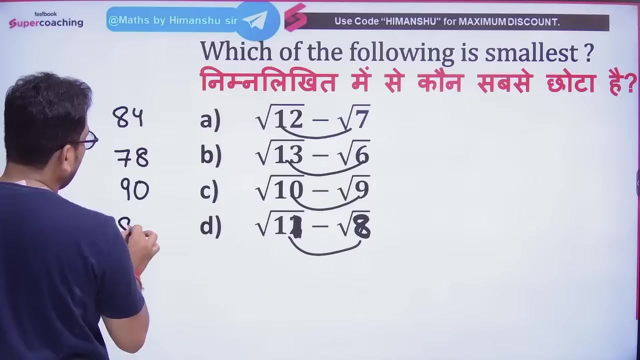 Otherwise, tell the zero's not to come and do lesson, but to do so Like there are too many children. I am saying this because I teach you in a good way and I want everyone to study in a good way. that's why I am saying this. okay, come on, let's come to this question. 12 and 7,, 19,, 13,, 6, 9,, 10,, 11,, 11, 8, 9,- this is the equivalent of 19,. now our child will do our calculation: 12, 7, 84,, 13,, 6, 78,, 10, 90, and 11, 8, 88,. sir, we have put minus. now we have to do our calculation. 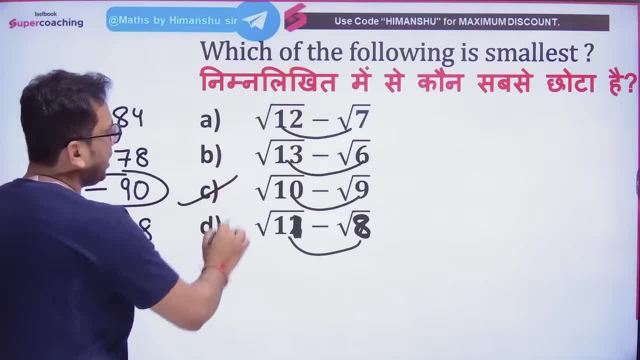 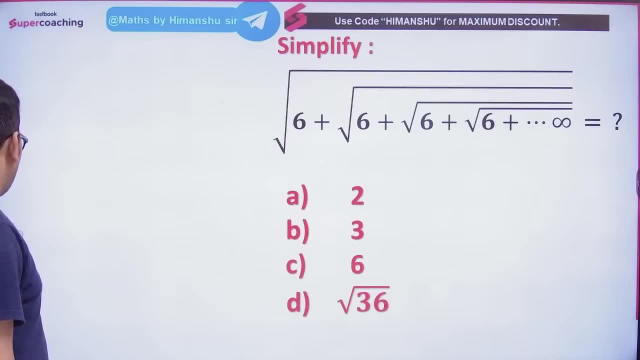 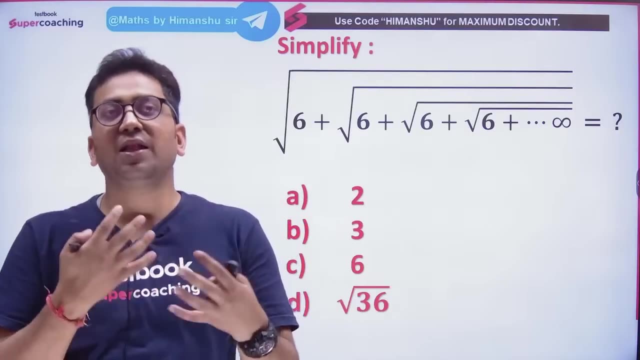 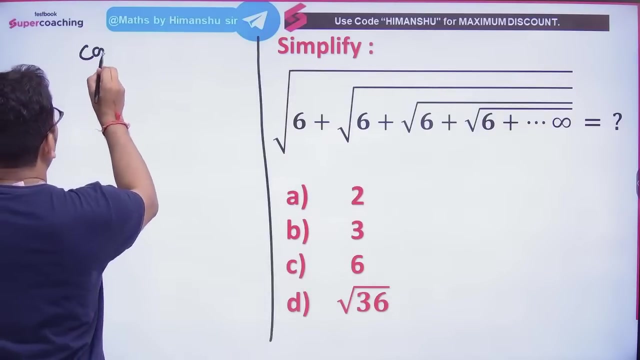 we are seeing the smallest, that is, minus 90, will be our answer. brother, today you are going crazy. you are getting C answer everywhere, isn't it? C answer is coming. very good, very amazing. here is the next question, now this question: what did I do? I have changed for you in every place in the questions. now this question is of simplification. in front of you, first of all, I will explain you its concept and then the way to shine. okay, then understand the concept, all of you, all of you. what is ready? then this: 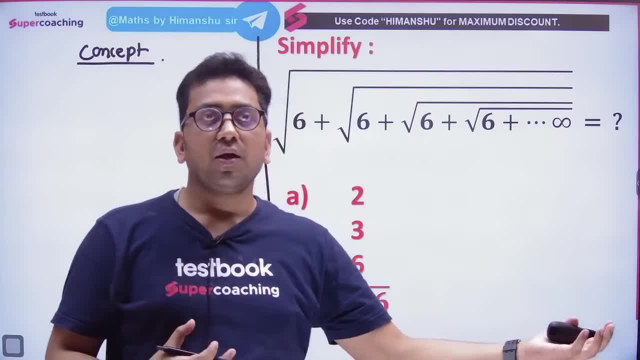 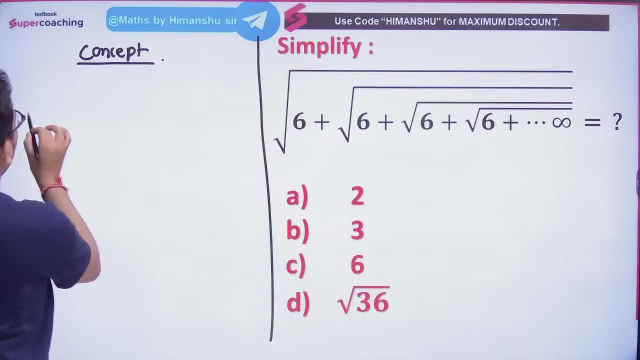 patience, keep it that. yes, I will understand the concept too. okay, and then I will understand the way to shine. don't just run towards the trick, then understand the concept too. see, son, what is this here? it is in this way, in 6 sets. in this way. it is going on, going to infinity. here. I have considered it equal to x, the question mark: I have considered it equal to x. okay, now tell me once, if I remove the square root from here, then the square will go up here. 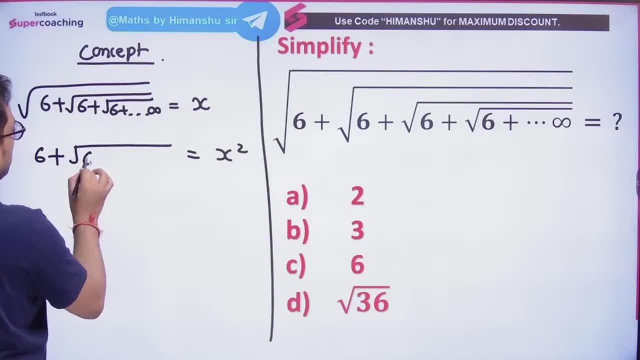 that is, how will you see when this root is removed, then the root is removed from here, but it is still attached to it. it is still enjoying in the root, isn't it, Brother? there is a roof on it. there will be a roof on it. yes, it will be okay. now tell me once if this was the whole x, I separated one from it, left the rest. then, brother, it will still be equal to x. 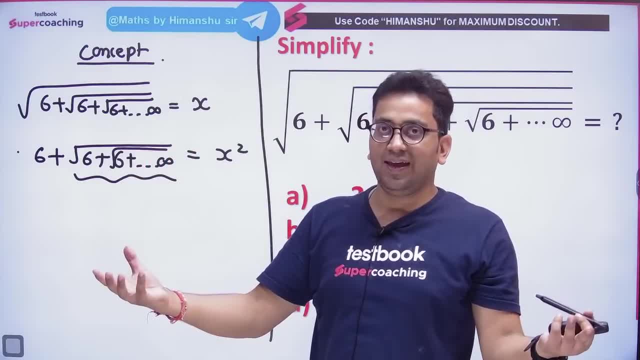 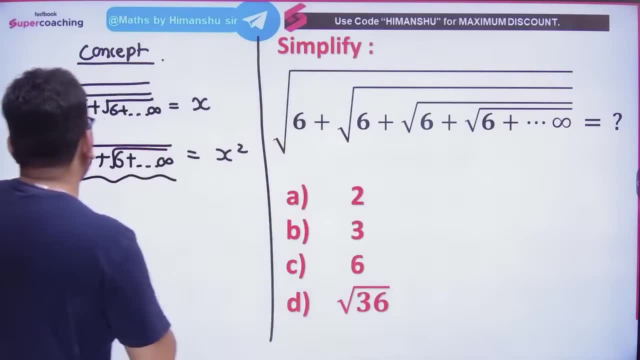 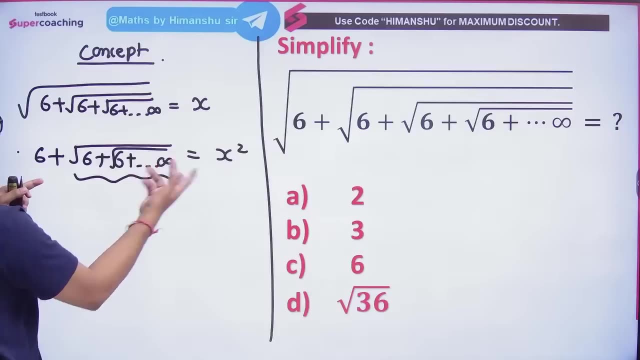 then also, it will remain the sea. it is not that it will become a river or a pond. no, brother, separate only one drop, I tell you, fill the bucket and separate it, no problem, it will remain the sea. so we have separated only one from here. if this is the whole x, then, brother, this is also x. it is still going to infinity. so this is x, that is 6 plus. I can call it x because I considered this whole equal to x. this is equal to your x square. now, see, I will take these two and take them there, son, this will be x square. 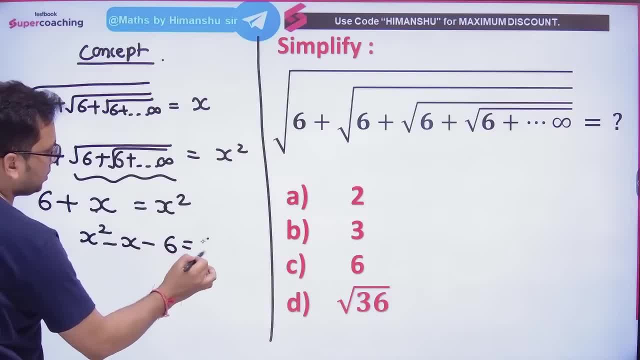 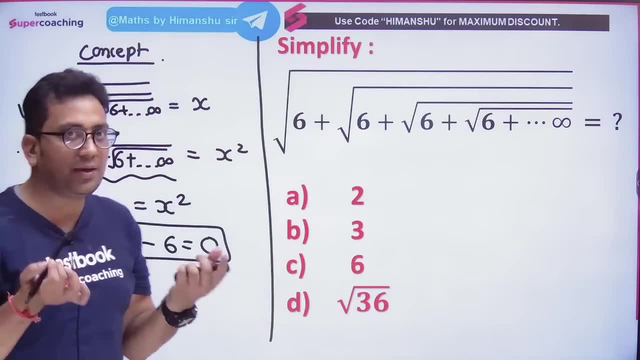 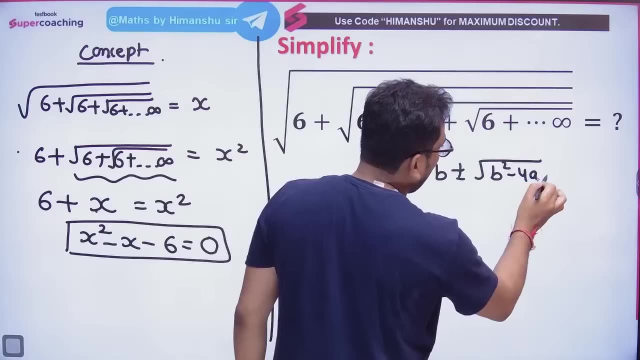 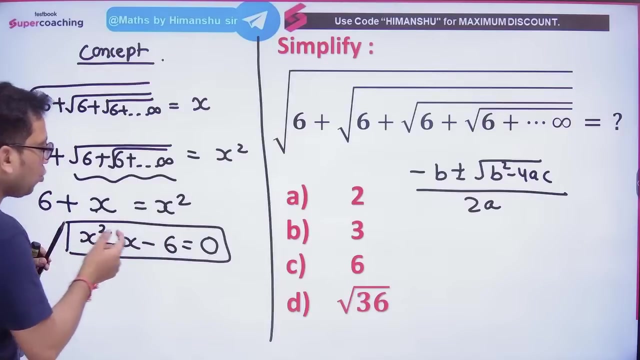 this will be minus x and this will be minus 6, it equal to 0, this is a quadratic equation of two fractions, that is, it has become a quadratic equation where I can remove it from the method of split. this is your formula: minus b plus minus root b square minus 4ac divided by 2a. I can remove it from this method also, though it will be solved from this: how to see: see 2 factors of 6 in this way that by, by reducing, I am getting minus 1, then you will say: 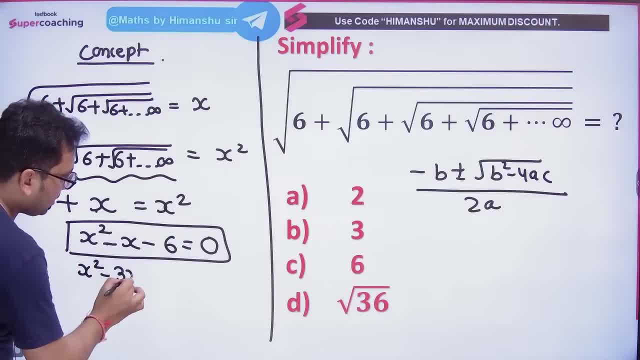 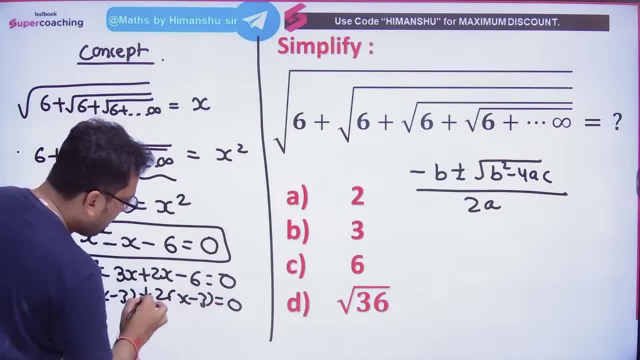 and from here, if I take 2 common, then x minus 3.. Okay, And then here x minus 3 is common in both of them. So this came out: x plus 2 will remain inside, which is equal to 0.. 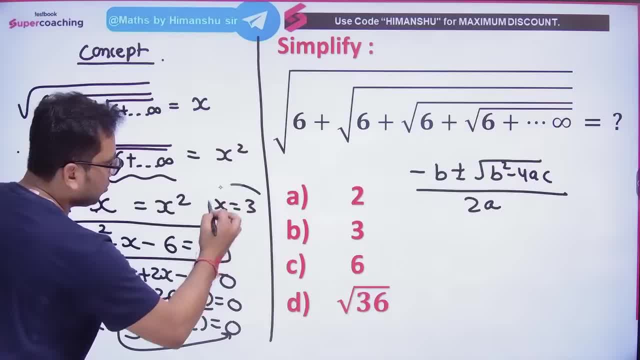 Once you put x minus 3 equal to 0, then x equals to 3 will come. Once you put x plus 2 equal to 0, then x equal to minus 2 will come. Minus 2 is not possible. 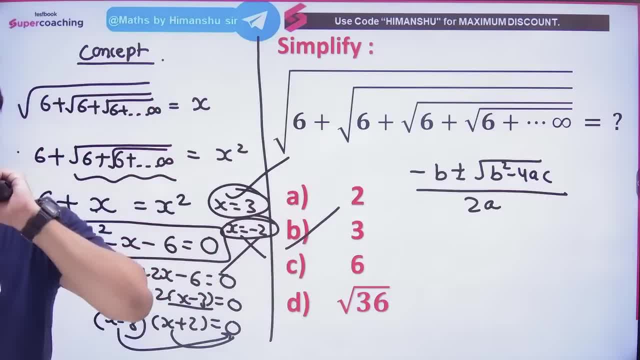 So 3 will be our answer. This is our answer. Okay, But this is your conventional way. You don't need to do this at all in the exam. What you have to do is see the way of shining. You just have to see. 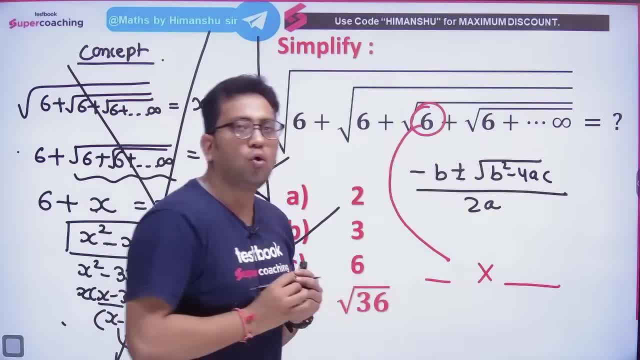 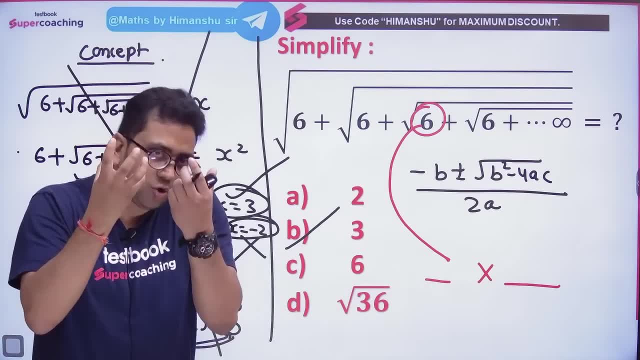 which two factors can I break the 6? in Which two factors See multiple. I can break it in the number. Which two numbers can I break it in So that it is 6 by doing the number, but the difference between them is 1.. 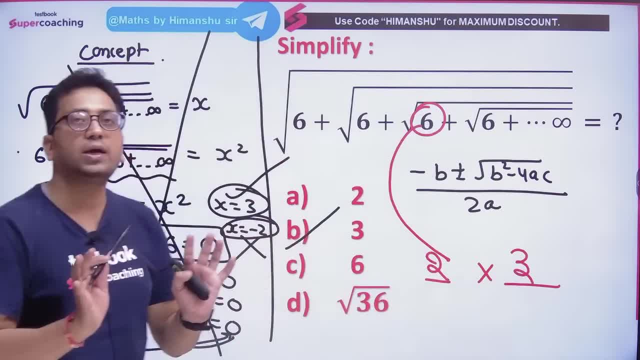 So you can say it is 2,, 3, 6.. What It is: 2, 3, 6. Say yes, it is 6.. And you will see on the number that if there is a plus sign here, 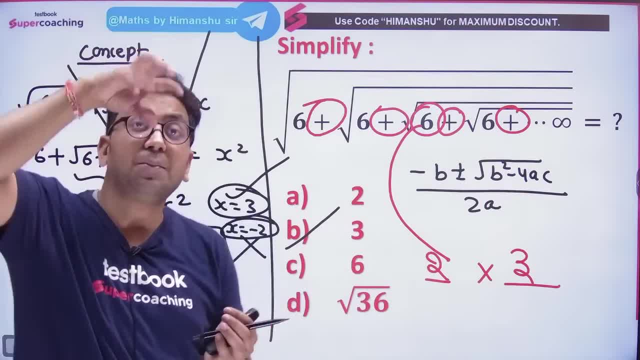 how is it? It is a plus sign, So you will take the big one. Plus means you will take the big one, So it means 3 will be our answer. That means option B will also be our answer. 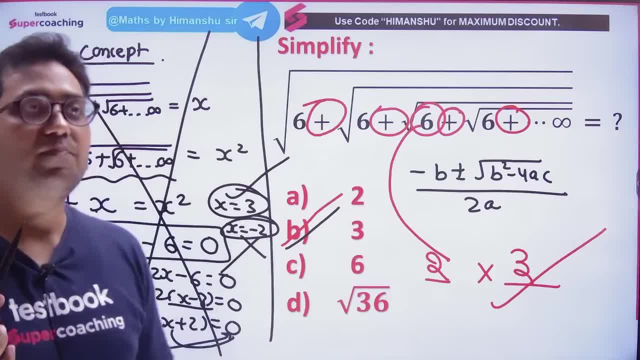 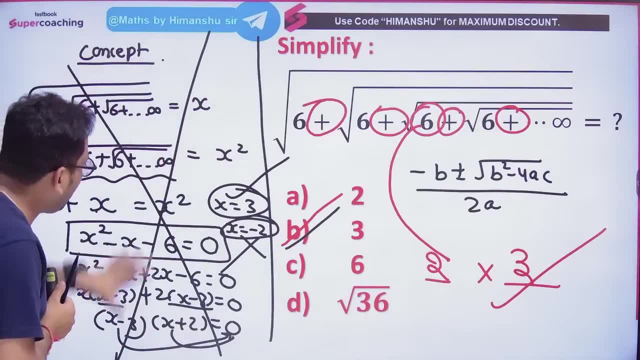 Are you understanding my words? Are you understanding, Sir? shine it and tell me Take it. shine it and tell me There is no problem. It is 2,, 3,, 6.. Okay, I have told this for those who are hungry. 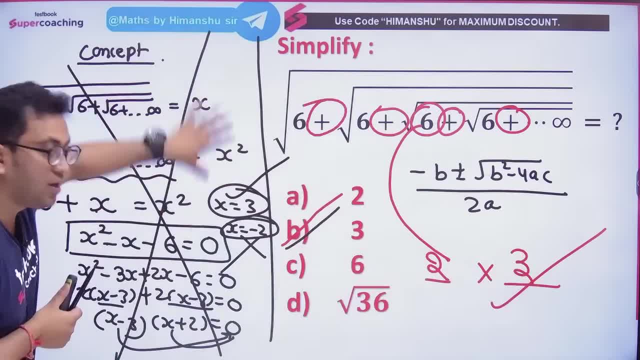 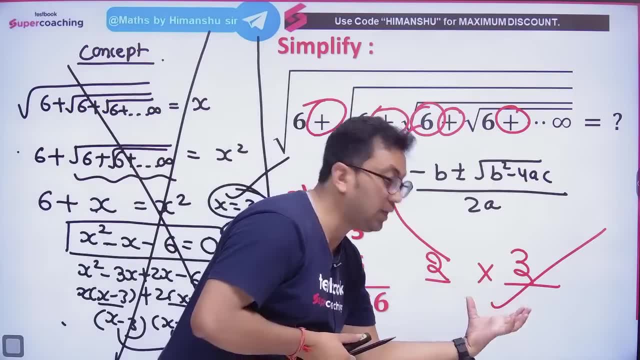 Sir, I have told this, Sir, I have told this, I have told this, I have told this: Those who are hungry from here will be gone, And those who are not able to escape from here will be gone from here. 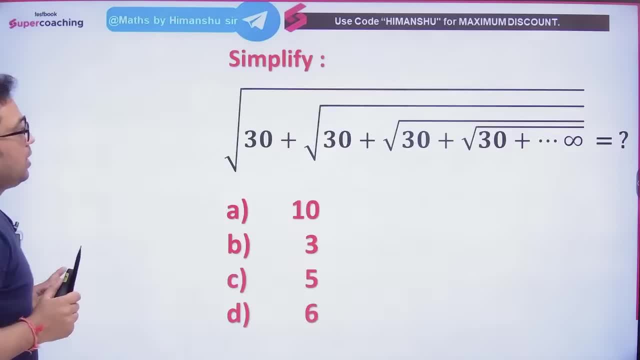 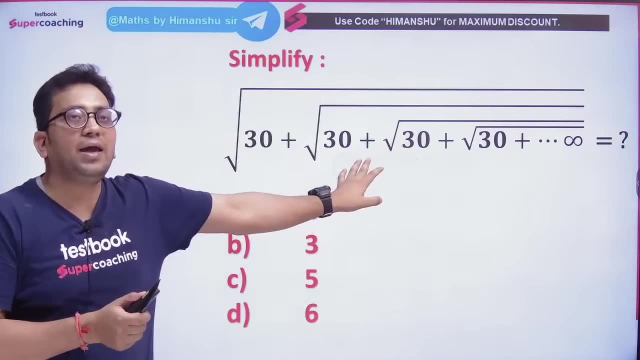 Are you clear? Next question. Next question: Shine it fast Break the number that is seen in two such numbers that by multiplying it it must come here. Okay, But the difference between them should be 1. Okay. 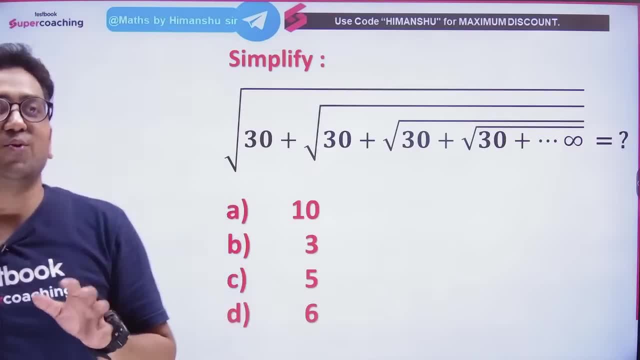 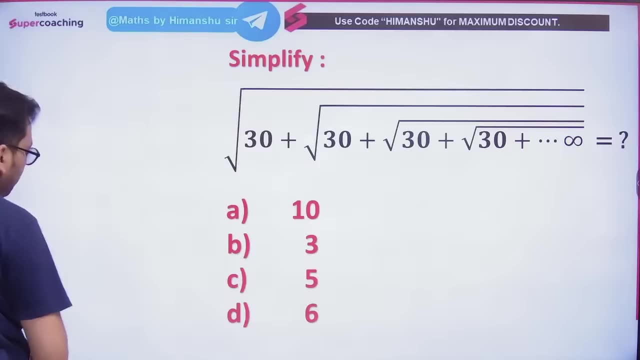 And if it is a plus sign, it is a big number, And if it is a minus sign, it is a minus. Nothing will be answered. so tell fast, Quickly, with speed. Look it is 30.. What do you have? It is 30.. 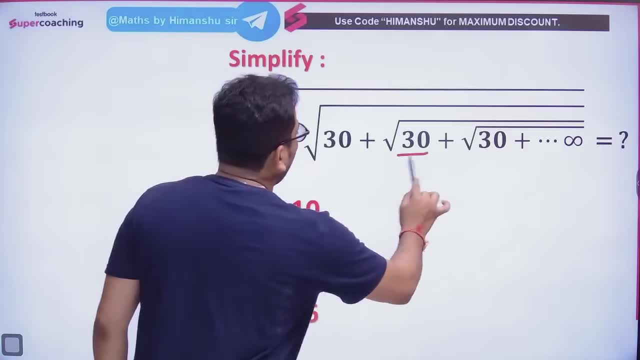 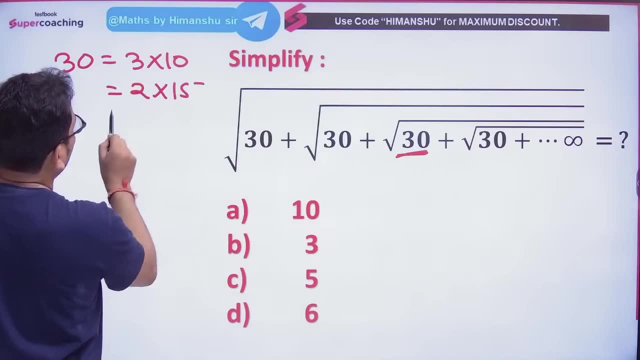 What will our child say? 30.. How can we say 30?, Sir? we can say 30 is 3 times 10.. We can say 2 times 15.. What can we say? We can say 5 times 6 is 30.. 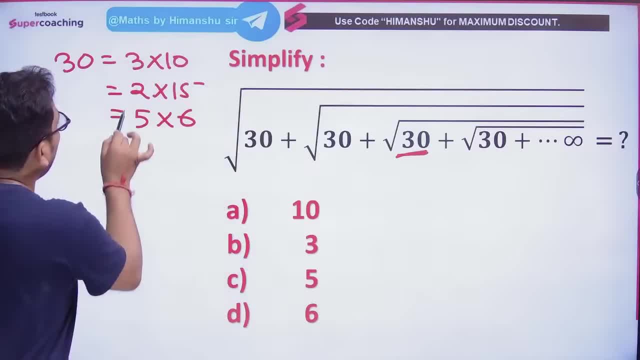 Tell me where is there a difference of 1 between them? So you will say, sir, there is a difference of 1 between them in 5 and 6.. So just take these two, That is, we have to take this pair. 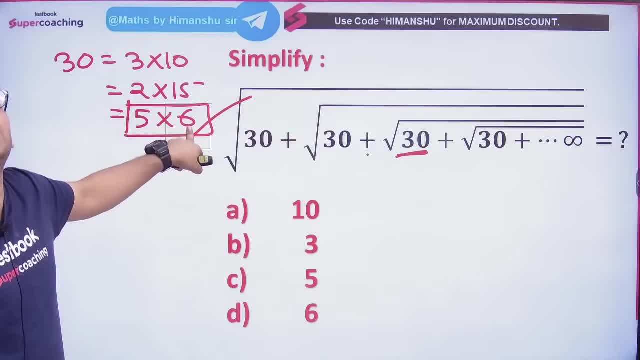 Now, if there is a plus sign, then you will take a big number, that is, you will take 6.. So 6 is our answer. Where is the end? Do you understand now? Are you applying all the sixes or not? 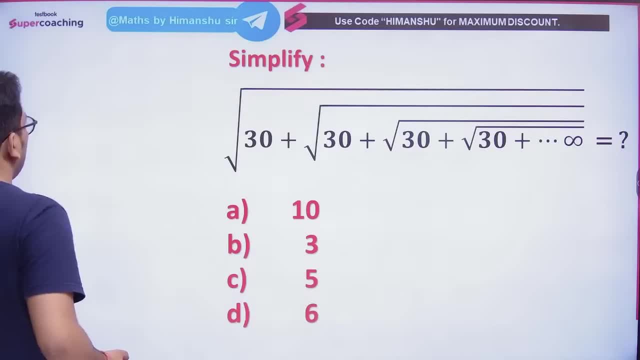 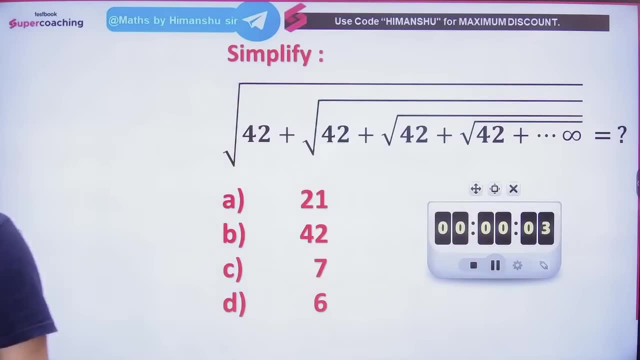 Are you understanding? Next question: Shine son, Tell me what will be the answer. I have given you the time of 20 seconds. Let's fly. Tell me what will be the answer. 1,, 2,, 3,, 4, 5.. 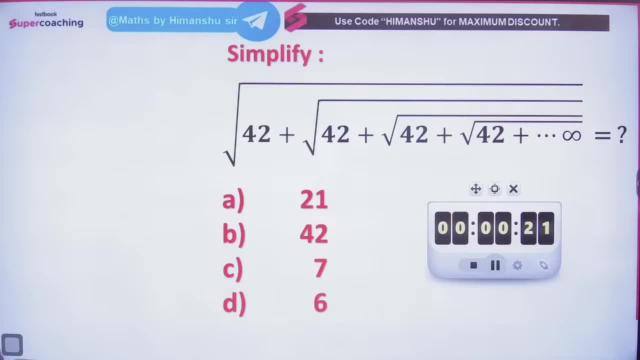 5,, 6,, 7,, 8,, 9,, 10,, 11,, 12.. 6,, 7,, 8,, 9,, 10,, 11, 12.. Right, You have answered all the seven answers, dear. 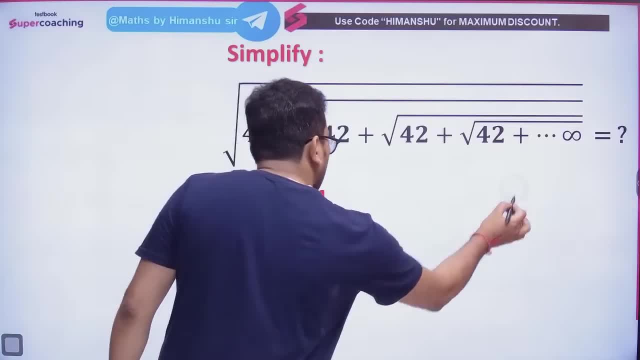 Now let us see this. I have answered all the seven answers, dear, And here is the question: What will you do, son? You have to divide 42 into 2 numbers in which the difference between them is 1.. 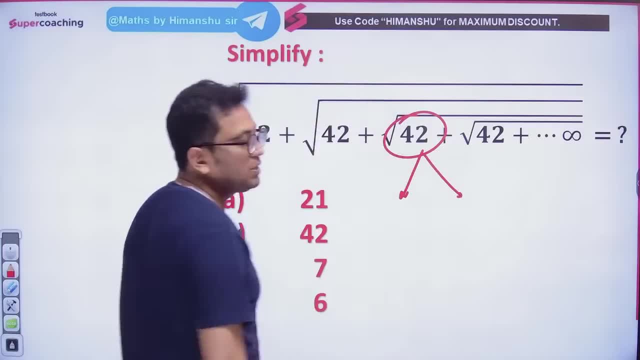 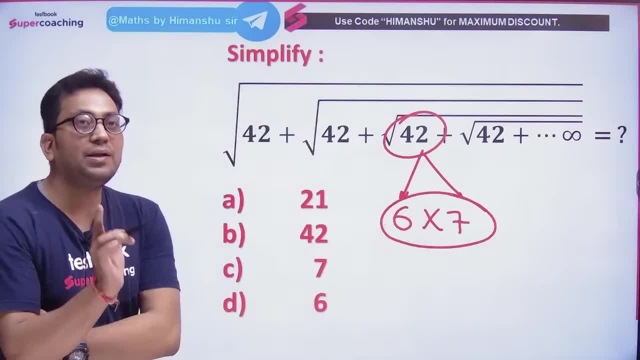 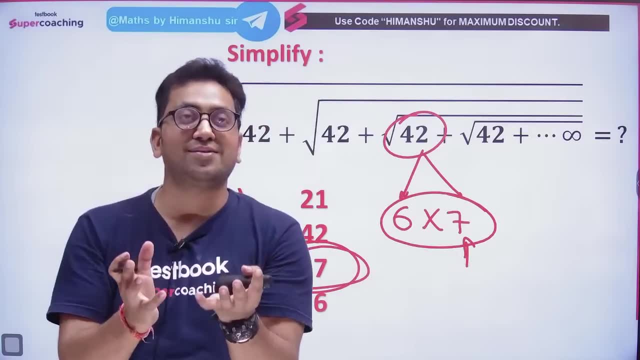 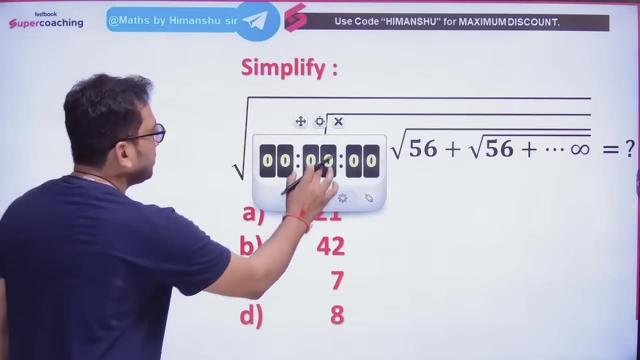 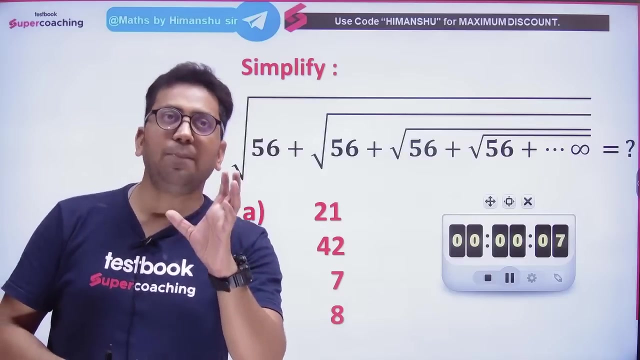 Say yes or no, Dear. I have said it, This is easy. If you say that it is a plus, sir, then it is a plus. then you picked up the big one. you picked up the big one, then we are together. I can see that everyone's answer is coming together. very good, very great. let's move on to the next question. next question: shine, son, tell me what will be the answer. 20 seconds time, the heart will print the questions inside you with the concept, with the trick in the mind. come on, tell me quickly. 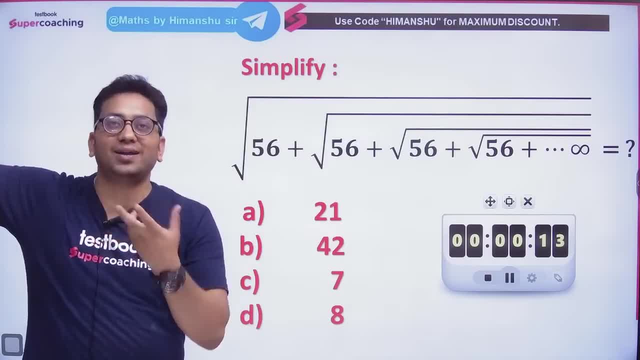 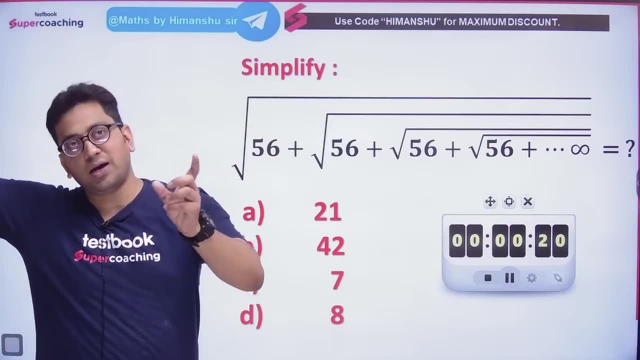 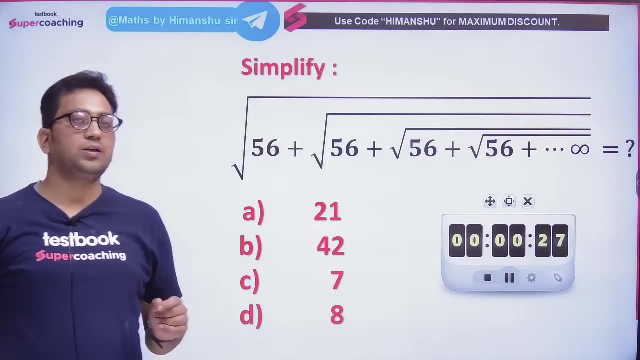 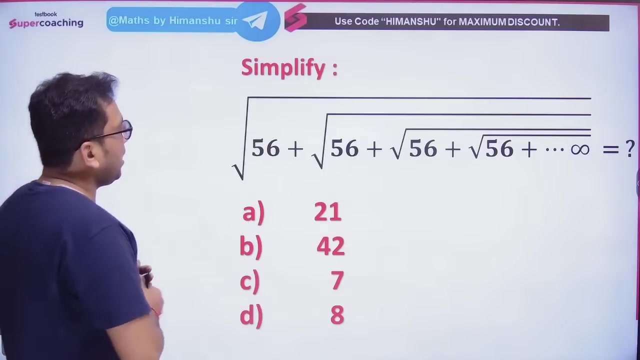 that is, I am not only teaching you to eat halwa, I am also teaching you to make halwa. okay, both things are learning: learn to make it and then eat it and have fun. tell me quickly what will be the answer. 56 has been given. this time, 6 seconds are remaining. everyone's answer should come. time is over here. this is 56, how will we break, sir, such a difference, such a number whose middle difference is 1, then everyone will see 7,, 8,, 56, there is no problem. 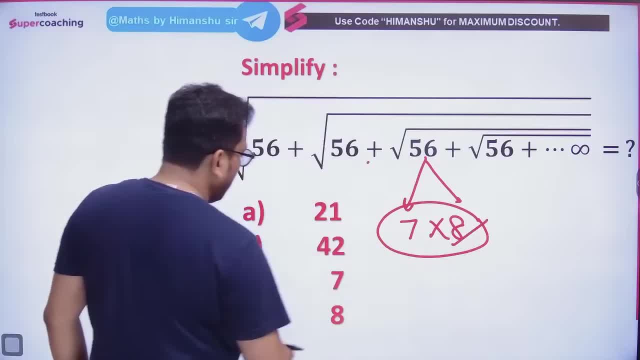 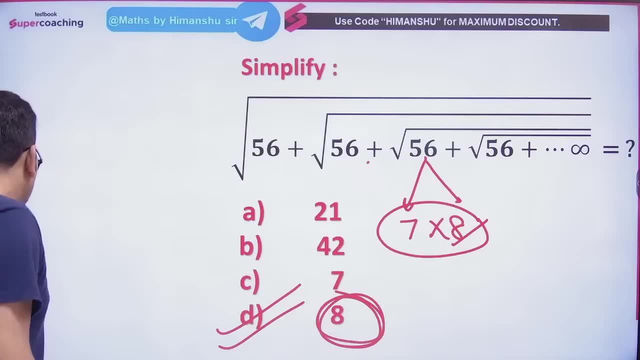 and if there is a plus sign, then we will pick up the big number. pick it up. pick it up, son, pick it up in your lap. 8 is our answer. everyone's answer is coming: 8,. very good, let's move on to the next question. 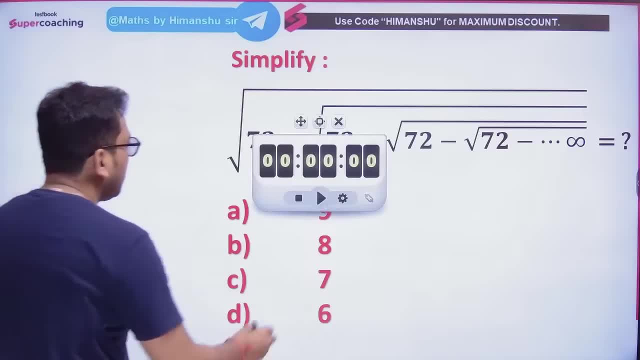 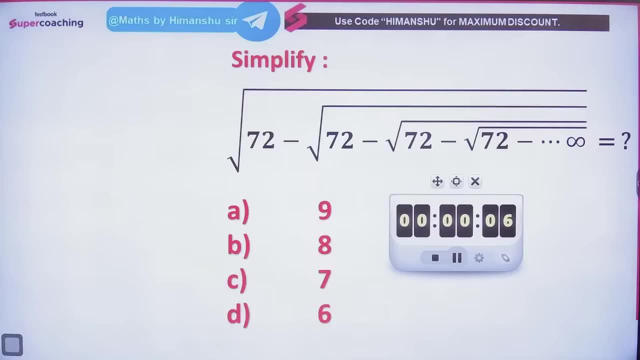 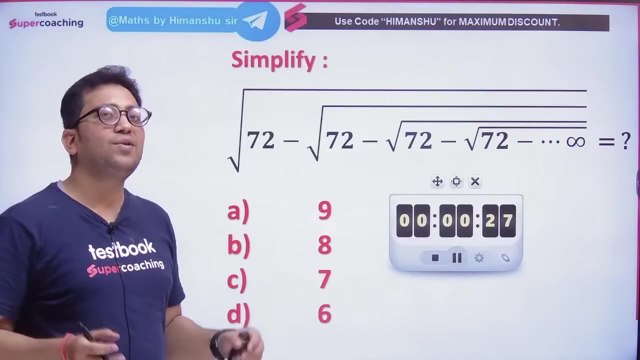 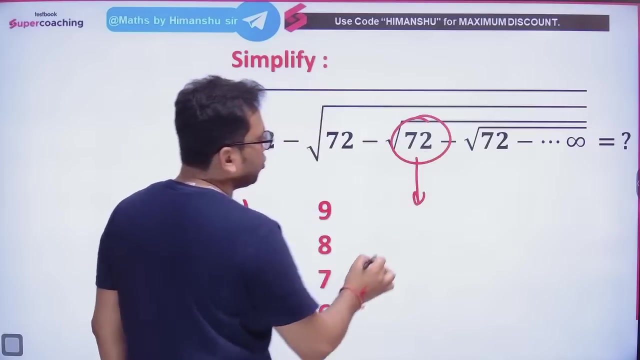 here. the next question has come in front of you. let's see how many children are able to give the correct answer. take 30 seconds time. 30 seconds. come on with speed answer. if you want to be negative, then it is negative, and first tell me about negative. then I have tell you why are you getting upset child? what is this son, this negative? there is no problem, your baster will remain there. you will break 72 in such two multiples between which there is one difference, so 8, in 72,, that is, there is a difference of 72 in 8,. 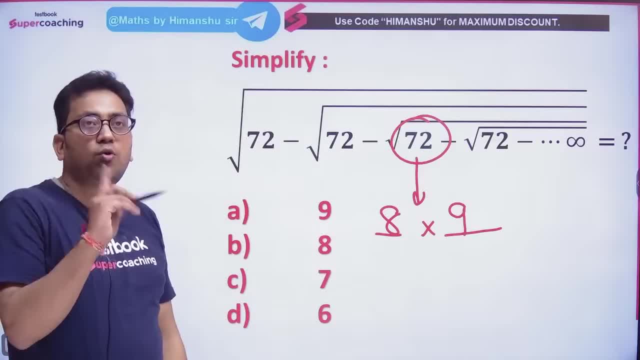 72 is equal to 1.. But if there is a sign of minus, then don't pick up the bigger one. You have to pick up the smaller one. That is, you will pick up 8.. 8,, 8,, 8.. 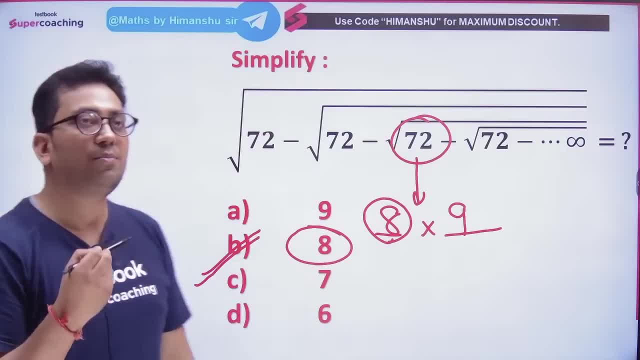 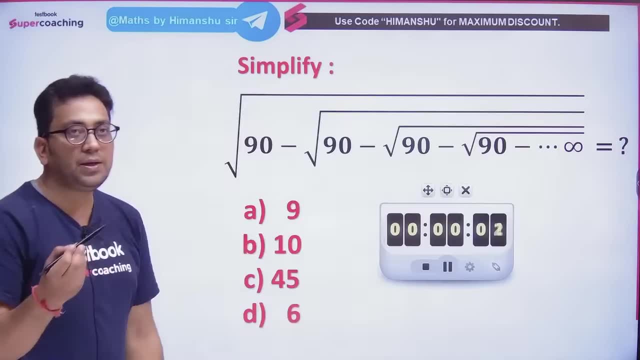 All the children who are answering B. yes, their answer is absolutely correct. 8 is the right answer. Great Next question: Ask quickly. Tell me what will be the answer. That is, you have to pick up the bigger one, You have to pick up the smaller one. 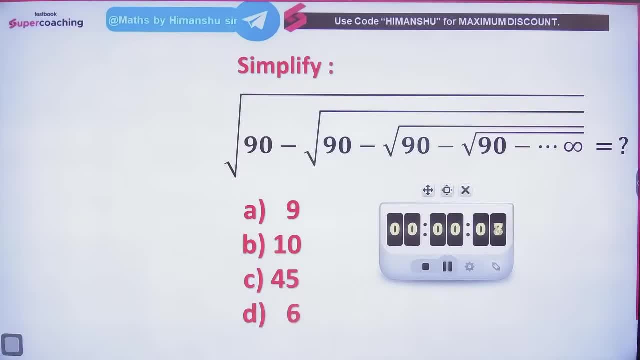 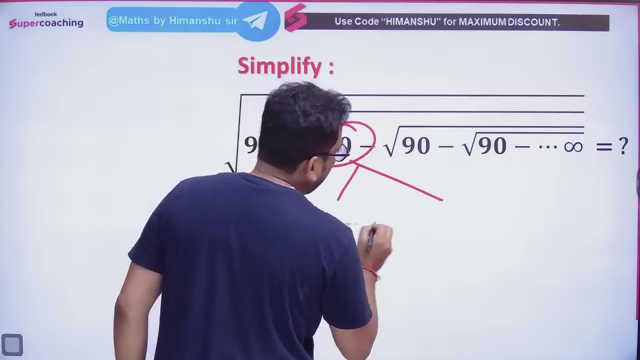 Tell me quickly. Answer with speed. Look my dear, Understand this carefully. Read it. He is saying 90.. We will break 90 in such two multiples in which the difference between them is: 1. Say yes or no. That is 9 times 2 is 90.. That is 9 times 10 is 90.. 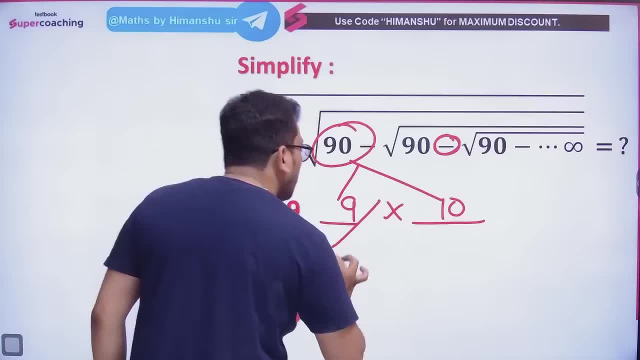 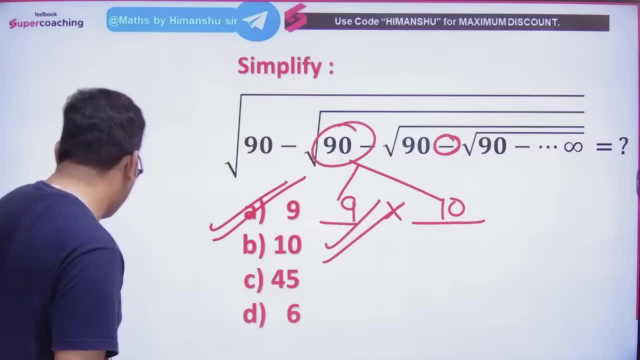 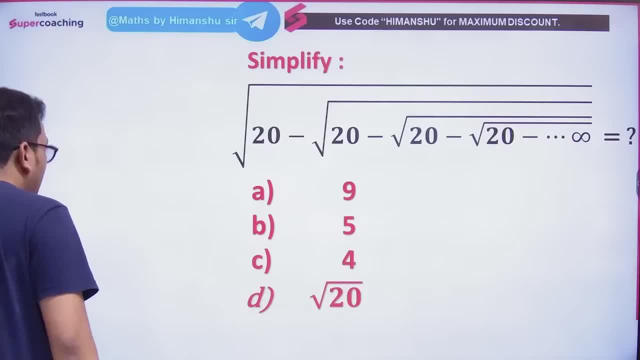 Is the answer coming? Is it coming or not? Yes, it is coming. Next question: Tell me quickly what will be the answer. You have given 20 this time. Answer quickly, all of you. Don't say entry in front of 9,, my dear Okay. 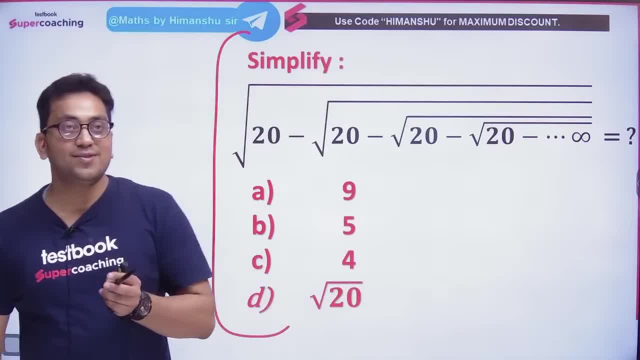 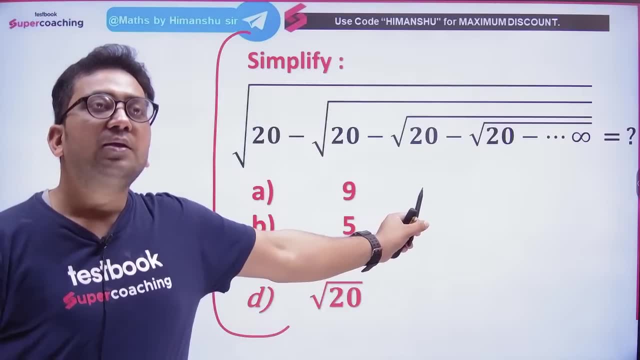 Because I have to enter the concept. I have to enter the concept, So don't say no entry, Just say no. All of you are getting a no Answer. this, my dear, All of you. Okay, Yes, What is a child saying? A child is saying something, sir. 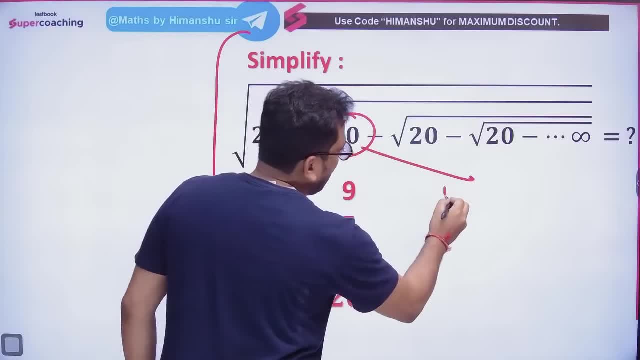 The comment is going: Look, son, there are 20.. You will say 4,, 5,, 20.. Yes or no? There is one difference between them. And if there is a minus, then who will we pick up? The small one? 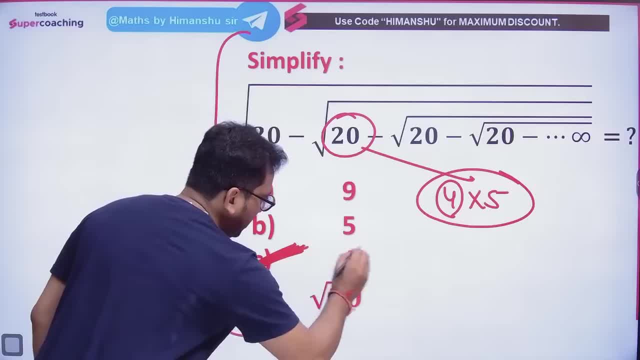 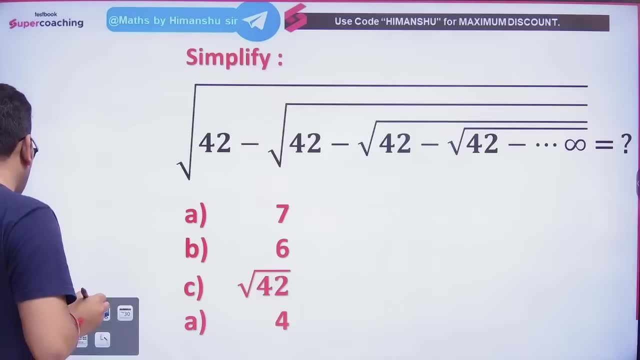 All of you are setting the boundary. Are you setting the boundary or not? Is it looking like a square or not? It is looking, sir. It is looking. Option number C is coming. It is looking Very good. It is looking like a tick on C. The next question is coming. 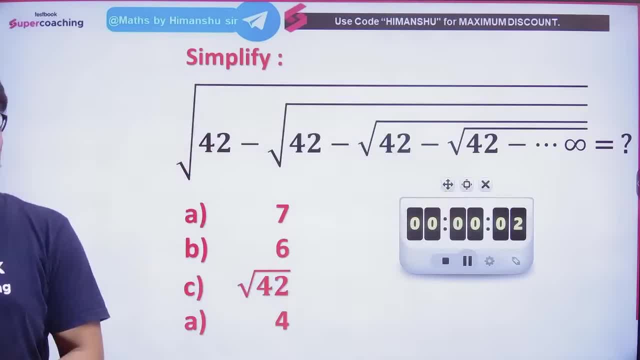 The next question is coming. Shine quickly, Tell me what will be the answer. Come on, brother, 42 has come. Thanks, god. Answer with beat all of you. Come on, brother, It is time here. crackdown of yours 42. what our dear. 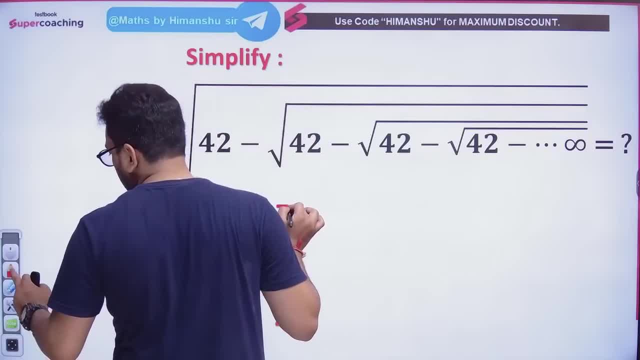 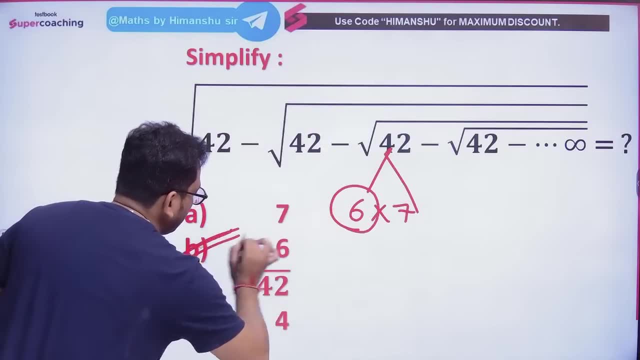 S742.. What is the s742?? S742?. Okay, If the answer is minus, then we will take a break. I put sixer. Sir, sixer is very good. Everyone put sixer. B answered Very good. 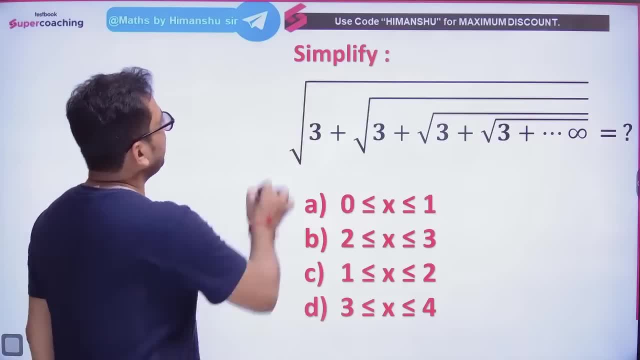 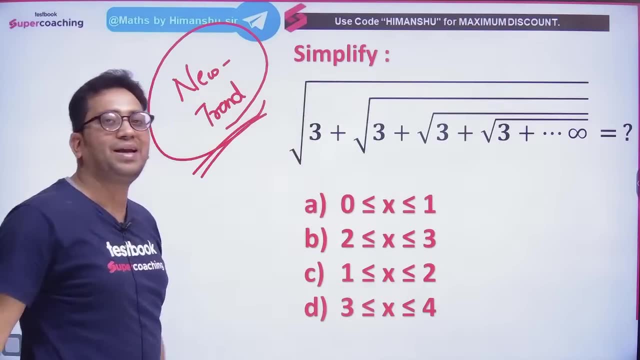 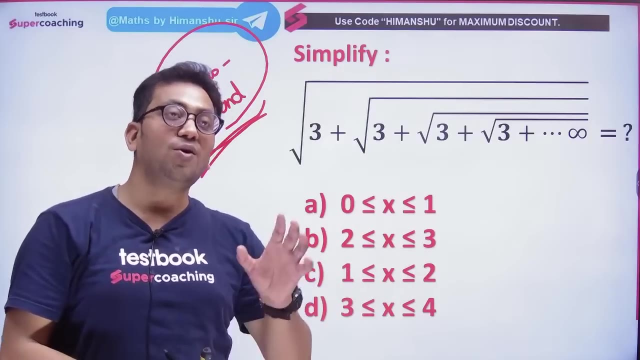 Now you will say: Sir, such questions are coming, Sir, this is a new trend. This is a new trend, Is it not? There are not only new ways, but also good and new questions are being asked to you, away from old and old questions. 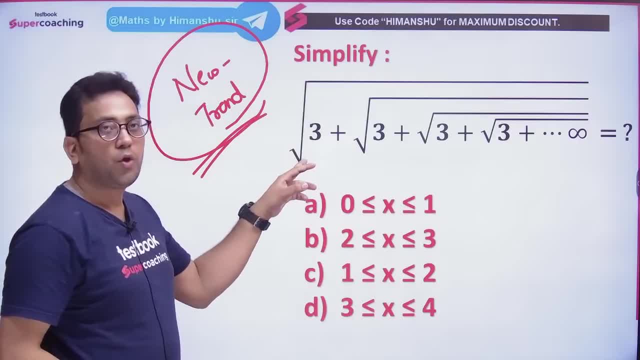 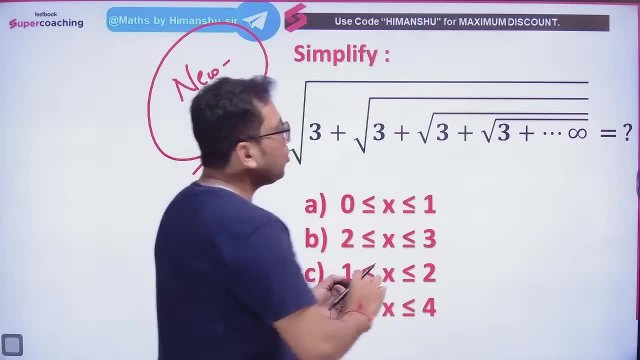 Now come here, son, This question, And in this question he is not asking you the answer. He is asking that if we solve it, then this X will come, It will be equal to X, And what will be the range of that X? 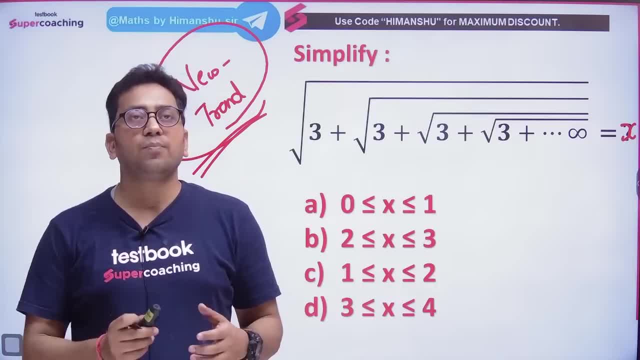 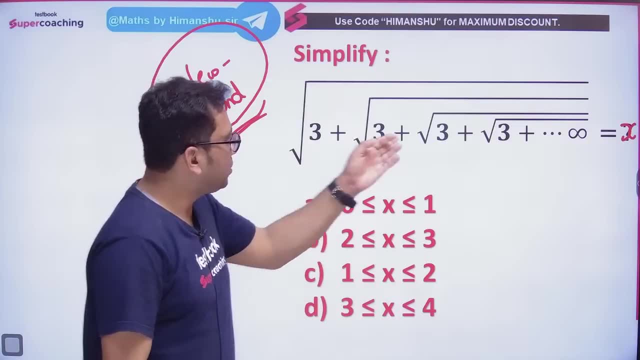 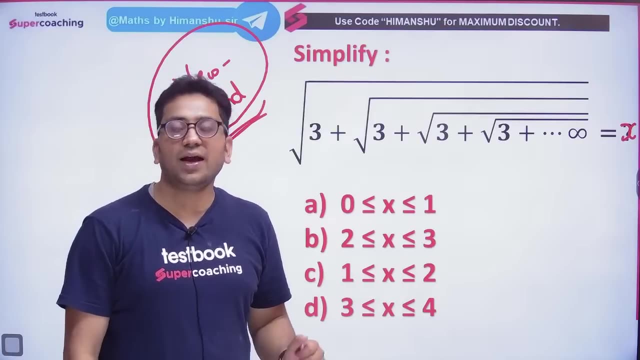 That is, in which two numbers will it come in between? What will be that range? What will be that ratio? He will ask you this: How to answer such questions, Sir? we cannot break these three. Can we break it? We cannot break it. 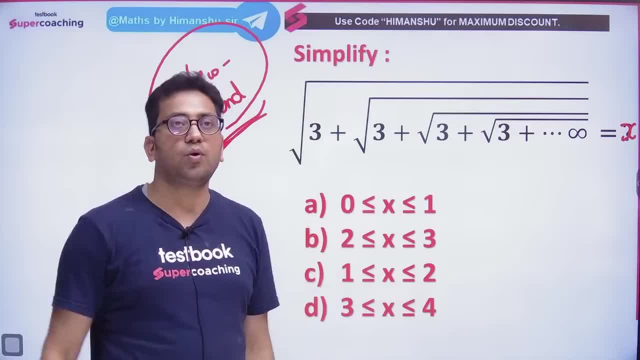 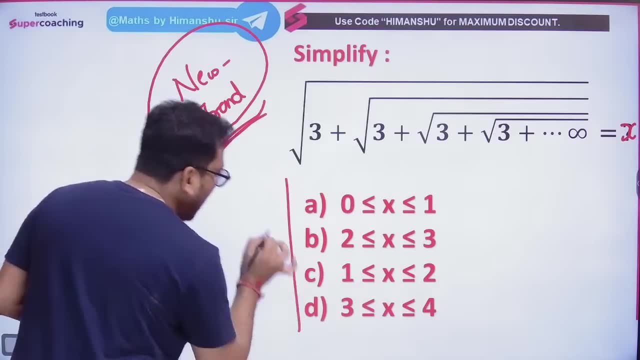 What will we do then, sir? What will we do? Let me explain to you- Come, sir, What you have to do. I will tell you how to do it. Then I will also tell you how to do it very quickly. 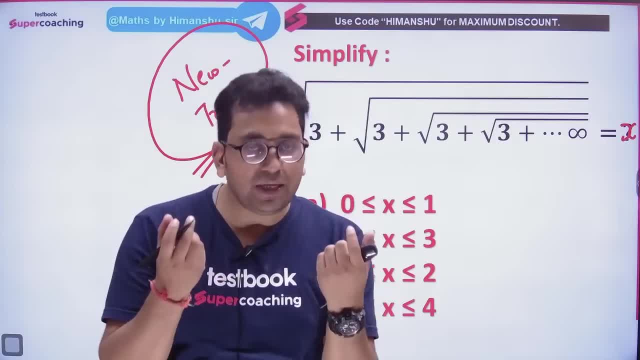 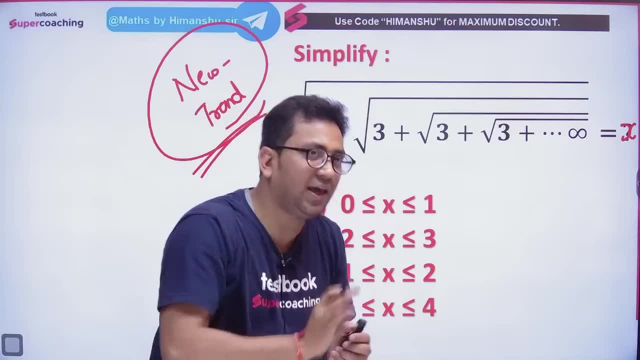 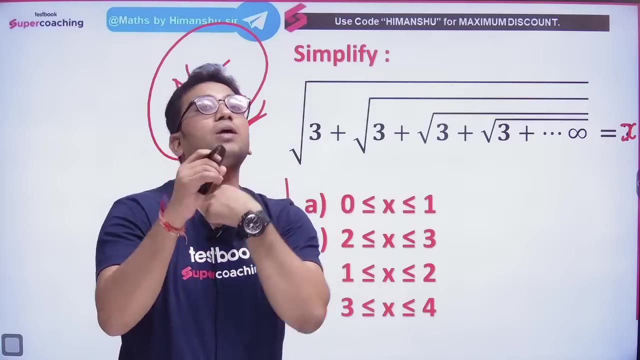 What you have to do. You have to see that three. If you are not able to break three in such two numbers, then you go ahead of three And ask him: do you have such two numbers whose range is equal to one, That is, can you break it? 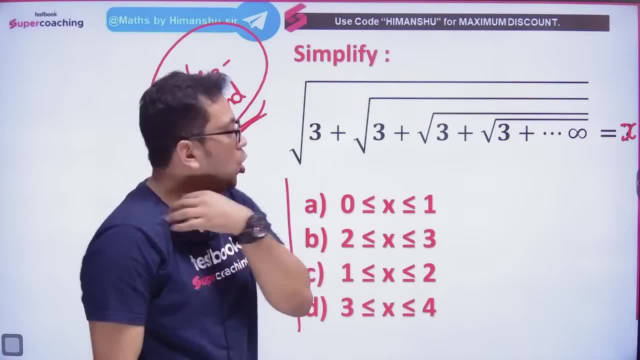 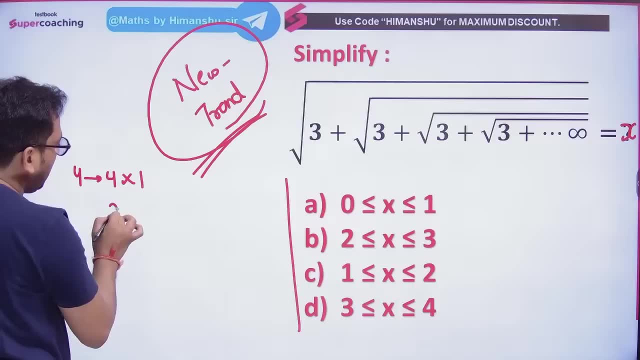 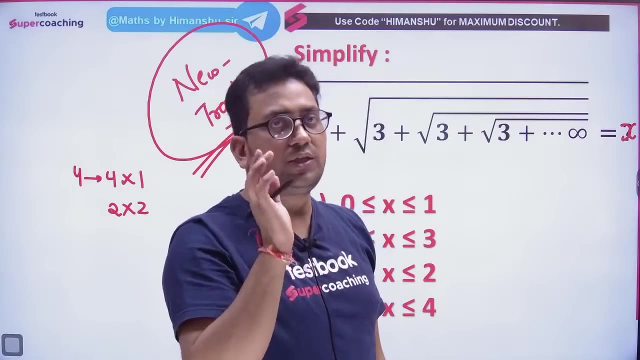 in such two numbers whose range is equal to one. So what comes after three? Four comes. If we talk about four, then we can say: four is four times one or two times four. So here the range is not one. What should happen? 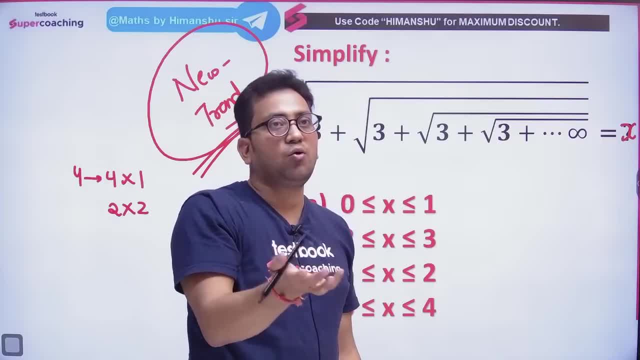 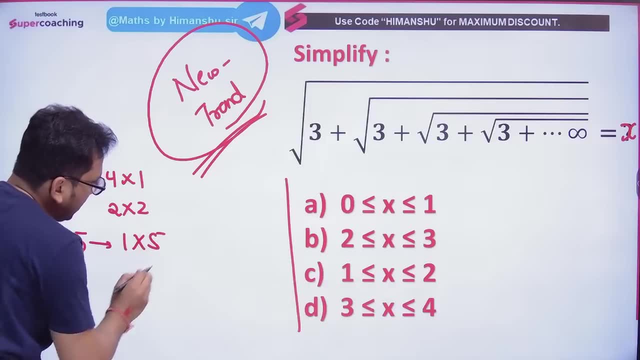 The range should be one. You will knock on the door of the number five. You will knock on the door of the number five. You will say five. Will you say five? Can we break three? He will say: you can break me. 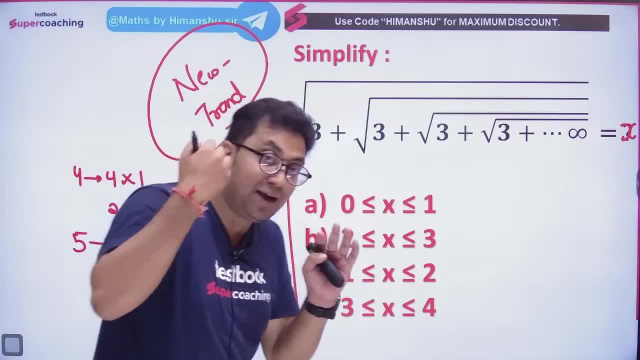 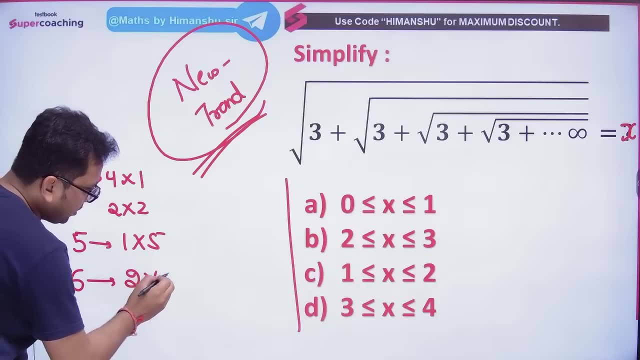 just one times five. That is, even I will not get an interval of one, So you will knock on the door of the next number of five. What is that Six? Then you picked up six And you will ask: six, can we break three? 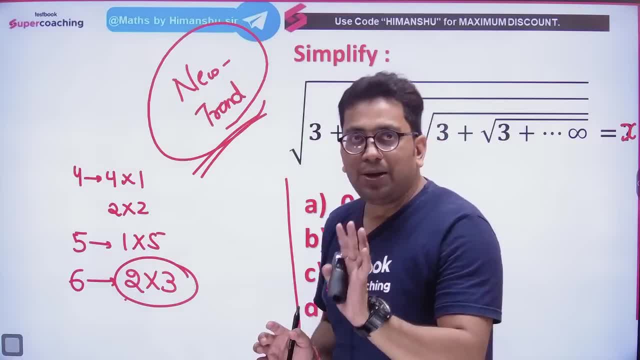 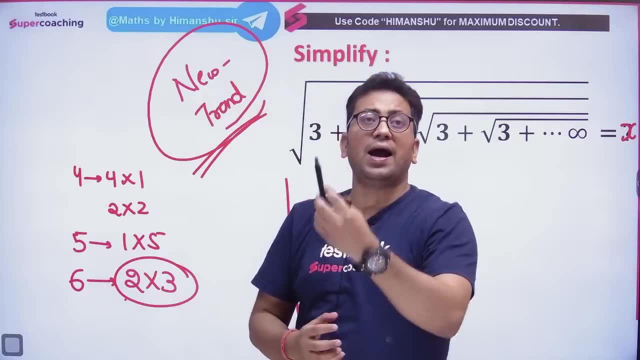 He will say: you can break it at all: Two, three, six where the difference is one. You have picked up six where the difference is one. That is, you have to go ahead of three. You have to go ahead of the number written. 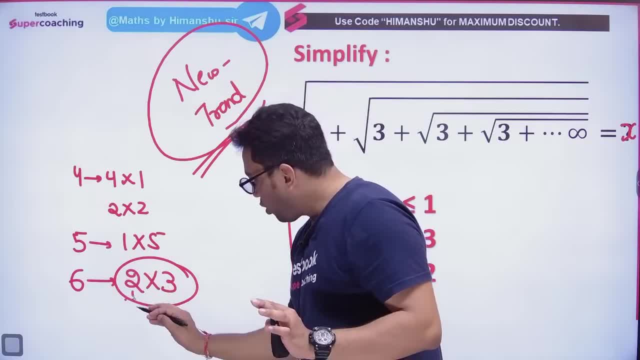 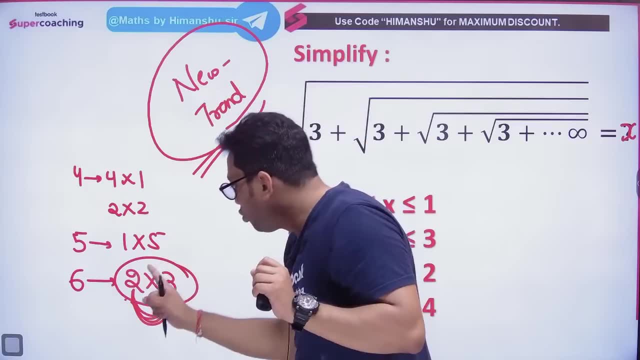 So you saw two, three, six, That is, we are getting six, So the two that have been broken into multiple. the value of this x will come in between these two numbers, In which In two and three. That is the answer that will be made. 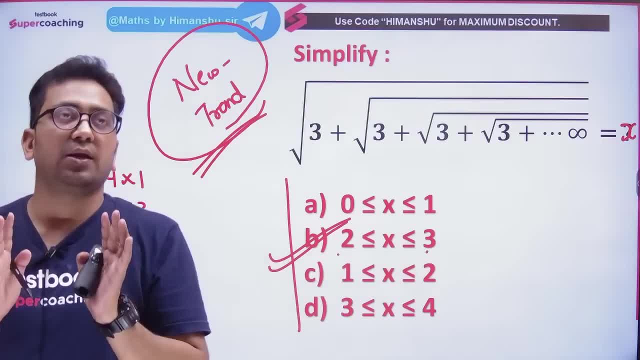 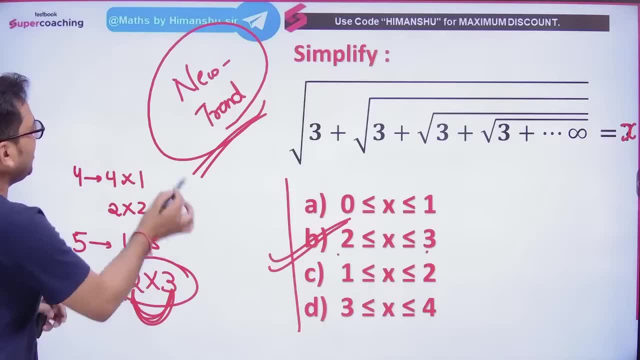 will be the alternative b, Two and three. Do you understand what I am saying? Okay, Now I will tell you how to shine. You will say, sir, if I start thinking like this, if I start wandering like this, if I start knocking on everyone's door, 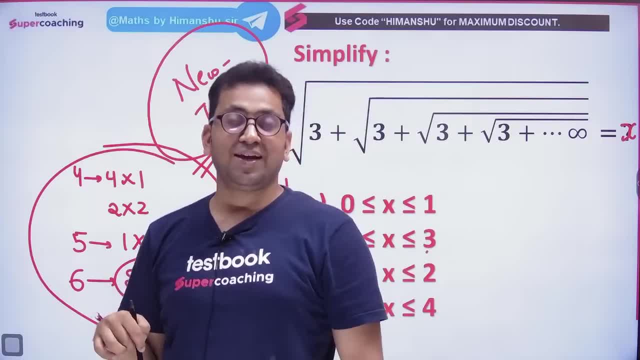 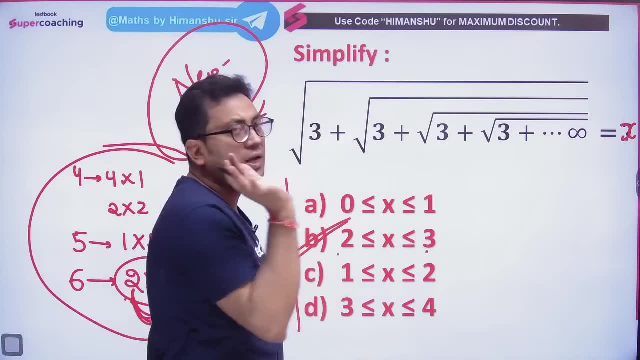 then, sir, if someone kicks me out, then what will we do? And, sir, there is not so much time. we are knocking on everyone's door. Sir, tell me some such way that I look at the question and tick the answer. 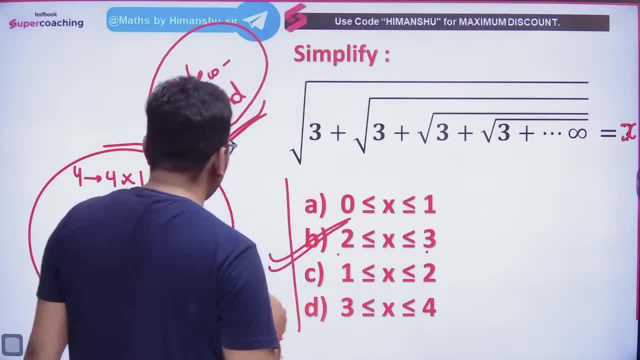 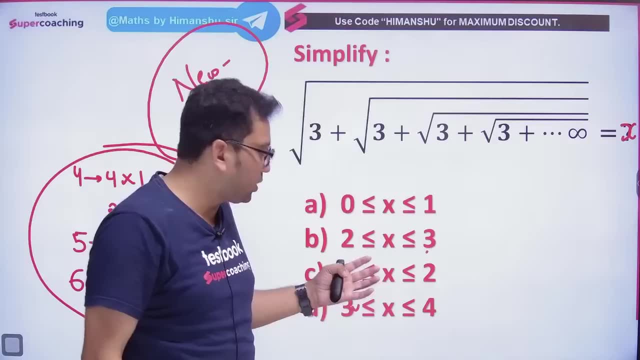 Tell me this way, sir. It will be fun. So understand this way. What will you have to do, son? Why are options given to you, Brother? that's why they are given. Use them. What to do? I will explain to you. 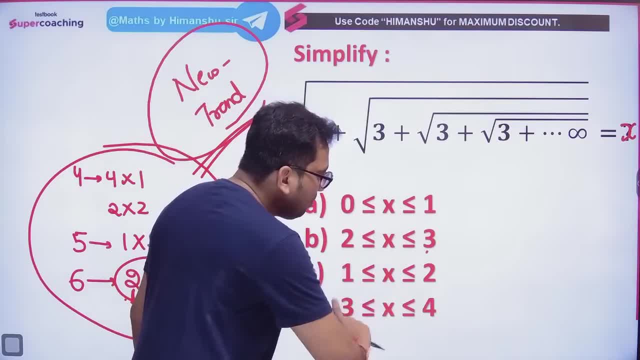 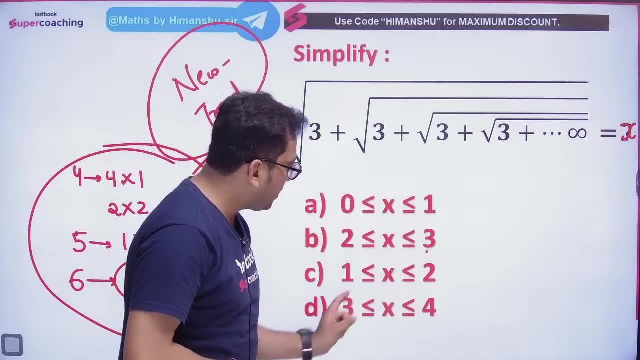 First of all, you have to see that the difference between the two numbers given should be one. You have to choose that option first. So you saw, yes, the difference between one, the difference between one, the difference between one is very good. 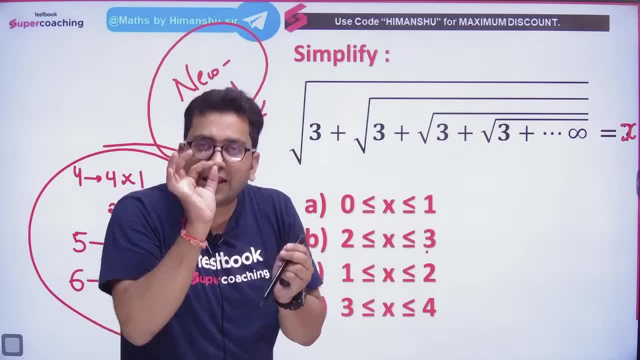 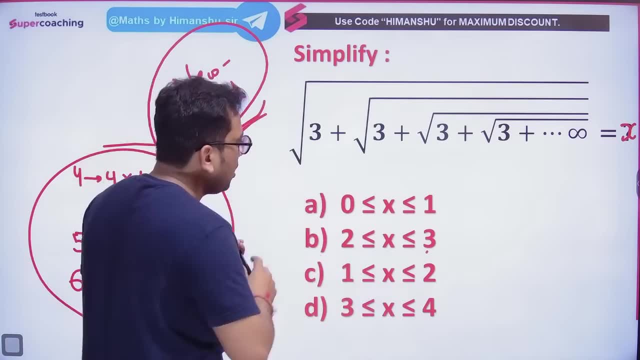 Now you do their calculation and calculate that it should be bigger than three. but it should be just big. The number that is bigger than three will be your answer. For example, if 0 is multiplied by 1, then 0 will come. 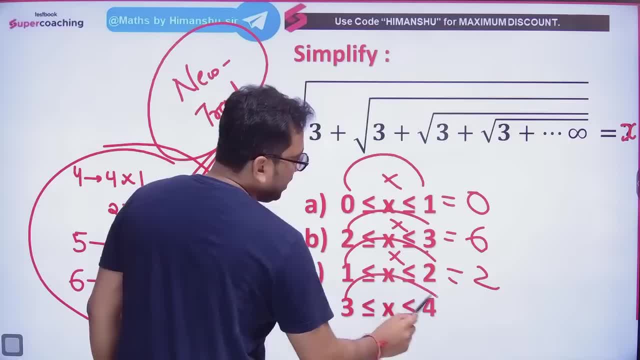 If 2 is multiplied by 3, then 6 will come. If 1 is multiplied by 2, then 2 will come. If 3 is multiplied by 4, then 12 will come. Tell me, do you understand so much? 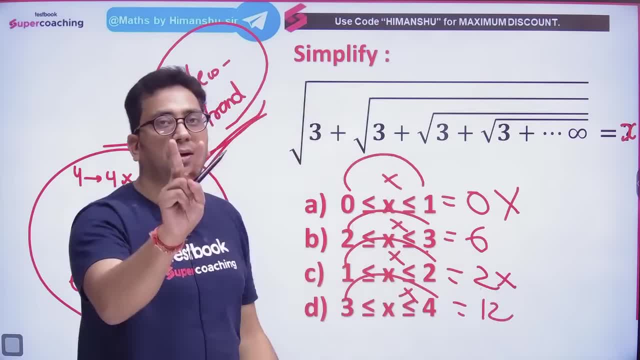 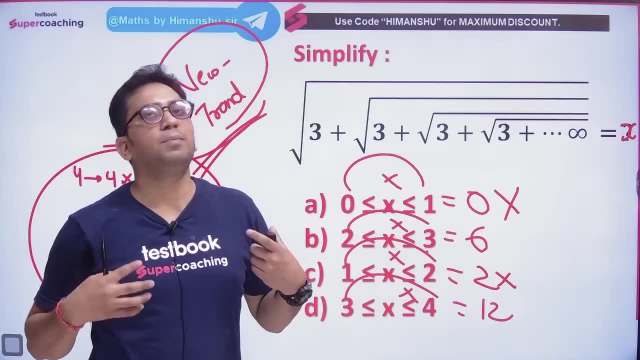 Now I want to see big. So, sir, it will not be 0,, it will not be 2.. I am getting two big numbers, 6 and 12.. But who got 6 first, Brother, what we wanted, we got it first. 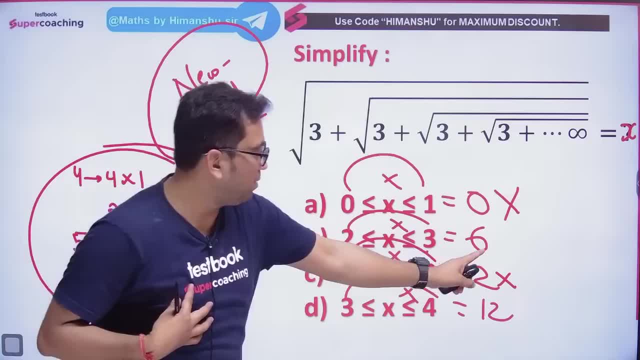 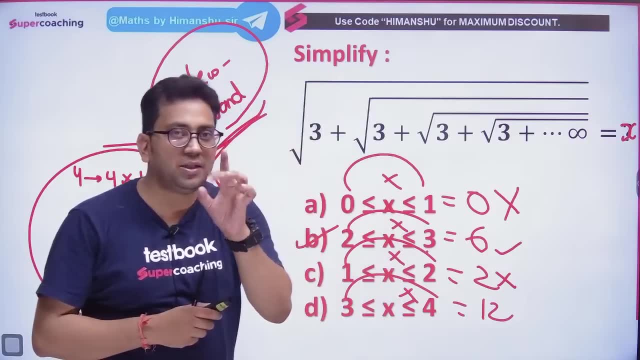 So why will we go to the next door, Isn't it? So 6 is our answer. Means this will be our answer. now You have to do this. You have to see the difference Where the difference is 1, you have to choose them first. 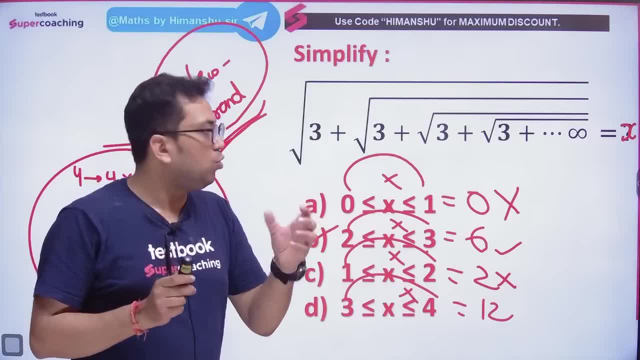 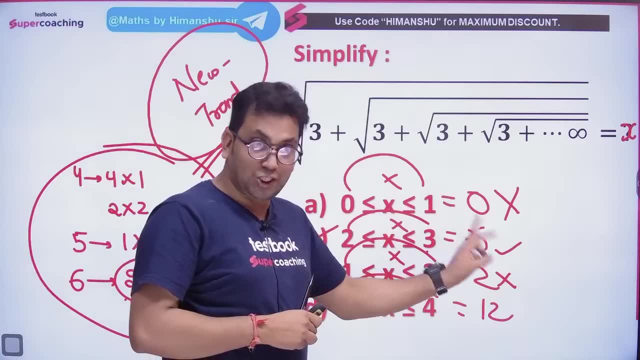 Where the difference is not 1, remove them first And then do the calculation and see that the number should be just bigger than this Means it should be big, but get it first. Now it is 12 or 6, but if you get 6 first, 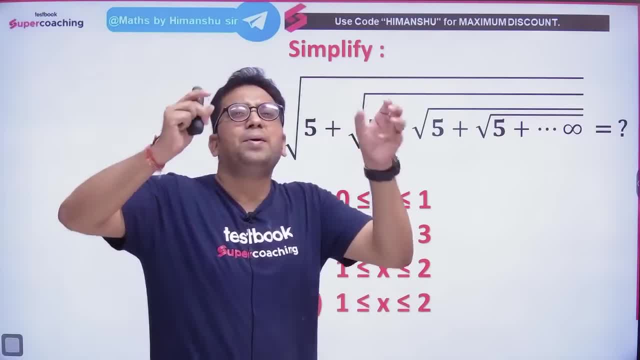 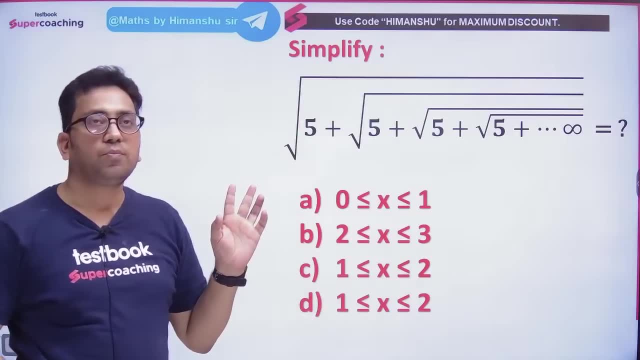 then this will be your answer. Now see, the next question is coming in front of you. You see, without thinking anything, you will get the answer. This is my guarantee. Tell me quickly what will be the answer. Look at this question carefully. 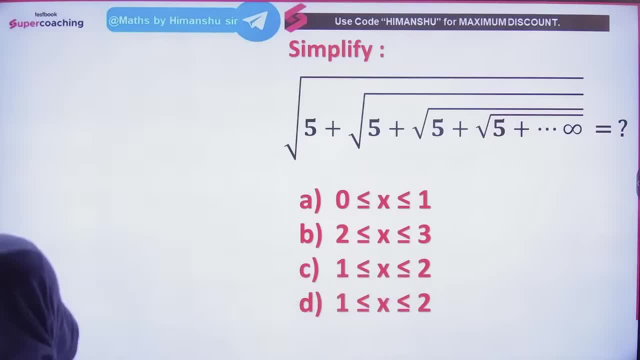 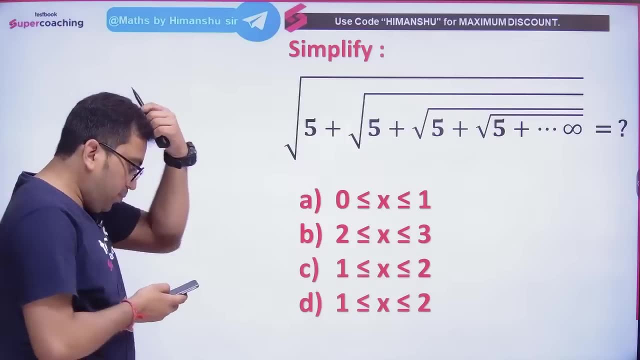 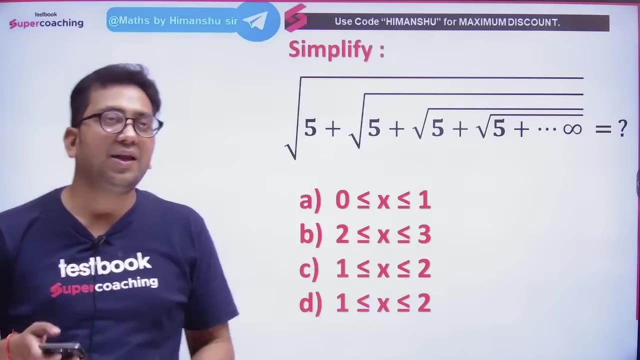 and guess the answer. Tell me quickly, Answer with speed. Ok, brother, I am able to see here. You people like all of them. There are only 749 likes here. Ok, I would like every child to, if you are having fun. 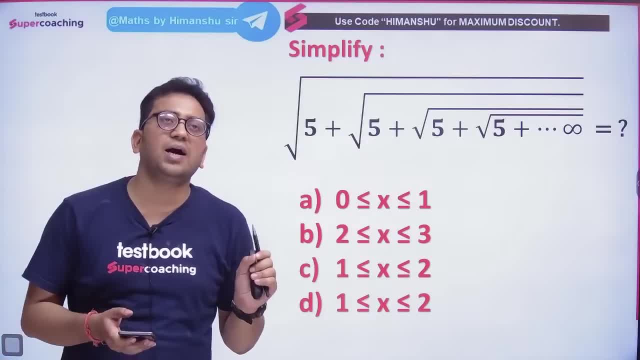 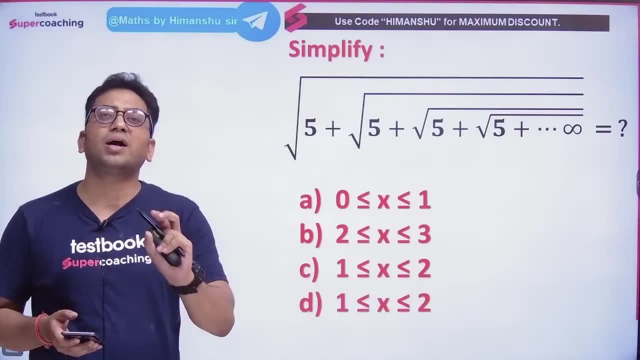 then all of you children click on it quickly. If you are having fun, then I am giving you such great things. I am saying with guarantee, I will write it on the pen and paper. You will not find such great things anywhere, Only and only at 12 o'clock. 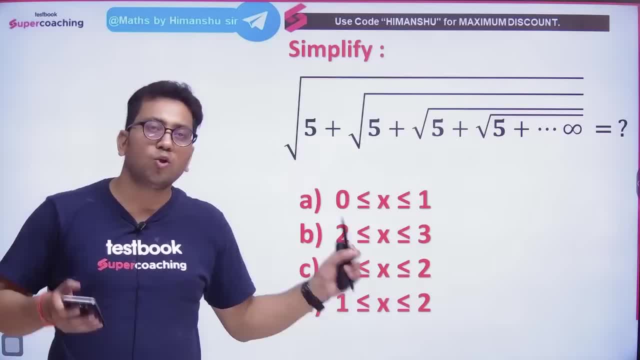 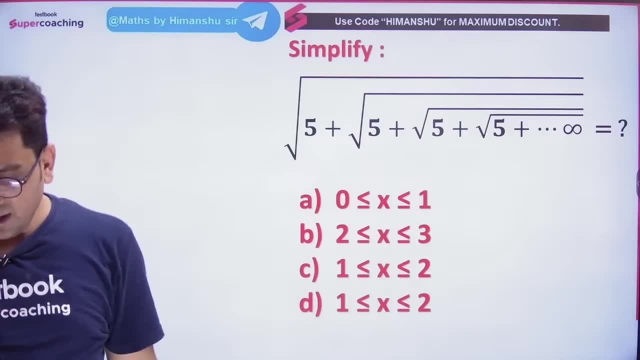 you will get the classes of Himanshu. sir, I am doing a lot of hard work to give you all these things, So a little is needed. I am not asking anything from you. Click on the like button. Who has clicked on the like button? 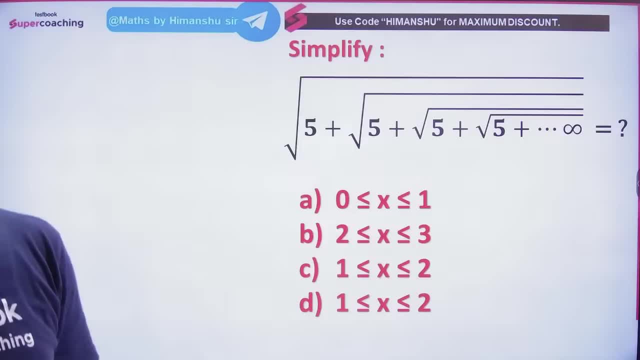 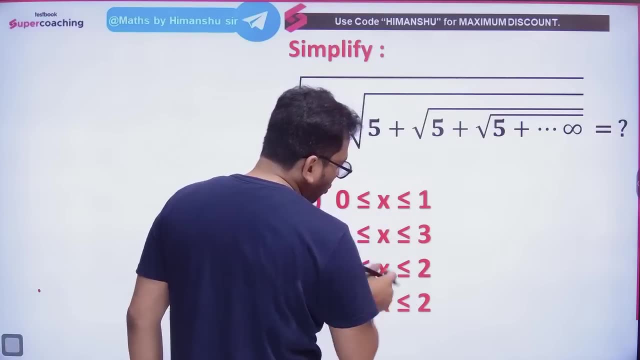 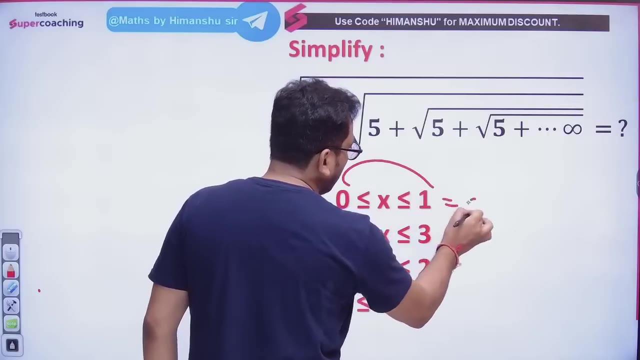 Quickly Come down. What will our child do? He will see the difference. Both the options are the same. The difference is the same. Now our child will do the multiplication. When he will do the multiplication, then it will be equal to 1 of 0.. 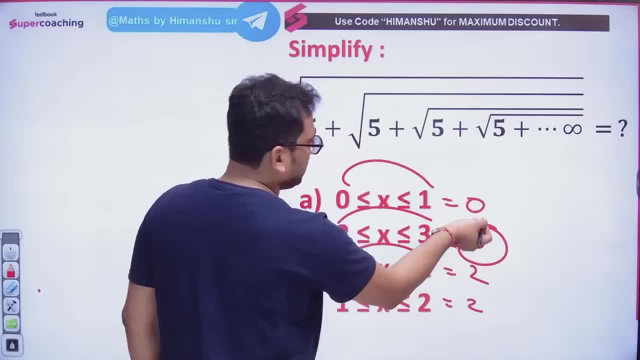 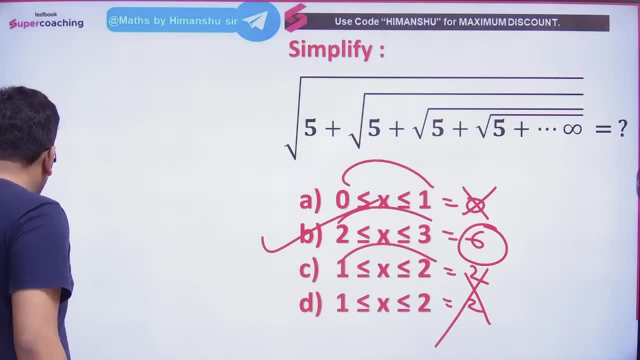 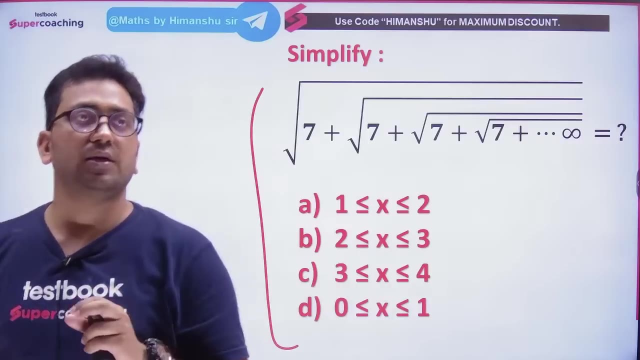 How much is 2?? 6. 2 is less than 2.. This is also 2.. Sir, we have got 6.. Ok, Do you understand? It is fun. Next question: Let's see how many children are able to answer. 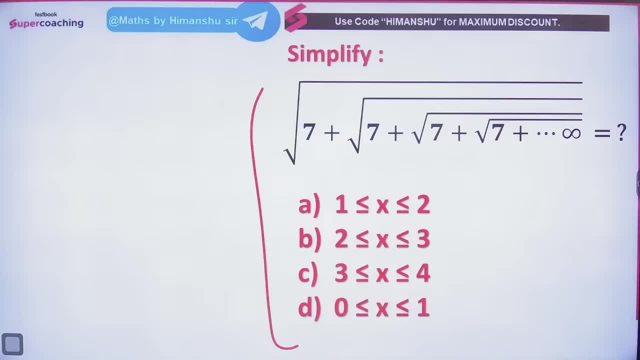 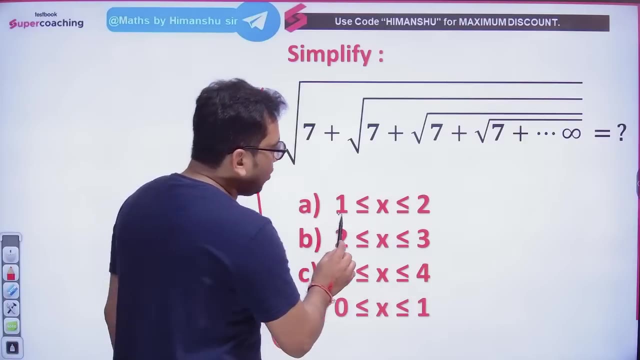 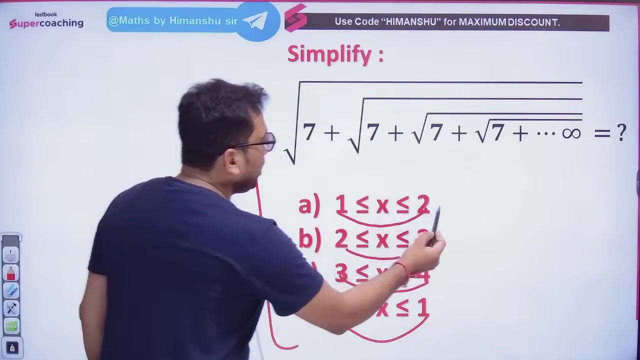 Let's see how many children are answering, Answer with speed, All of you. Let's see What are you seeing? There should be a difference. There should be a difference. There is a difference everywhere. Now we will do the multiplication. 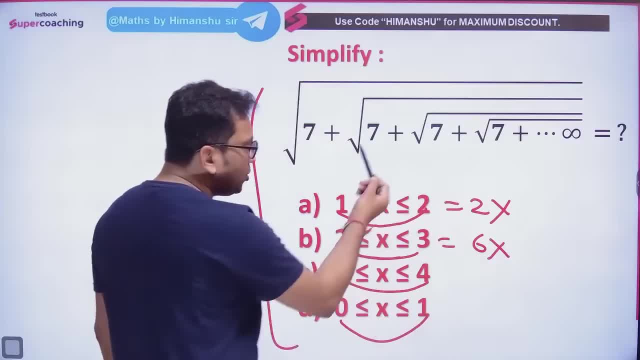 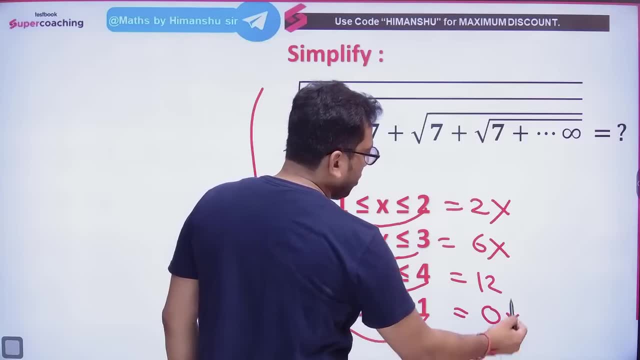 2 is less than 2.. There will be no answer. Why not? 7 is small. 7 should be bigger than 7.. 3 quarter is 12.. We will do the multiplication of 0 with 1.. There will be no difference. 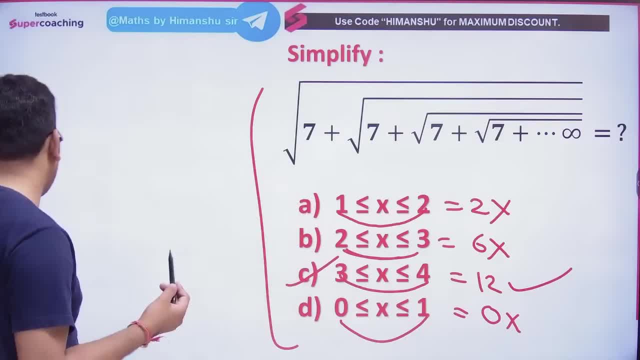 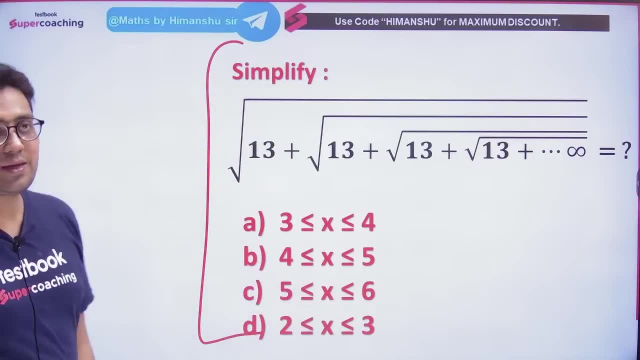 Only one option is visible And this will be our answer. C is our answer. Next question. Next question is in front of you And you will not answer it now. You will answer it in the comments section. Where will you answer it? 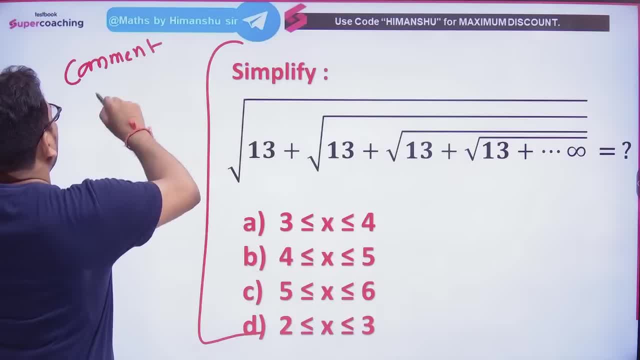 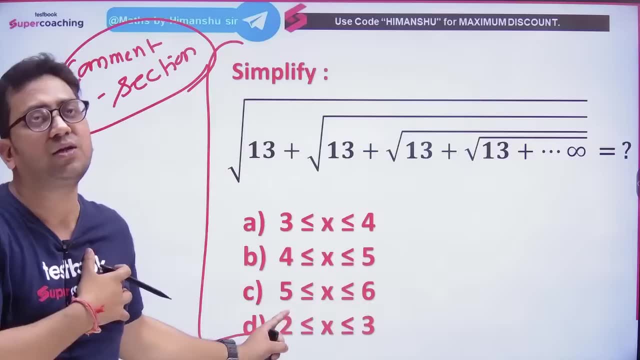 All of you will answer it in the comments section. All of you, And I would like to That whoever is watching this session Keep your hand on your heart and say and promise that all of you will answer it in the comments section. All of you. 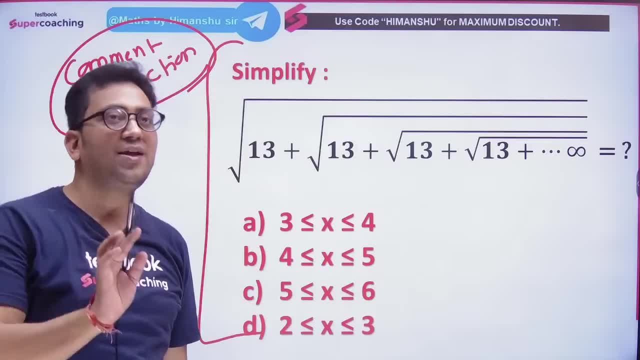 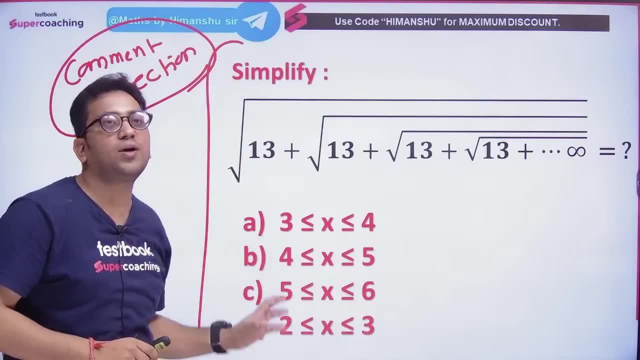 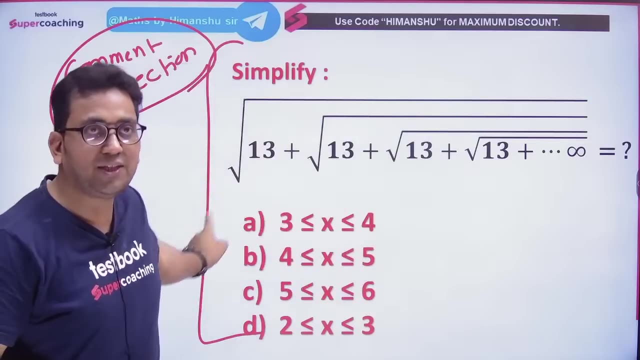 I want the answer in the comments section of every child. There should be no difference. After the video is over, in the comment section below, every child has to answer it And you have to write together. I love my Bihar. Once all the children will write in the comment section. 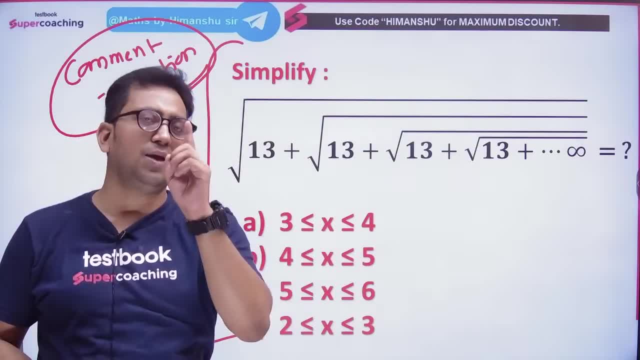 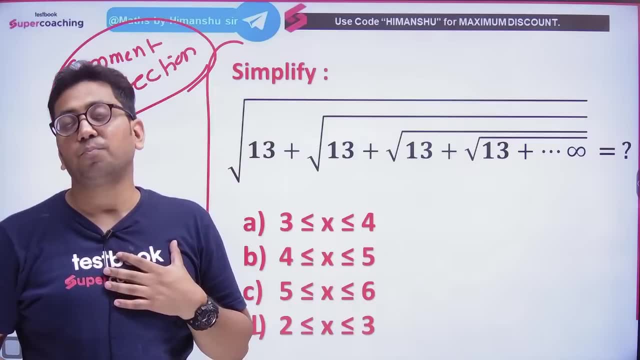 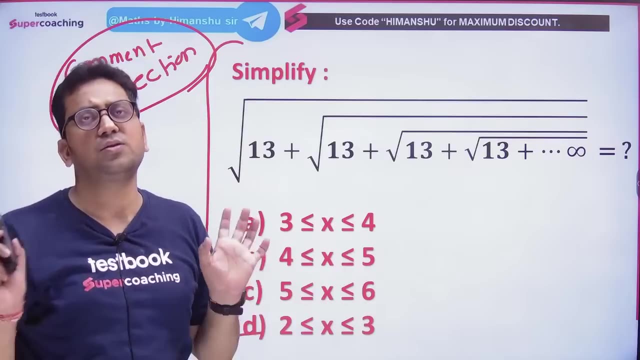 After the answer is done, after the video is over, every child will write answer and then I love my Bihar, Do try. I don't say this should be right, But I have so much pride in myself and I have so much faith that you will all answer this correctly. 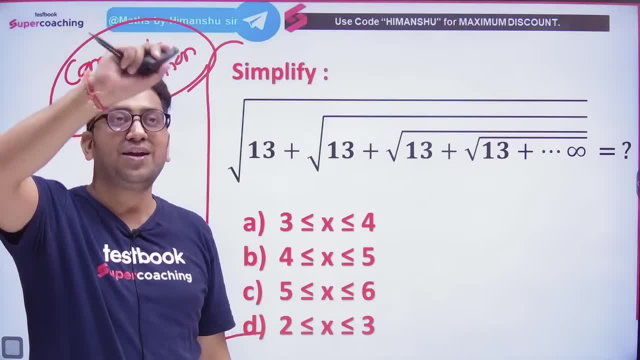 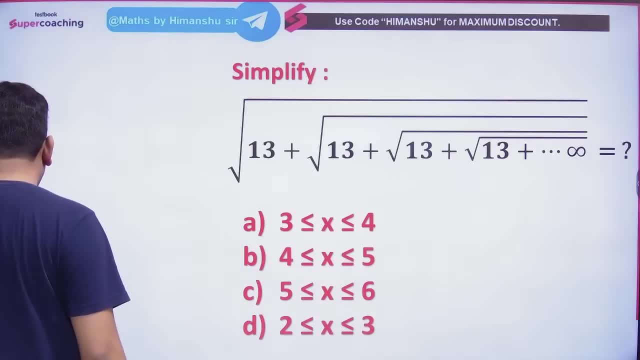 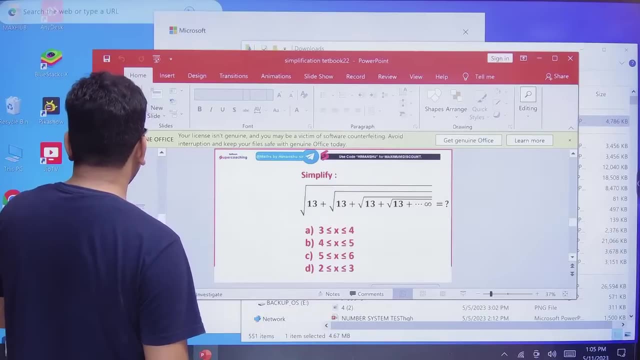 Because you have got this concept in your mind, Isn't it Very good? Okay, now I will give you some more information. First of all, the child who is not yet connected to this telegram channel: Maths by Himanshu sir is a telegram channel. 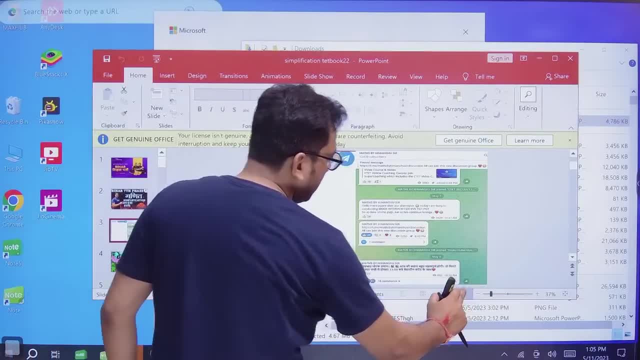 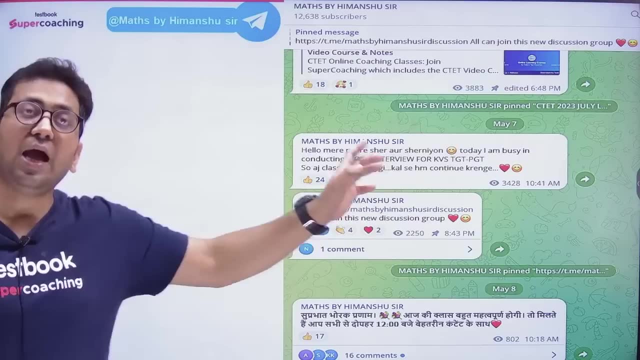 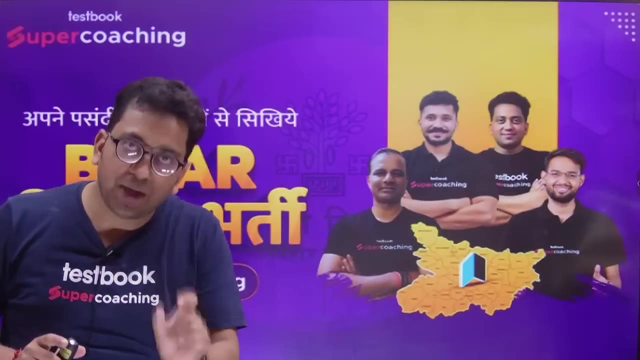 All of you children should connect to this telegram channel. Maths by Himanshu sir is a telegram channel. The child who is not yet connected, the child who is deprived, should not be deprived. All things will be provided here. Okay, And along with that, the paid batch of Bihar Shiksak Bharti is also available on your Super Coaching. 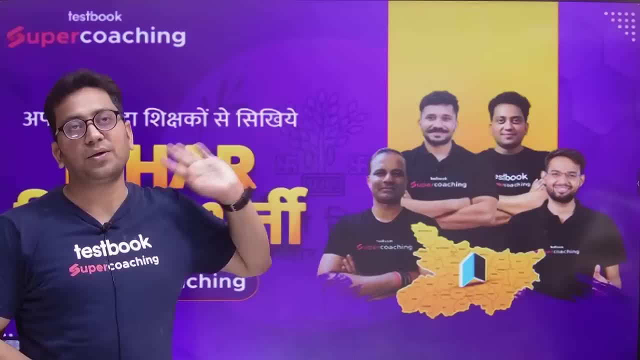 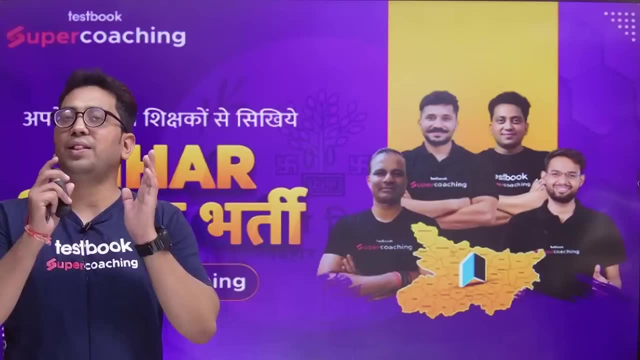 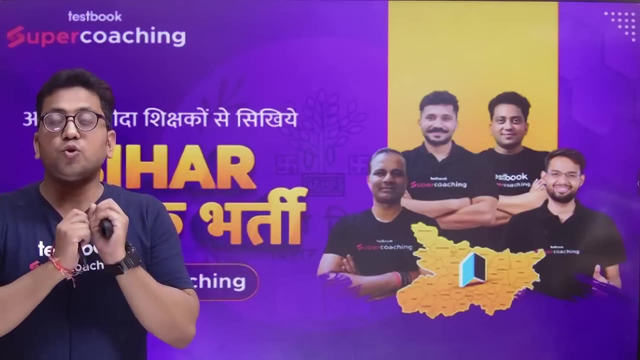 You can enroll. it will be with you till the exam date. Okay, As soon as the notification comes, you will get all the teachers teaching you live. Okay, And now I will explain the video for you. The video has been provided so that you can utilize your precious time. 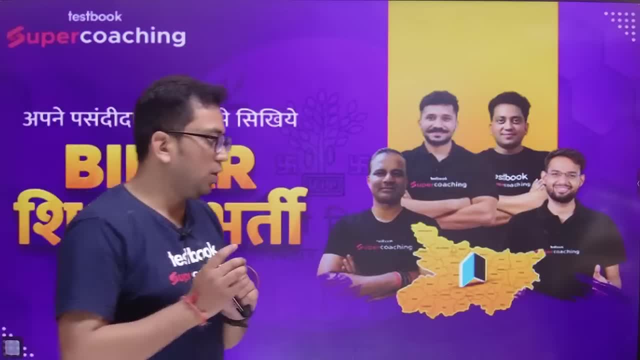 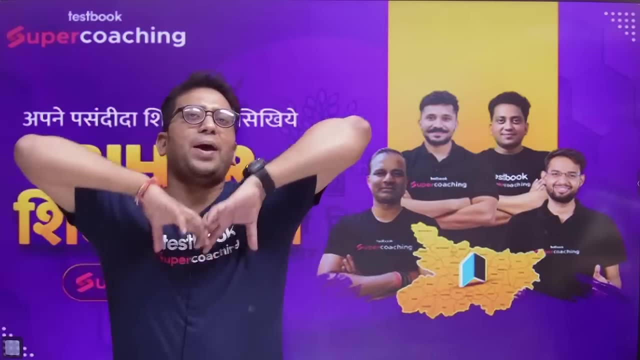 So you also have topic-wise videos available here, Okay, So let's meet you all Tomorrow. at exactly what time? At 12 o'clock, in this class, And with excellent, amazing questions. I will join. Every child has to come and join. 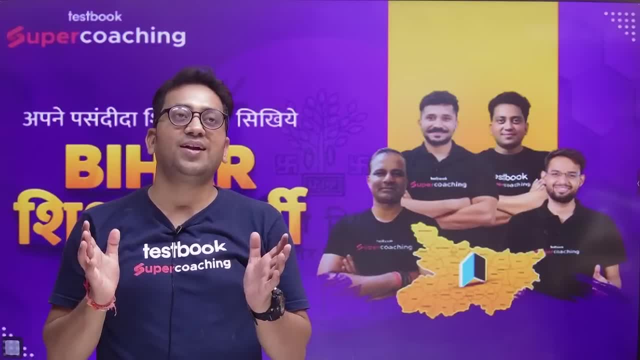 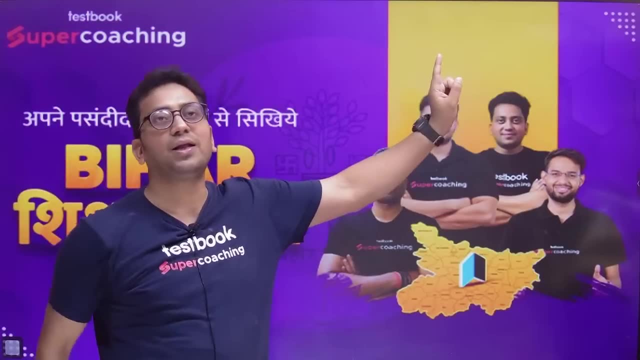 Tomorrow. at exactly what time? At exactly 12 o'clock. I am your Maths faculty. Who, Himanshu Gupta. All of you will write in the comment section Maths by Himanshu Gupta, So that every child who is not yet connected to this Telegram channel.